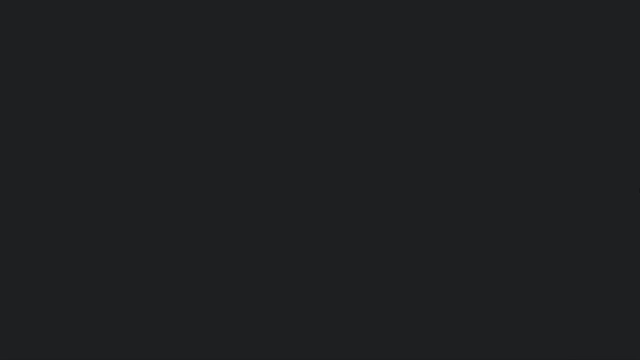 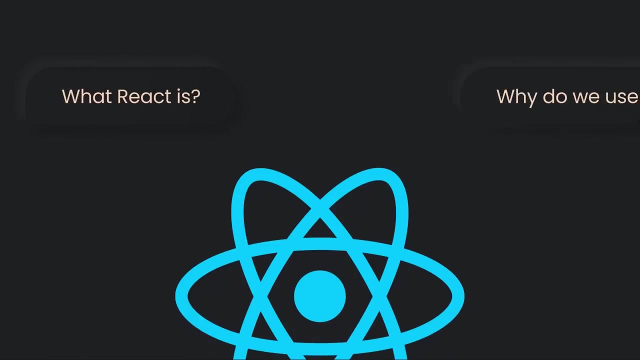 Hi there. If you want to learn everything from the essential JSX syntax all the way to more advanced React topics like state hooks, data fetching and more, you've come to the right place. I'll first give you a high-level overview of what React is and 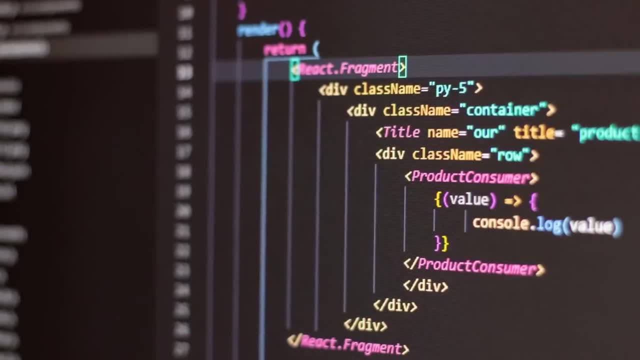 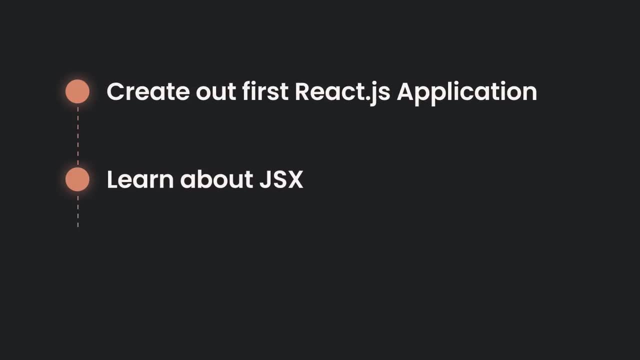 why do we even use it? And then we'll quickly dive into the code, create our first Reactjs application, learn about JSX, which forms the core Reactjs syntax, and learn about the best file and folder structure when working with React. Most importantly, in the end I'll teach you how you can build a Reactjs application. 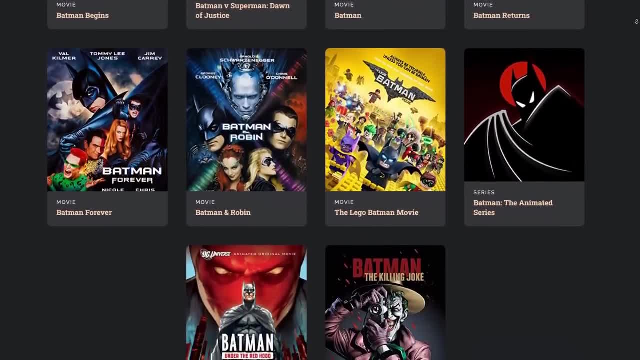 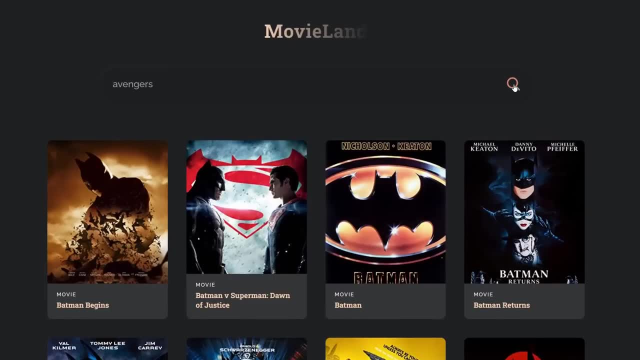 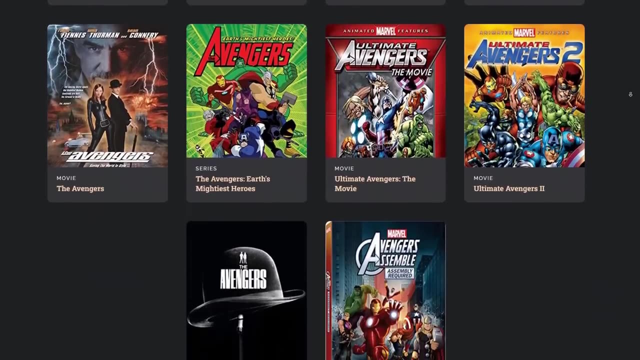 so that you can actively internalize and independently apply everything you've learned in this video. By the end, you'll know precisely what you need to do to become an outstanding React developer capable of building phenomenal applications. With your React skills, you'll also be able 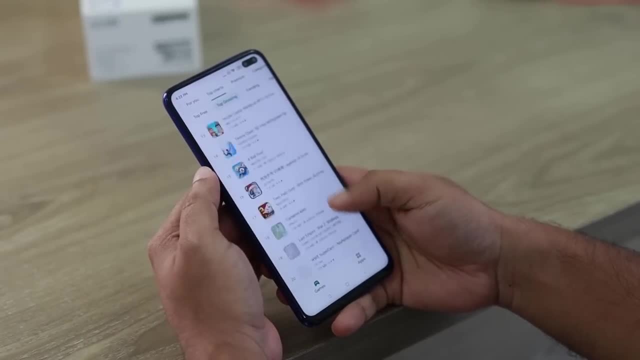 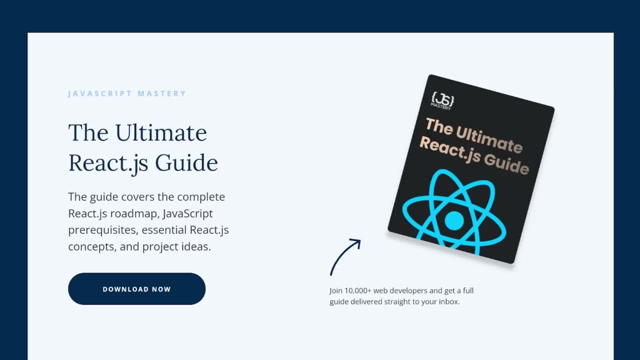 to build native mobile applications. Thanks for watching. The link to the guide is in the description. You can download the guide and use it if you want to learn more about Reactjs and other mobile applications. Isn't that crazy? Alongside this video, I've also prepared the Ultimate Reactjs Guide that covers everything. 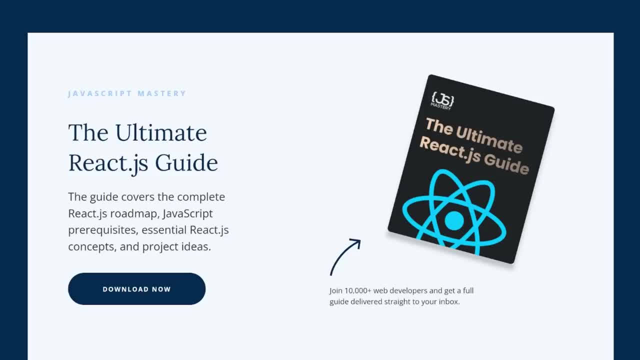 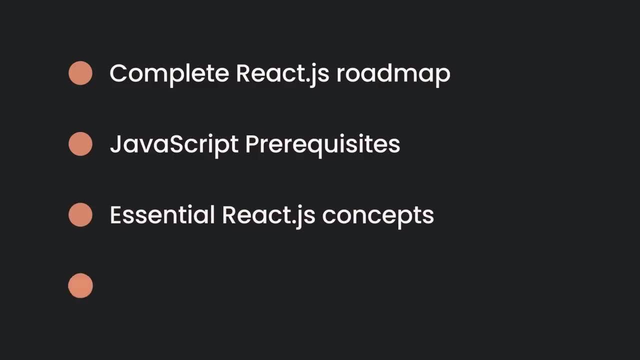 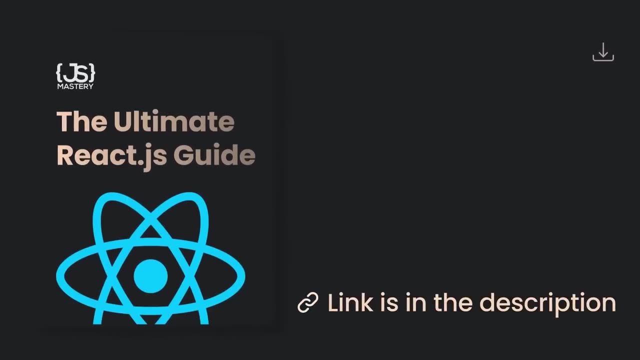 you need to know to become a fantastic developer. The guide covers the complete Reactjs roadmap, JavaScript prerequisites, essential Reactjs concepts and project ideas that you can build and deploy to put on your portfolio and get a job. You can download the guide and use it as a reference on your Reactjs journey whenever. 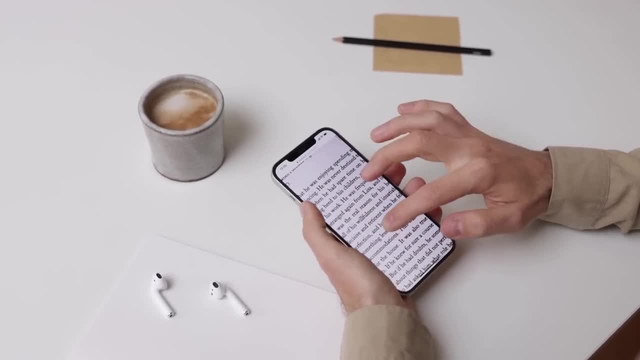 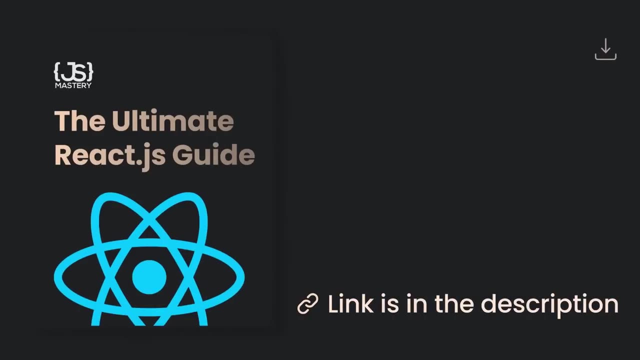 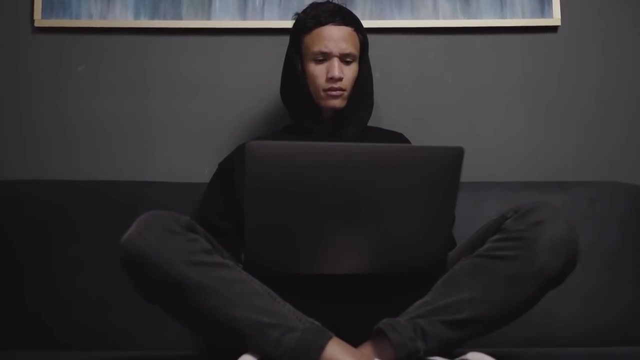 you're unsure what to learn next. Of course, the guide is completely free And, once again, the link is in the description. Still, I'd strongly recommend that you watch this video until the end, because, although the guide is great as a quick reference point, the video will provide you with absolutely. 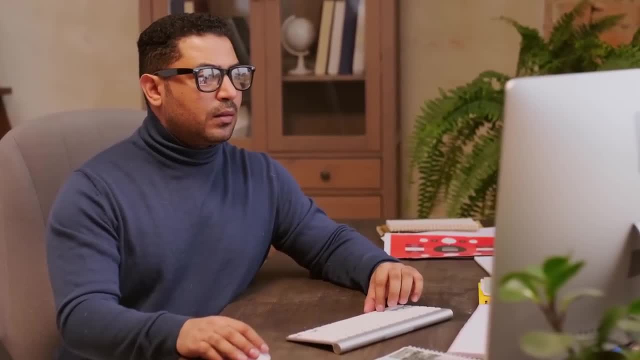 everything you need to become a professional React web developer And, of course, exclusively in this video, we're going to build a Reactjs application. So, until the end of this video, don't forget to subscribe to my channel and turn on the notification bell so that you 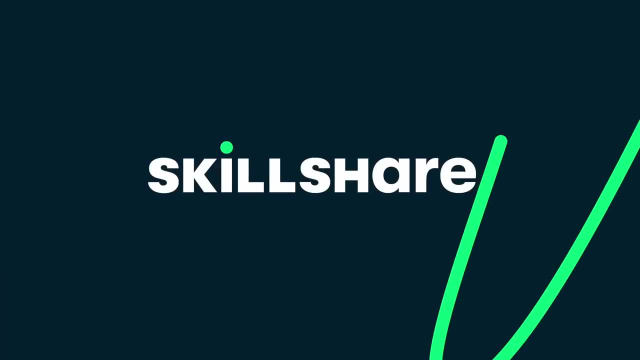 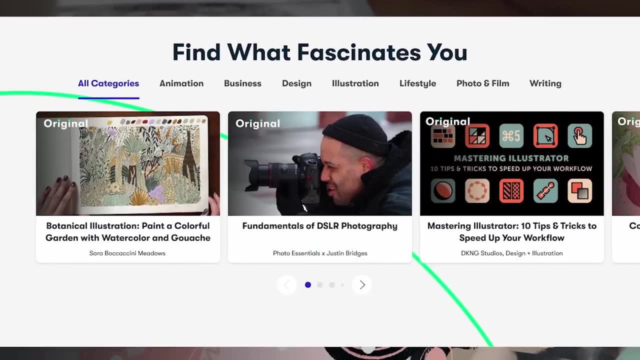 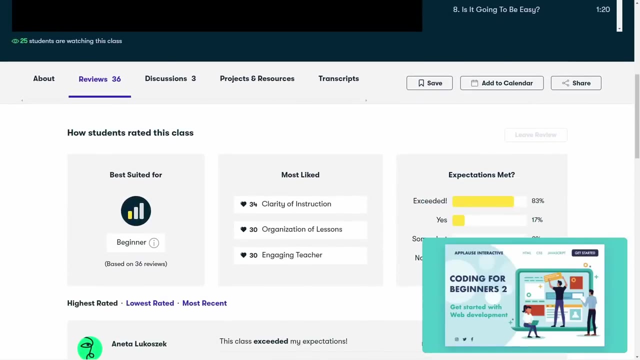 don't miss any of my new videos. This video is brought to you by Skillshare. Skillshare is an online learning community with thousands of inspiring classes for anyone who wants to learn new skills. As I was in the process of creating the Ultimate React developer roadmap, as you saw in the intro, 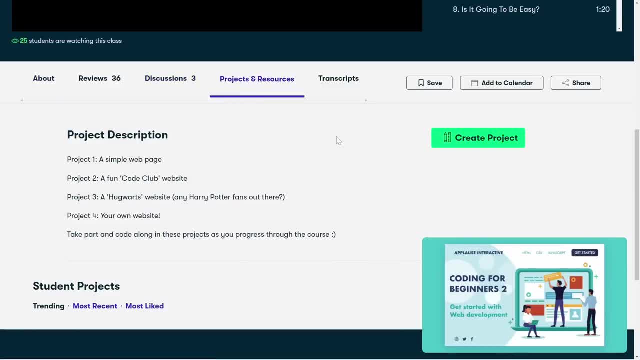 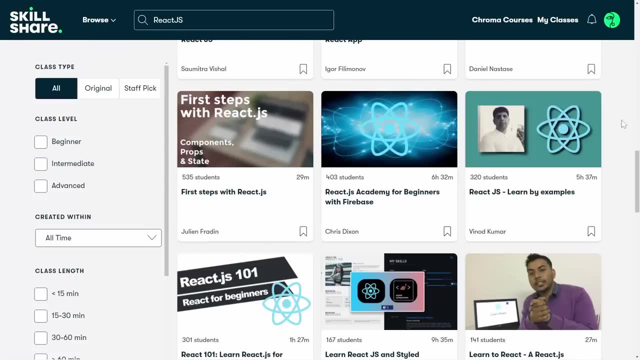 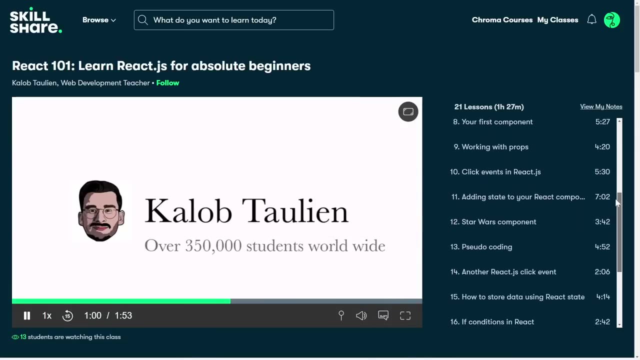 I needed to revisit everything from bare beginnings. That's why I browsed the courses in Skillshare and stumbled upon Reactjs. The tutorial was called React 101 – Learn Reactjs for Absolute Beginners by Caleb. If you're a beginner React developer, I'd strongly suggest you watch this video first. 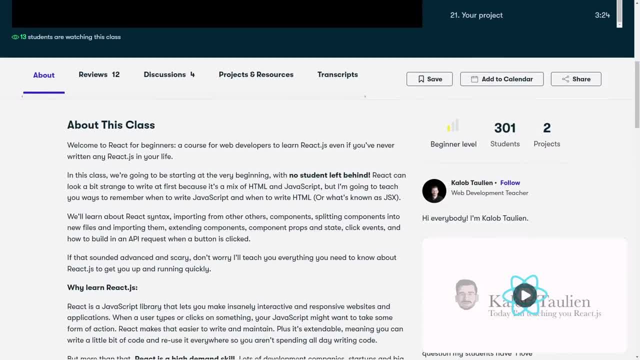 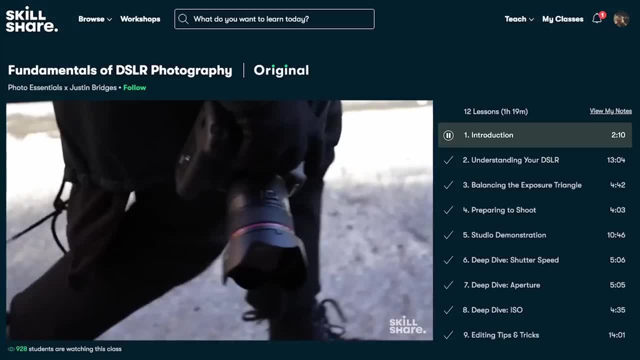 and then go check out this course on Skillshare to get as much knowledge as possible. If you're a more experienced developer, you'll love their more advanced courses. If you sign up right now, you can start learning for free with the unique free trial link in. 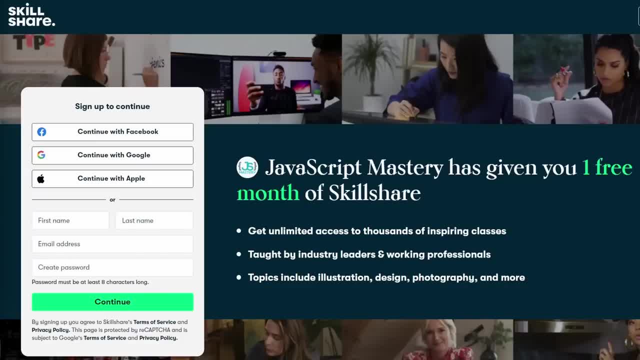 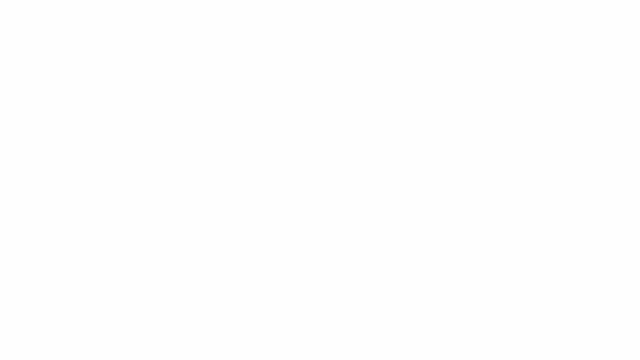 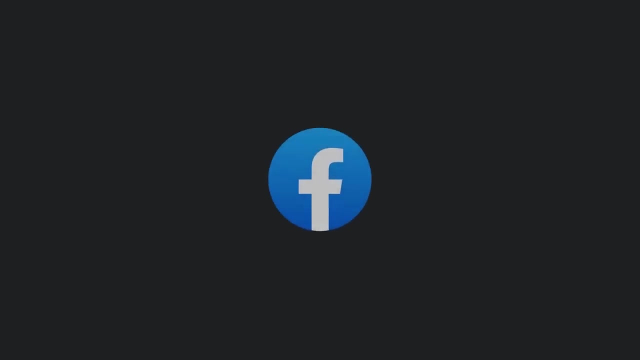 the description. The first 1,000 people to use this link are going to get a month of free Skillshare. Once again, the link is in the description. React is a front-end JavaScript library for building user interfaces. It was developed by Facebook and is maintained by Facebook and the open-source community. 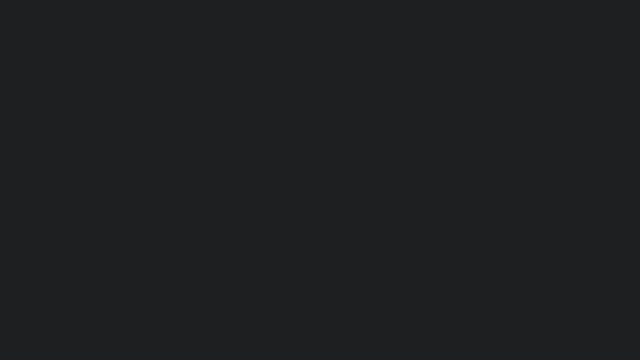 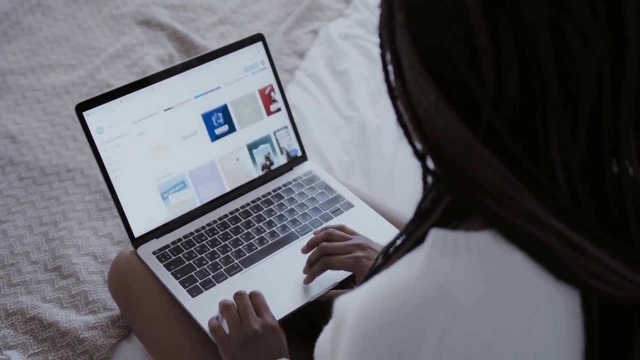 Reactjs is a phenomenal library that is easy to understand, has excellent cross-platform support, has a fantastic community and is one of the most loved libraries out there. There are also two great Reactjs competitors: Vuejs and Angular. These libraries and frameworks are mainly used to create fast and efficient single-page applications. 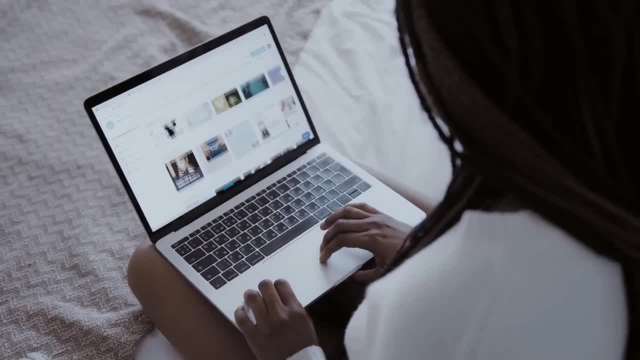 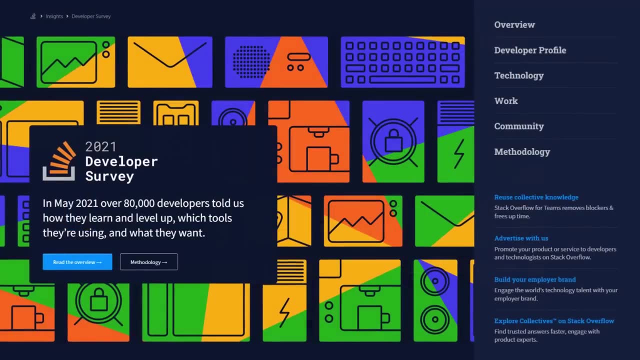 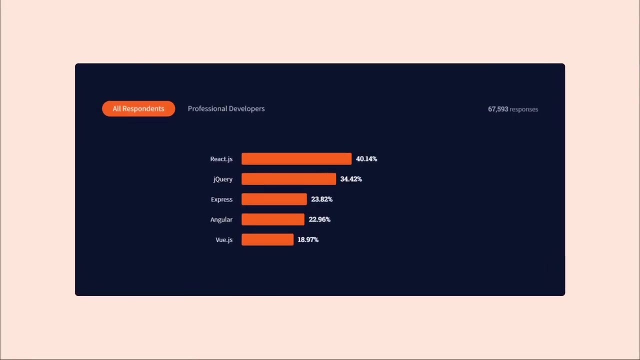 Although these are great technologies, taking a quick look at Reactjs, we can clearly see that Reactjs is still in the lead by far. On the Stack Overflow developer survey, which is the biggest web development survey in the world, 40% of developers chose React. 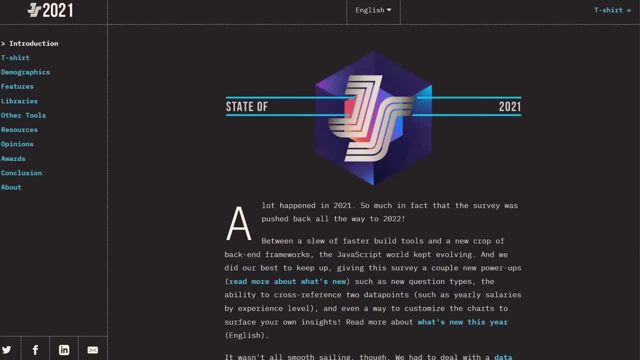 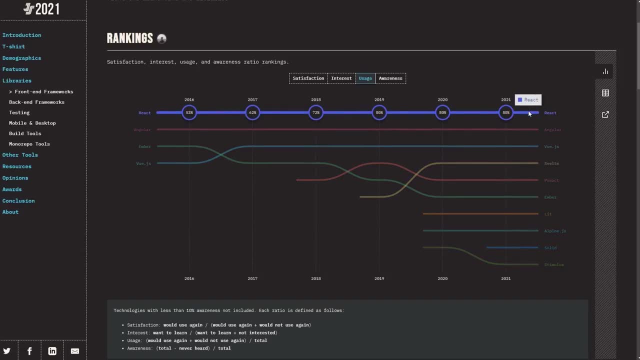 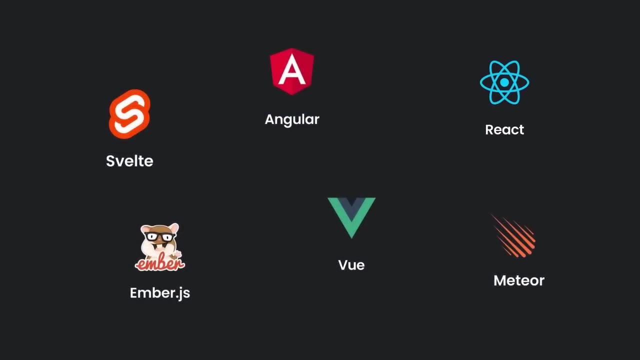 On the state of JS 2021, under front-end frameworks sorted by usage, React has been in the lead for six straight years. With everything I've mentioned, we can safely assume that Reactjs is still in the lead by far. Reactjs is the most popular JavaScript library amongst all other libraries and frameworks currently available. 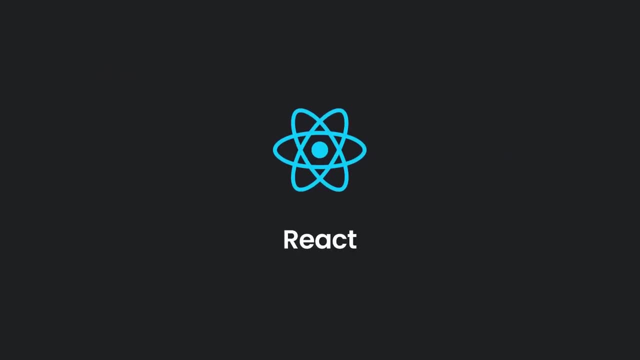 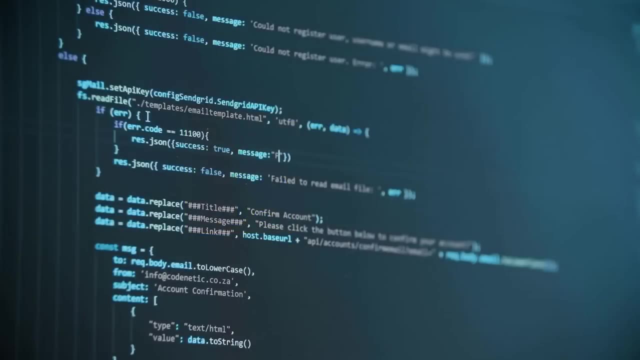 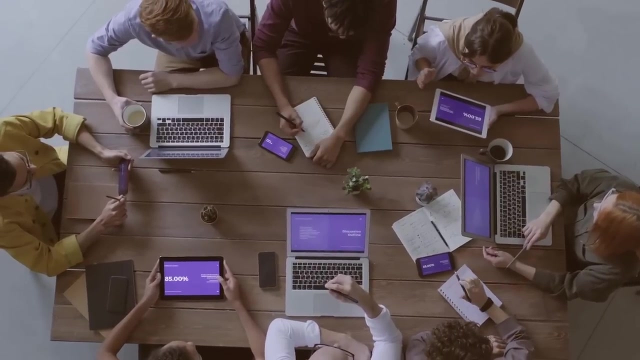 Reactjs also plays a major role in the most popular programming stack, Mern. Mern stack is a JavaScript stack that is used for easier and faster deployment of full-stack web applications. It is designed to make the development process smoother and easier With the Mern stack. 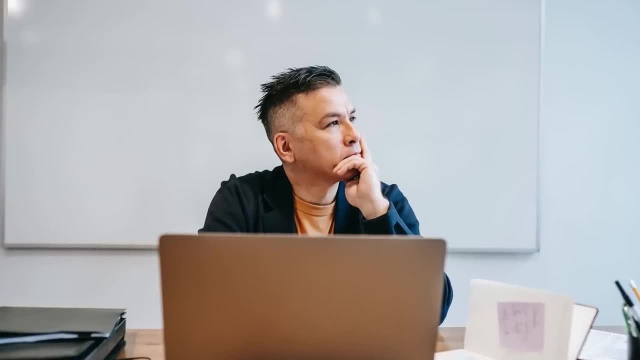 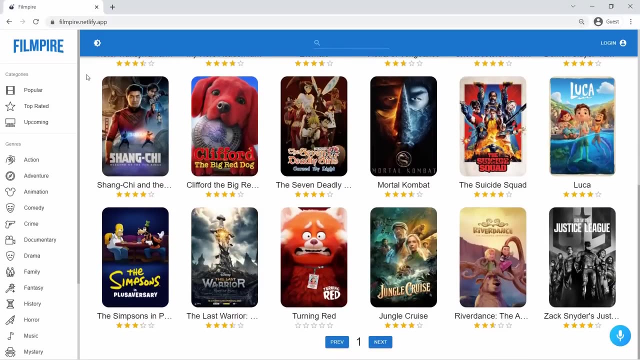 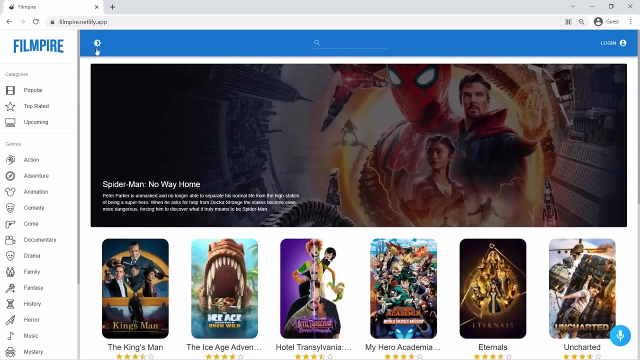 you can create absolutely any web application you can think of. With that said, now let's take a look at Filmpire, the first project-based course of the upcoming JSM Pro platform, which is built entirely in React. Here we can browse around, select a category, select a genre. 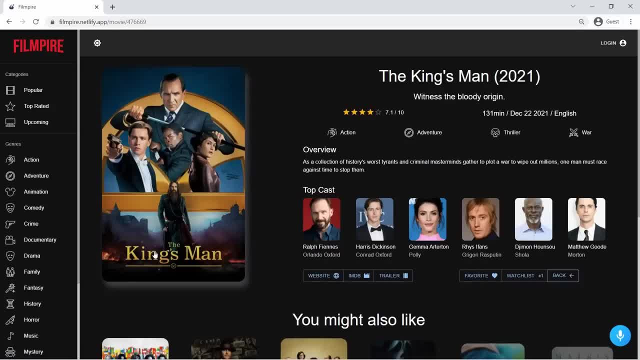 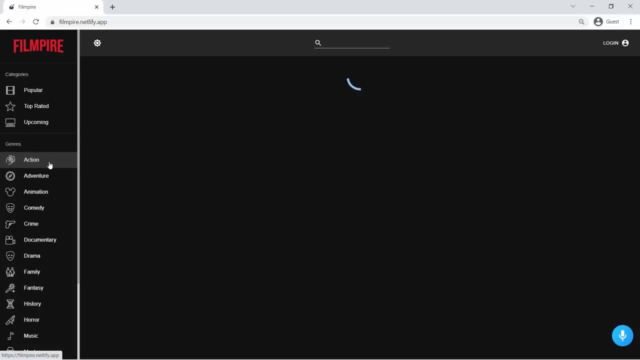 click on a movie poster to see more details about the movie, and everything happens so smoothly and instantly. And you can also notice that the website never reloads. You can see that on the top bar, which means that we don't request and load multiple HTML pages. 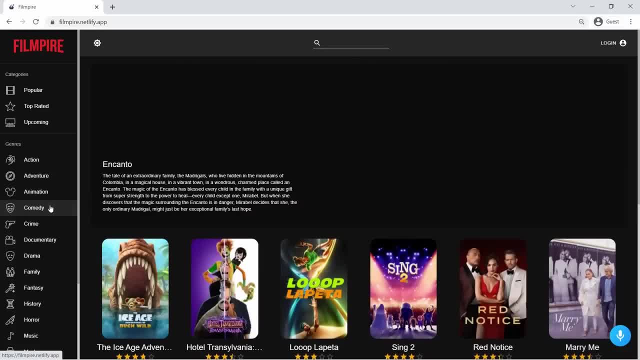 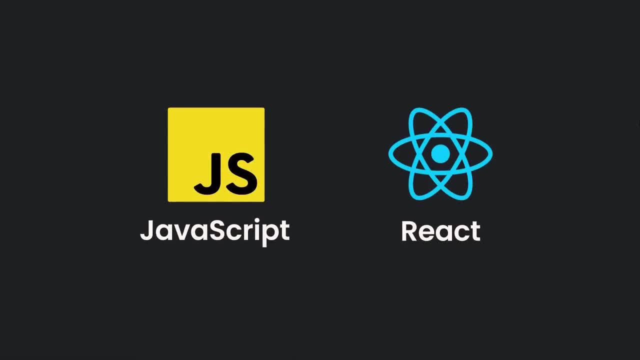 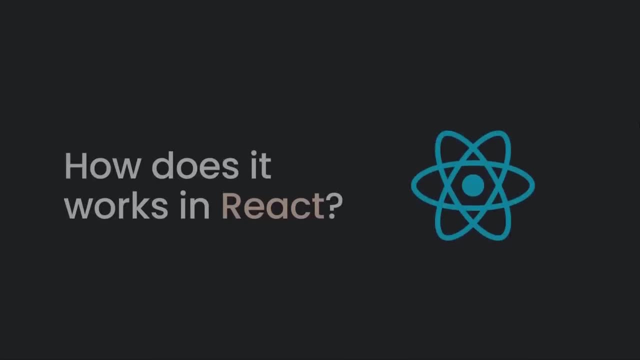 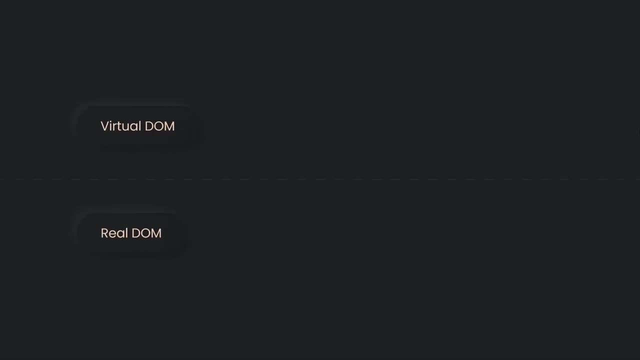 It's a lightweight representation of the DOM. Updating the Virtual DOM is much faster than updating the real DOM. Thus, React only updates the section of the page where the change was made, not the entire page, which is super important. So React uses the Virtual DOM to update the section of the page where the change was made. 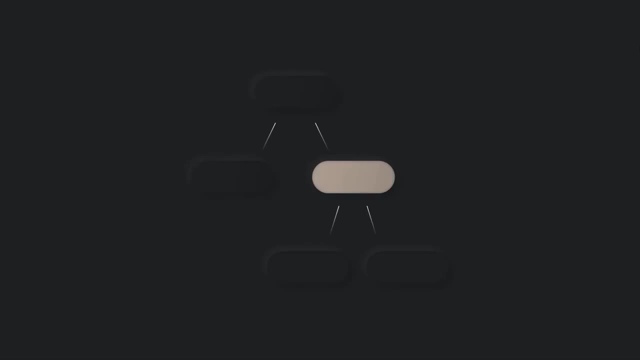 When something changes in a component, we get a new React element. React will then compare this element and the children of that element with the previous one and it figures out what has changed, And then it will update a part of the real DOM to keep it in sync with the Virtual DOM. 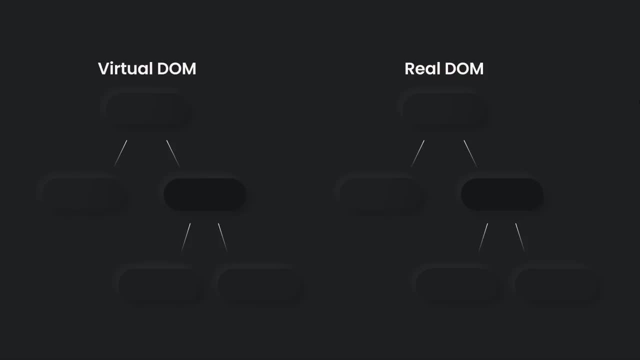 So why does React use this so-called Virtual DOM? Well, because Virtual DOM is way faster than the regular DOM. The main advantage of this is that we don't have to worry about the JavaScript DOM API, and React will do all the heavy work for us. 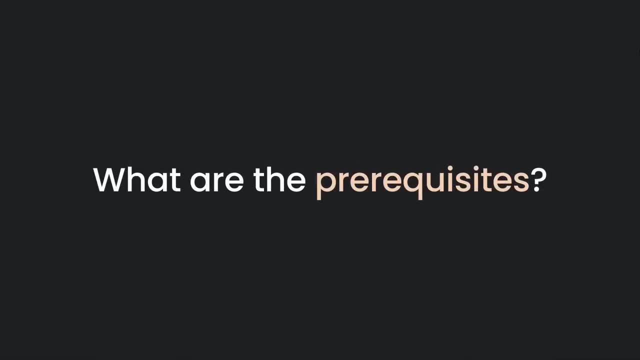 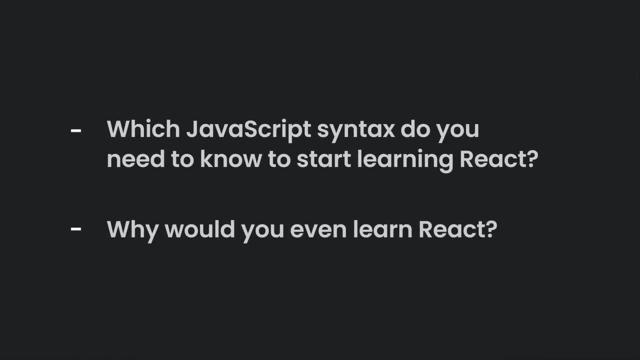 Now you might be wondering what are the prerequisites to learn such a great JavaScript library? There's only one prerequisite, and that is JavaScript. If you're wondering, which JavaScript syntax do you need to know to start learning React? or why would you even learn React and not code everything in vanilla JavaScript? 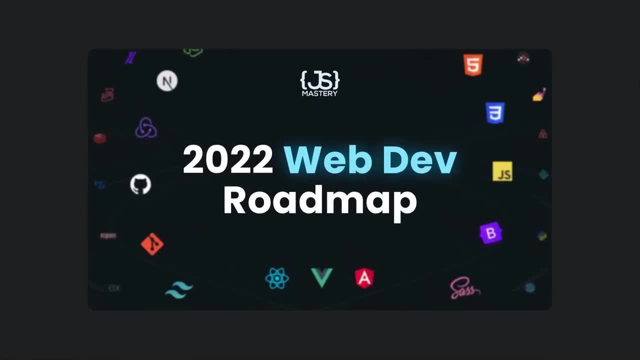 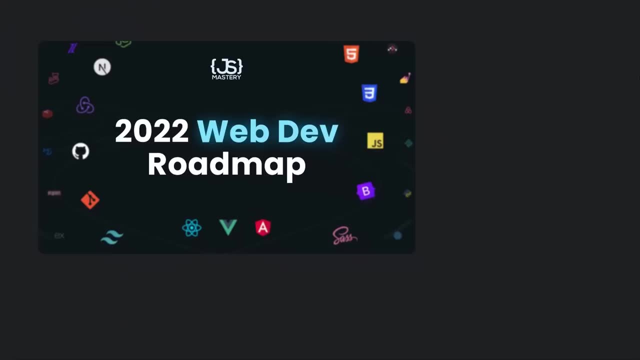 then you must check out my previous video, The Ultimate Web Developer Roadmap. I've answered all of these questions and more in that video. The link to the video is going to be in the description, But if you don't feel like watching the previous video, 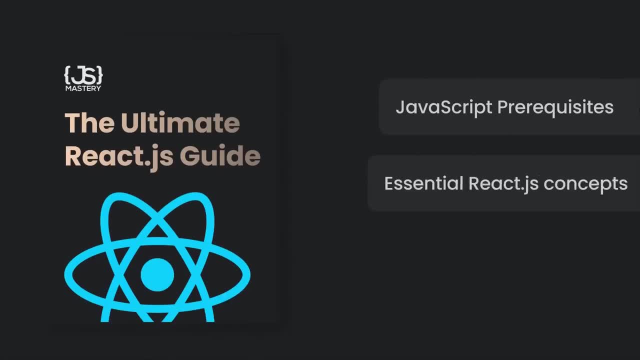 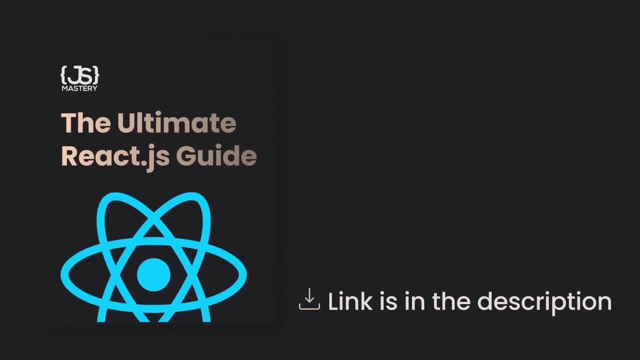 I've also included all the prerequisites, essential ReactJS concept, ReactJS project ideas and more in the Ultimate ReactJS Guide, of course, in the description, completely for free. I hope this makes your life just a bit easier. We cannot talk about ReactJS without talking about components. 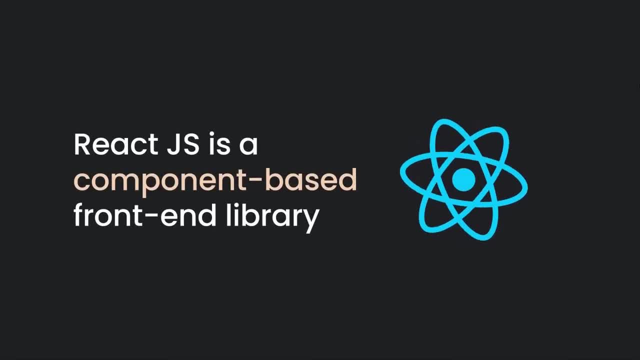 ReactJS is a component-based frontend library, which means that all parts of a web application are divided into small components. A component is a small piece of the user interface. Every ReactJS application is a tree of components. Components: let you split the UI into independent, reusable parts. 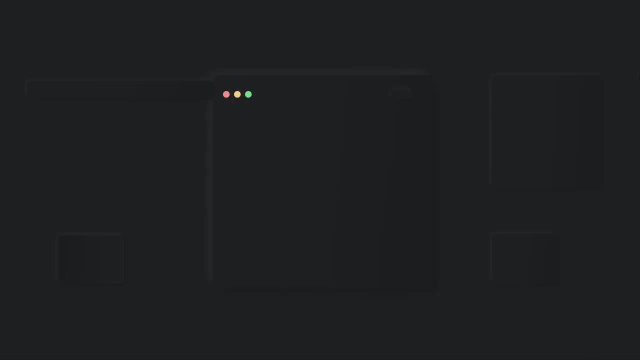 So when you're building an application with React, you'll build independent and reusable components and then you'll combine them to build a full-fledged web application. Let's take a look at the same example I've showed you earlier to represent what are components. 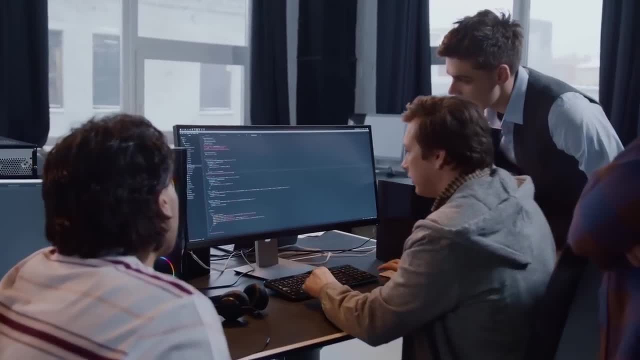 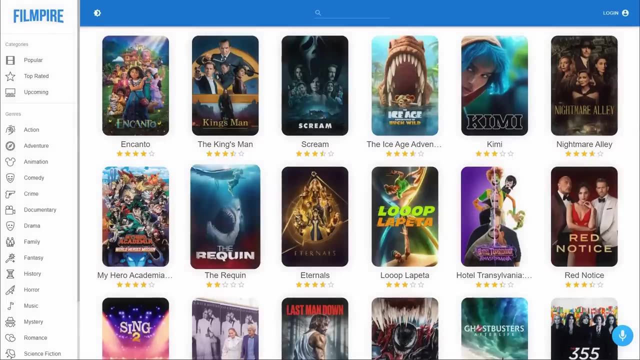 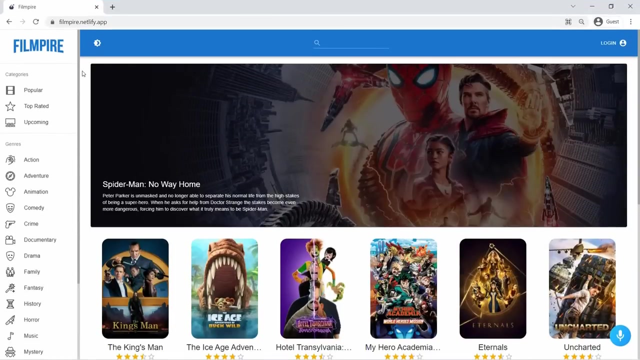 So imagine we're building this website. How would we make it? Firstly, we'll split the user interface into smaller components like sidebar, search bar and movies, which includes several single movie components with names and ratings. I can't even tell you how excited I am to share this course with you extremely soon. 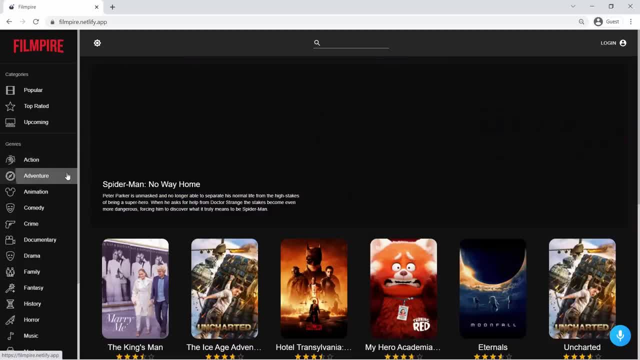 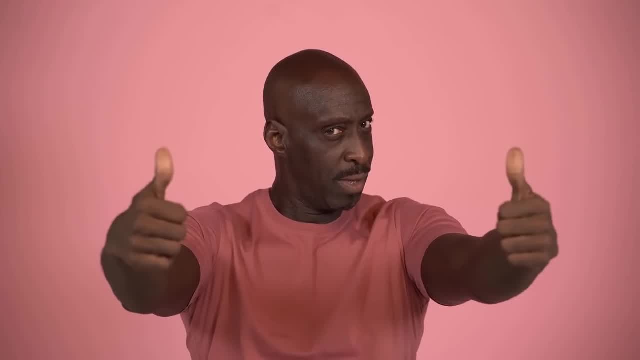 It's been months into making and I'm happy that you'll be able to learn from it soon. So everyone who downloaded the ReactJS guide will get updates about the course and, more importantly, discounts. If you still haven't clicked that download link in the description, now is the time. 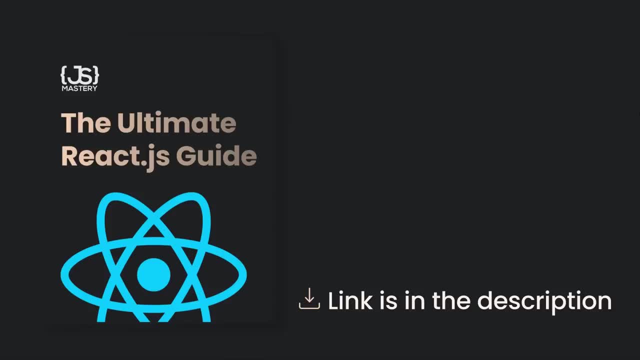 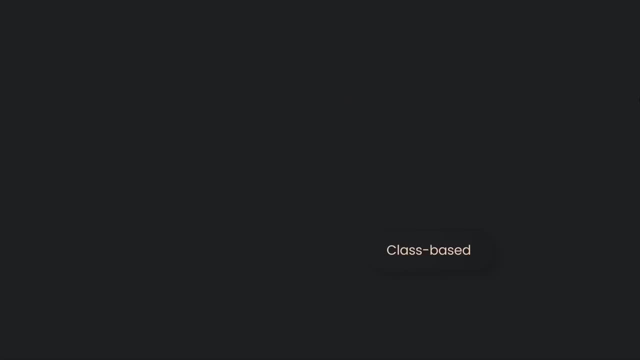 And talking about components in React, there are two types of components: functional components and class-based components. Let's see how does a standard class component look like? Firstly, we import React and the structure component from React. If you're a complete beginner, you might wonder: where are we importing React from? 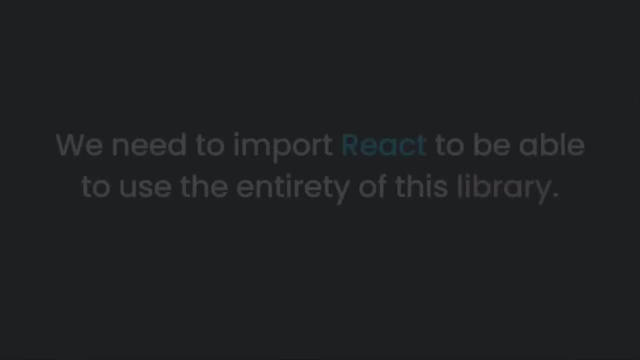 Why do we even need to import it? We need to import React to be able to use the entirety of its library. Then we use a regular JavaScript class to make a React component that extends the React component or the written for us in the library. Then we use the render method that describes: 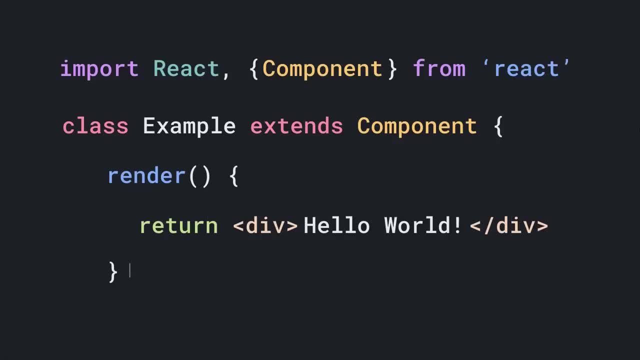 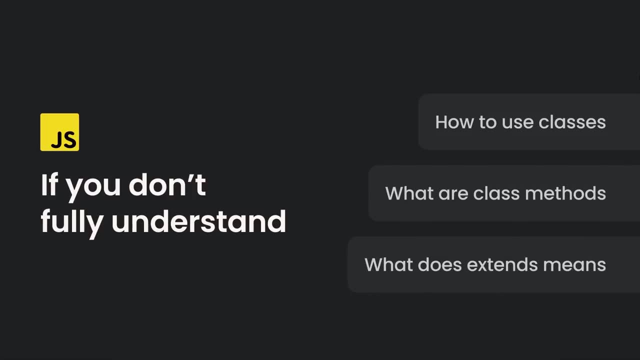 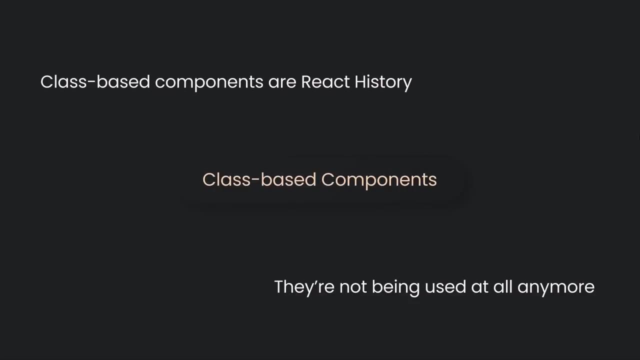 what should be displayed and how should the UI look like? If you don't fully understand how to use classes? what are class methods and what does extends means? don't worry at all. Class-based components are React history. They are not being used at all anymore. 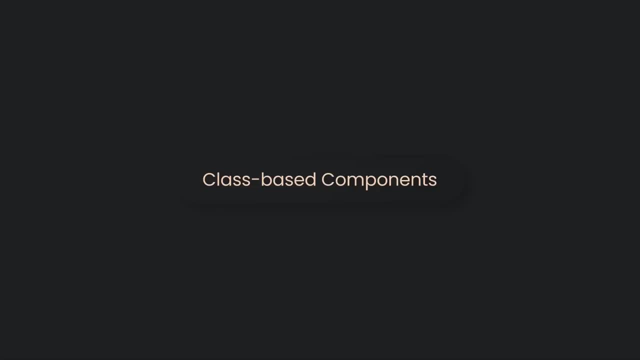 and they are entirely replaced by their simpler counterparts, functional components. Now let's understand how the functional component is written. First, as usual, we import React from React library. Nowadays you can also skip that line In the newer versions of React. it's not needed anymore. 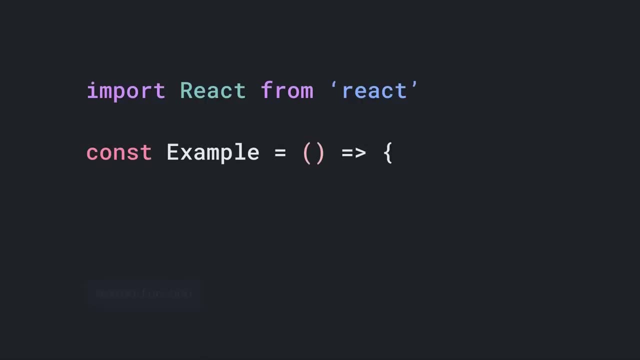 Then we can create a function which can be a normal function, arrow function, named function, whatever you prefer. In this example we're using an arrow function. In the function we return something that React should display. That's it. That is a React component. 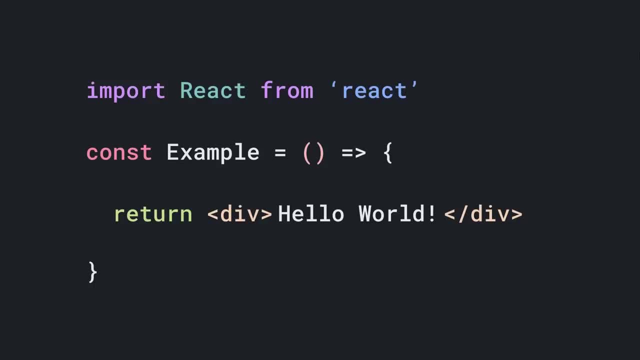 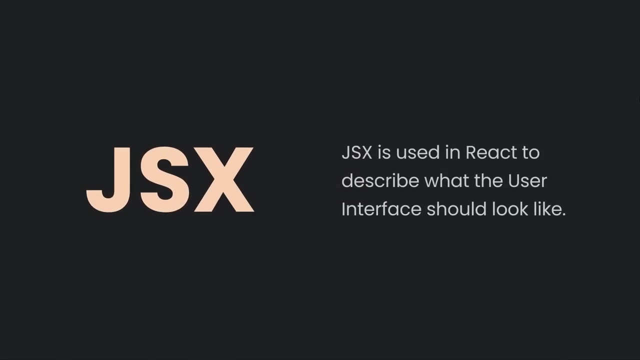 You can see how easy it is. You might be thinking: why are we writing HTML when returning something? The stack syntax is neither a string nor HTML. It's called JSX. JSX is used in React to describe what the user interface should look like. 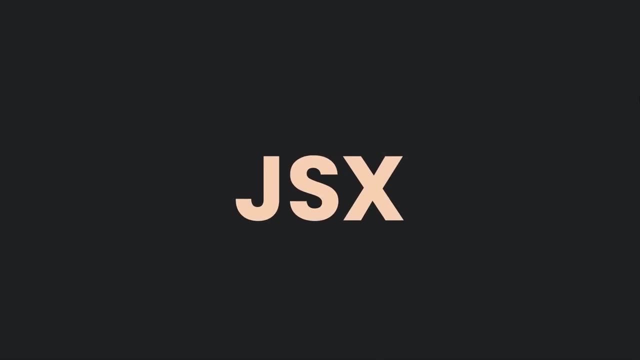 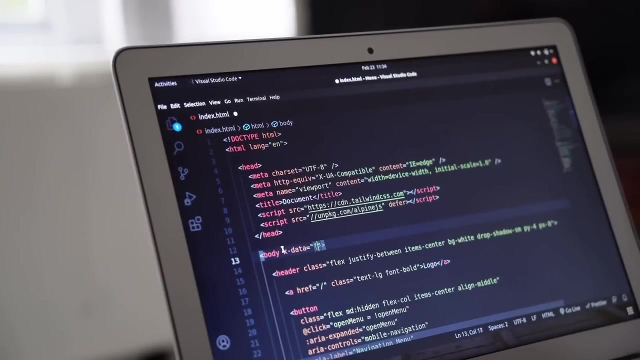 JSX may remind you of a template language, But it comes with the full power of JavaScript. JSX produces React elements. It forms the core of React syntax. So to learn it better, let's dive into code and set up our first Reactjs application. 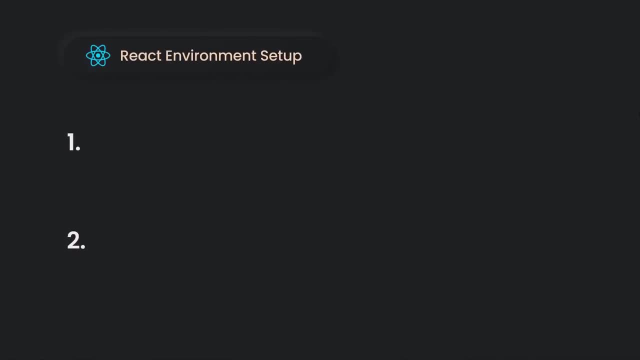 There are two main ways of setting up the React environment. The first one is to manually set it up using Webpack and Babel, And the second one is to use the create React app command. If you're just starting, I would suggest using the second method, as it saves you. 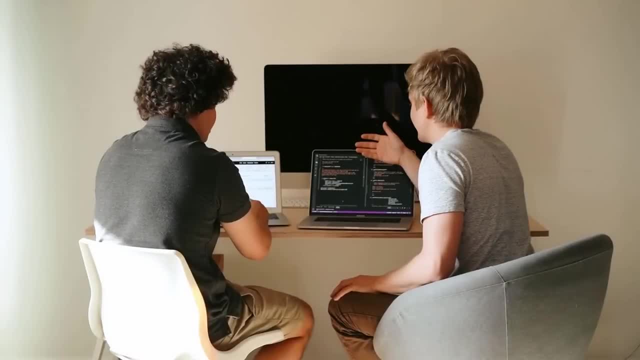 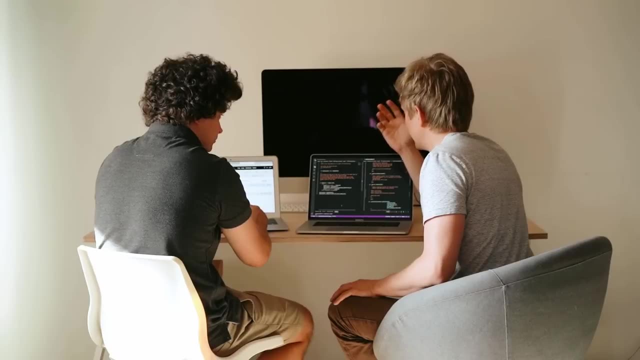 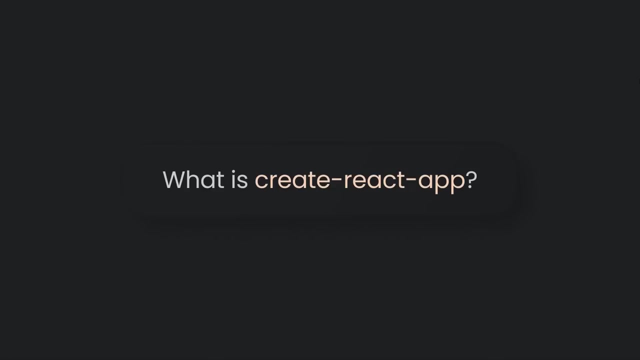 from time consuming setup and configuration. Create React app is a comfortable environment for learning React and it's the best way to start building a new single or multi-page application in React. So what is create React app? Create React app is a simple tool or a 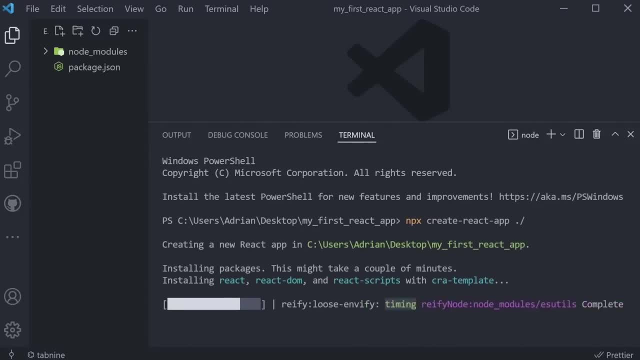 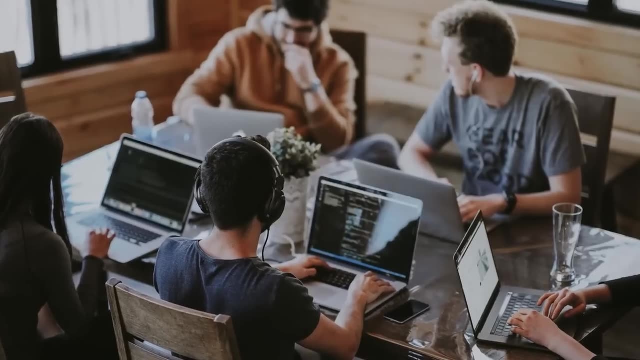 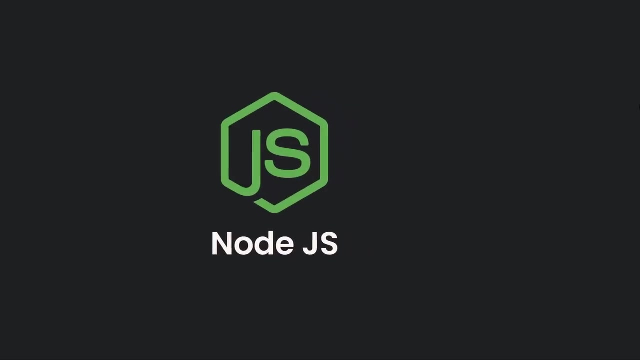 command that generates the required files and folders to start the React application And run it in the browser. It's also officially supported by the React team. To run the create React app command, you need to have Nodejs installed on your PC. Node is a JavaScript runtime that allows you to execute JS code on the server. 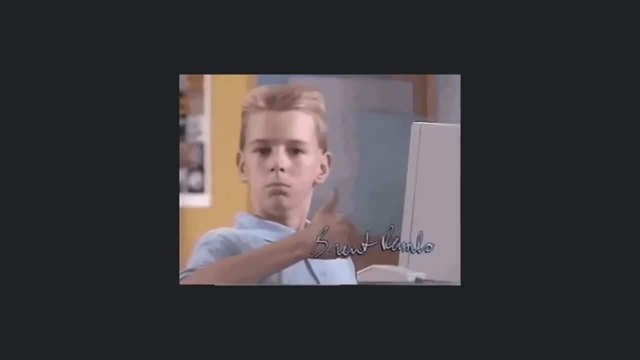 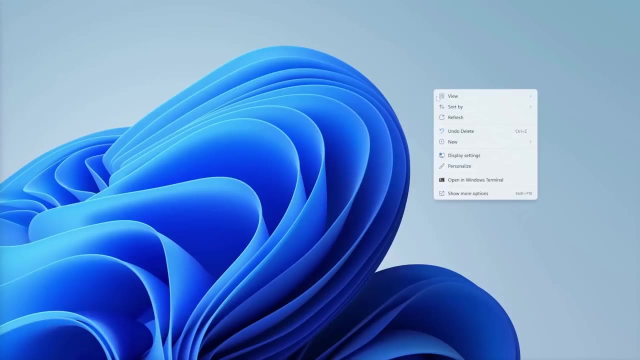 It's highly probable that you already have it installed, But if you don't go to Nodejsorg and download and install it After that, we can create an empty folder on our desktop. Let's call it something like my underscore first, underscore, react underscore app. 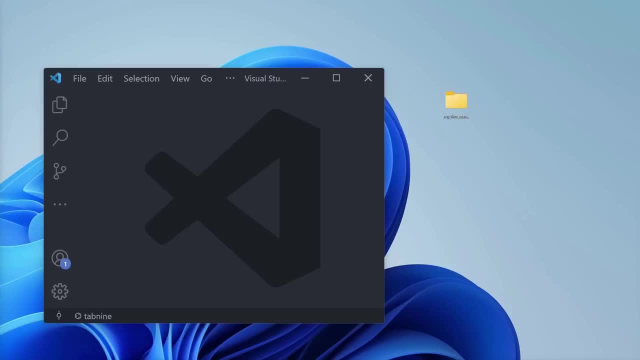 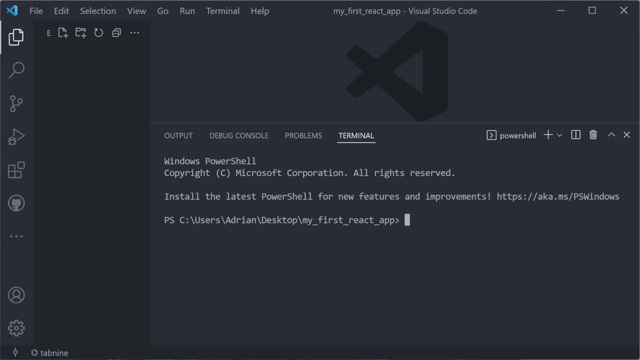 Then you can open up your code editor of choice- In this case, I'll be using Visual Studio code- and you can simply drag and drop your folder into it. Now you can head to view and then terminal. Finally, let's run our first command, which is mpx create-react-app. 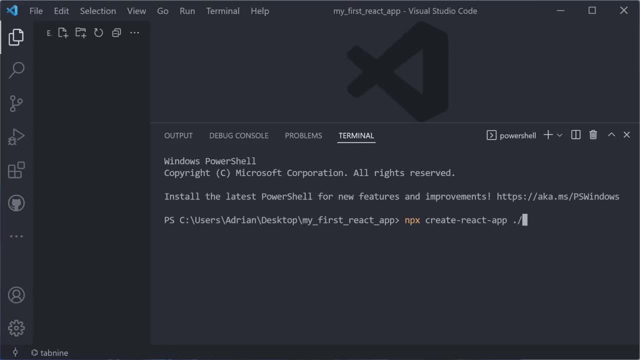 And then tmp player slash URL. I'm going to use the example of mpx create react slash to install it in the current directory. Let's press enter. You might get an additional message here, because this is the first time you're using create React App. 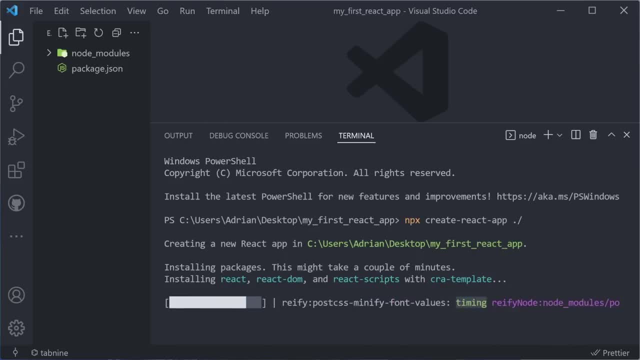 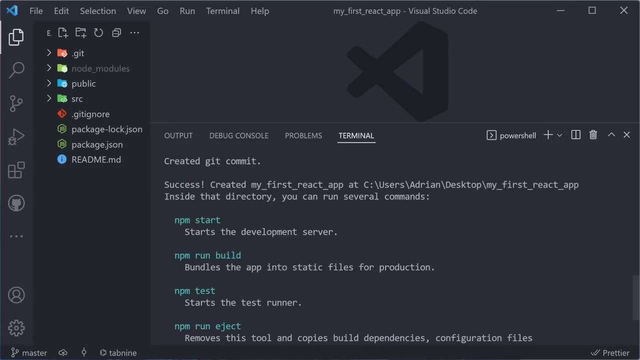 But after that you should be able to see creating a new React App and then your directory. this is going to install Primary React packages like React, react-dom, React scripts. This process usually takes about a minute, So success created my first React app. 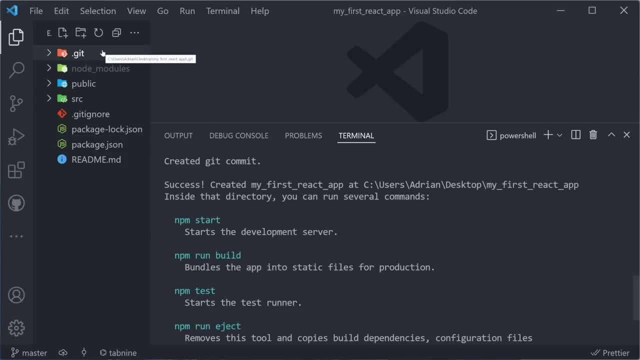 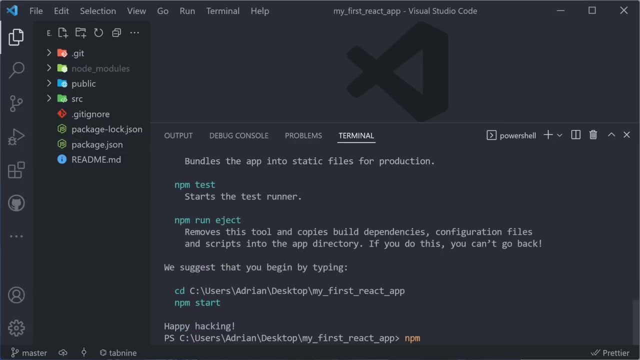 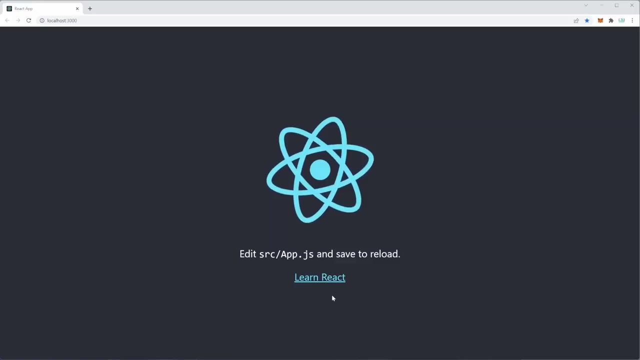 This command just generated all the files and folders needed for your first React application, So let's run it. You can run your application by running npm start and then press enter. This is going to run our application on localhost 3000. And in a few seconds, there it is rotating ReactJS logo with a text that says: edit source. 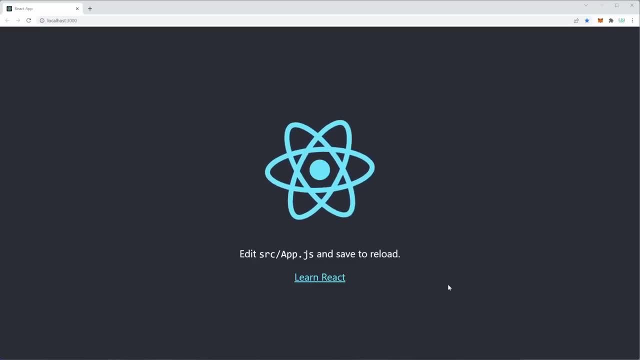 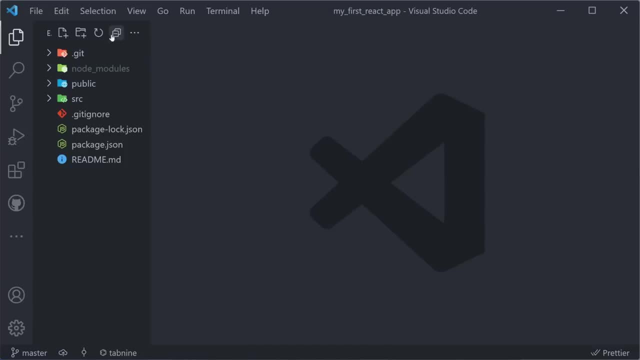 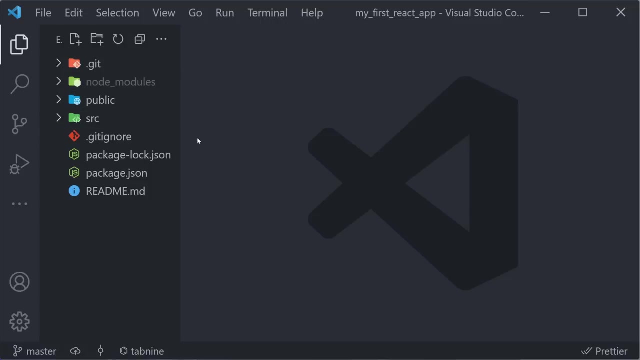 appjs and save to reload. That way we'll be able to modify our ReactJS application. But before we do that, we can take a minute to properly explore the file and folder structure of a ReactJS application. Over here you can see all the files and folders. 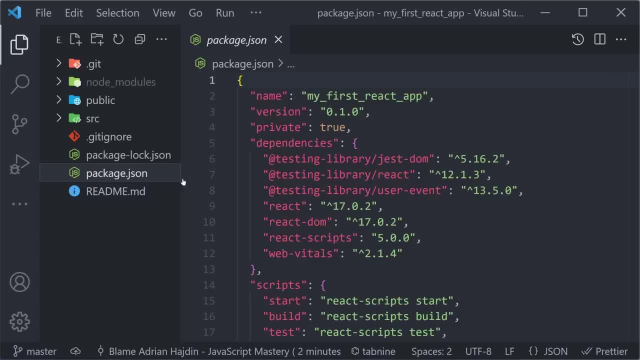 Let's check them out. The first one is packagejs. Inside of here you can see all of the dependencies or packages that your application currently has installed. As you can see, the core ReactJS packages are right here, And then all the other npm packages that you install later on are going to be added here. 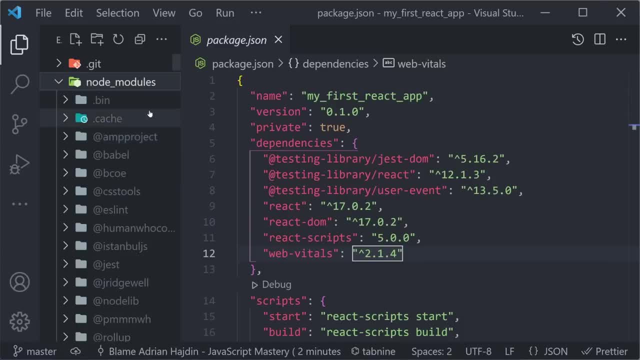 as well. The code for these packages is going to be added in our huge node modules. This is not the folder that you have to manually explore. It's just there and it serves the code, The src, src, src, src, src. 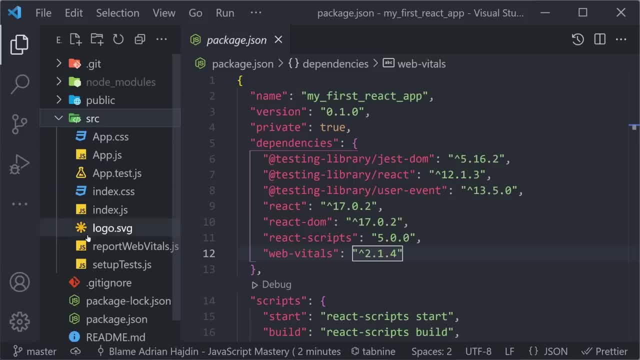 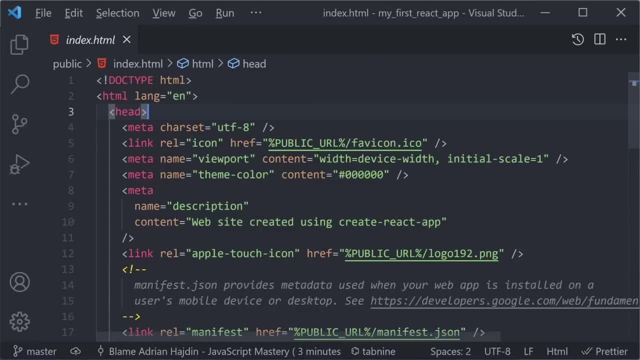 code versions. Of course we have a message up in theuis: More millennial. These are our top 8 code versions that we also handle, and we are kind of low on power up there right now, So do you wanna give it a try? 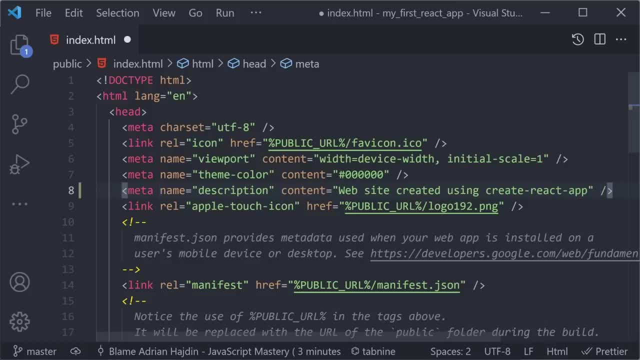 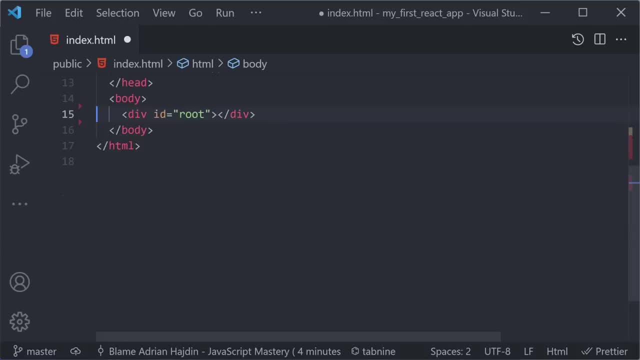 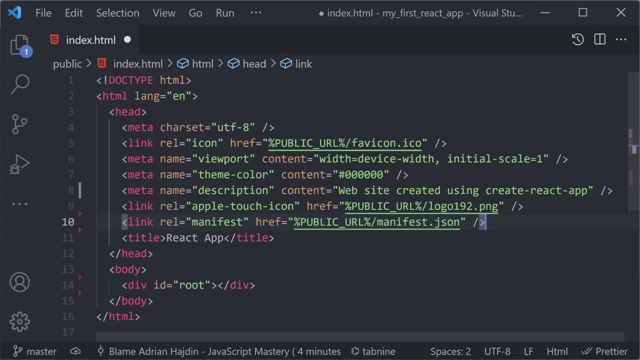 Let me try some. Let me try one here. Let me try one. okay, comments that we can delete. a few link tags, some kind of a big comment right here and that's it. If we remove all of the unnecessary things, we are left off with the simplest possible. 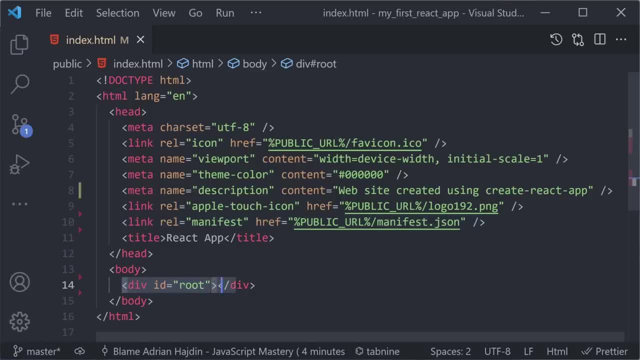 HTML document that has only a single div with an ID of root. The way React works is that all of our React components are going to get injected inside of this div with an ID of root. To properly explore that, we can go into source and then indexjs, the starting point of every. 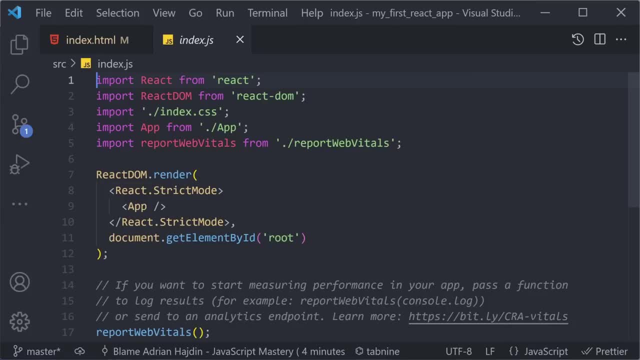 Reactjs application. Inside of here we have React DOM, which we only call once in our entire React application, no matter how big it is. React DOM is used to render our components and our entire application into the real DOM, more specifically, into a div with an ID of root. 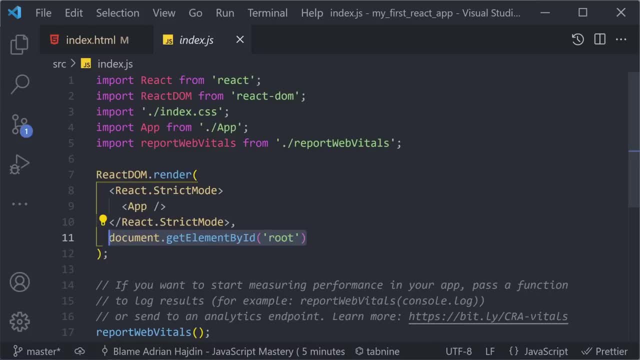 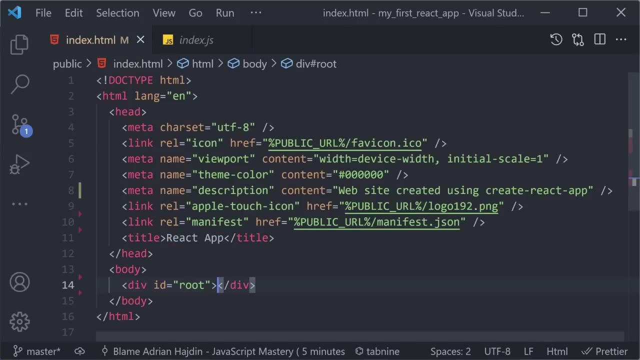 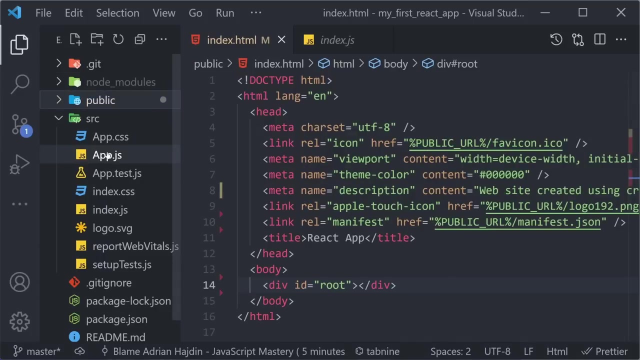 This is how we're accessing the basic DOM. we target this div and we populate our entire React application and we inject it right here. That is the base premise of how Reactjs works. Now, if we go to explorer source and then appjs, you can see that we have a functional. 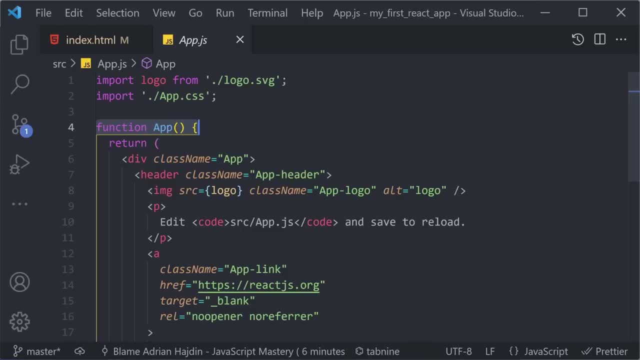 component, something that we've discussed before. Remember what I've said earlier: Functional components are the ones that are primarily used nowadays. No more class-based madness, And this code that you can see right here, that is not HTML, This is JSX. 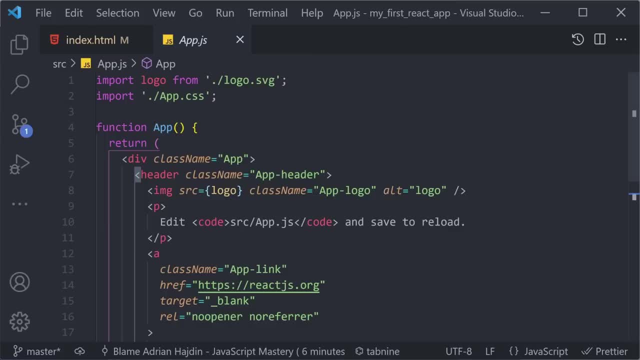 Because you can see it is in a js file, not in a html file. There are a few differences between HTML and JSX, although generally it's incredibly similar. One of these differences is that you can notice class name. Usually in HTML you would write that as class. 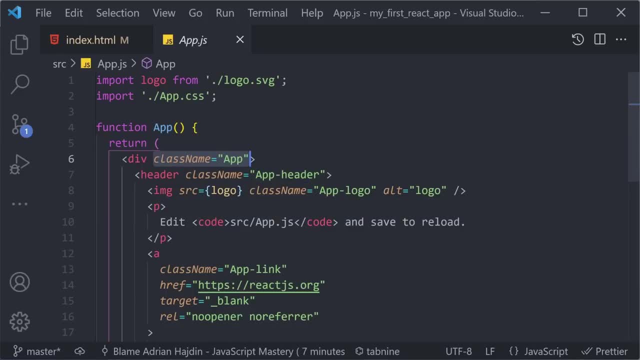 But class is a reserved keyword in JavaScript, so we had to use class name. Since we use JSX in React, the extension of JavaScript, we have to use class name instead of that class attribute. So keep that in mind. All of the similar gotchas of using JSX are also linked in our Reactjs guide, so make 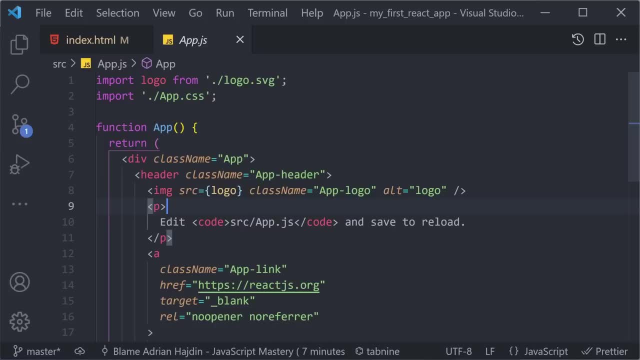 sure to go for it if you want to get more information on the JSX syntax. Inside of curly braces you can put a class name, For example, class name. You can also put any valid JavaScript expression. So in here we're dynamically assigning a logo to this image. 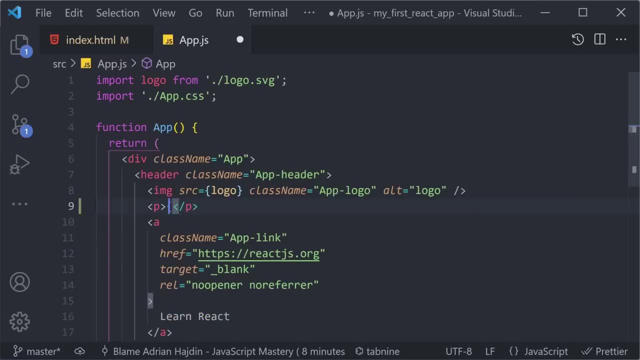 For example, we can remove the text inside of this paragraph, open up a pair of curly braces and write 2 plus 2.. In HTML, the only thing that you would get would be curly brace, 2 plus 2, and then curly. 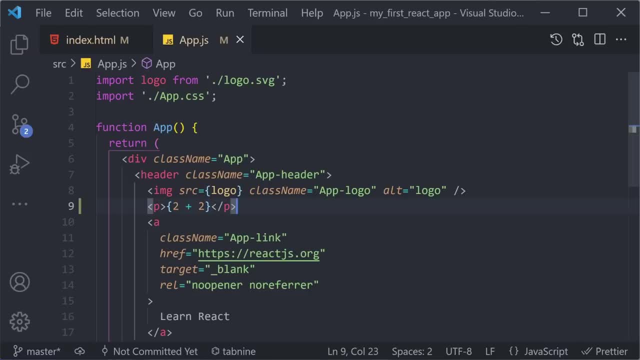 brace, Literally. But now, if we go back to our browser, as you can see in here, we have 4.. And that might seem incredibly simple and not meaningful, But think about the power that this represents. You can write JavaScript code straight inside of something that looks like plain HTML. 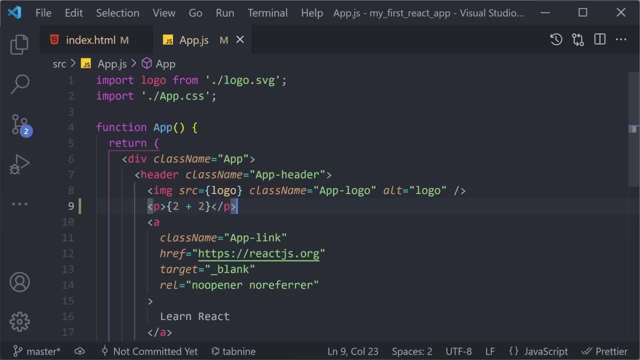 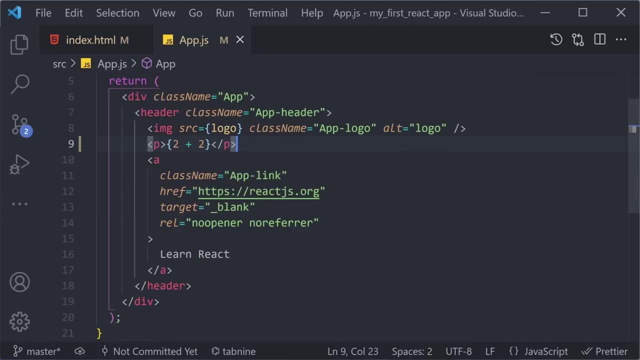 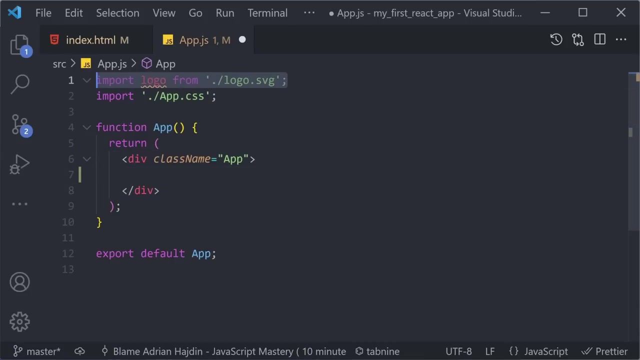 That means that you can dynamically render real data inside of your browser. Isn't that cool? So now let's delete this demo example by deleting all of the code inside of it. We can leave the div with the class name of app, And let's also delete this logo, because we're not using it anymore. 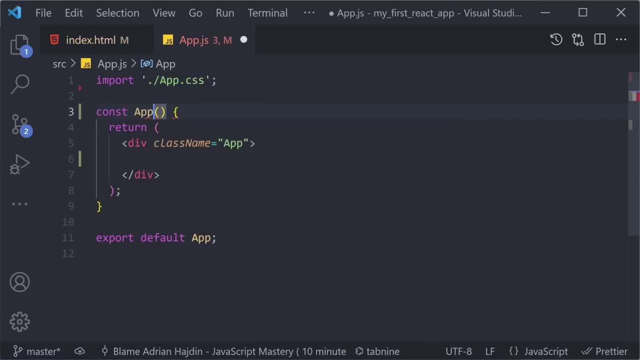 We can also convert this function app into a const app And that is an arrow function component. Inside of there, let's simply create an h1 that's going to say hello world, Or rather, let's do hello react And let's save it. 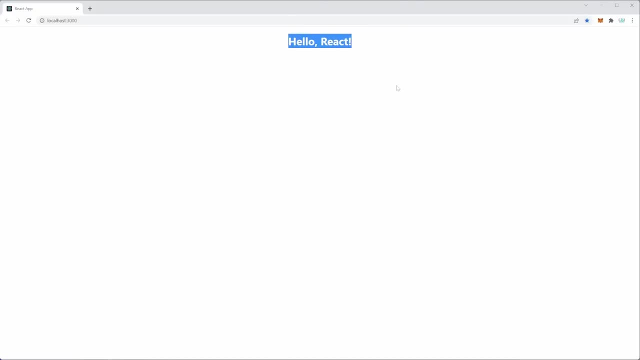 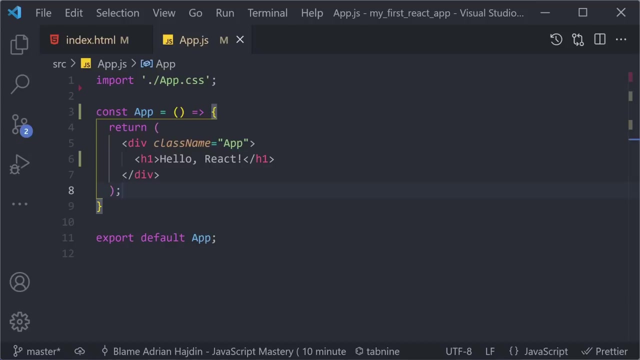 And there we go, An h1 that says hello, react. Now we can dive deeper into the syntax And explore all of the benefits that ReactJS offers. Let's go ahead and get started with the real thing. Before I start showing you all of the benefits that React offers, let's open up our browser. 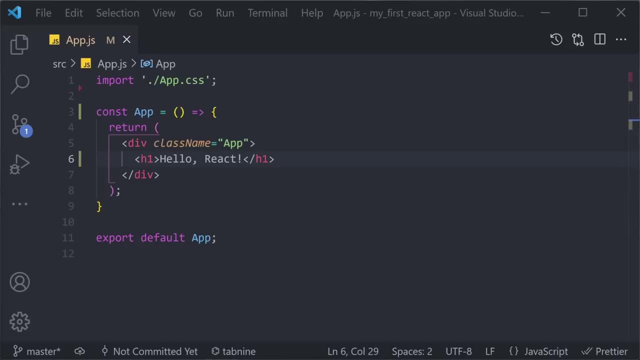 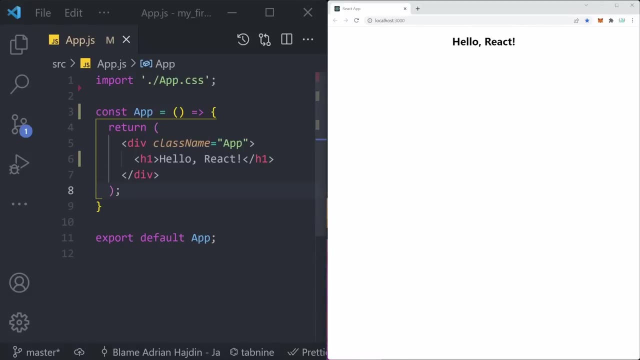 and put it side by side with the editor So that we can see in real time the changes we're making. There we go. I've put the code editor on the left side and our browser on the right side, So now, if we type something, 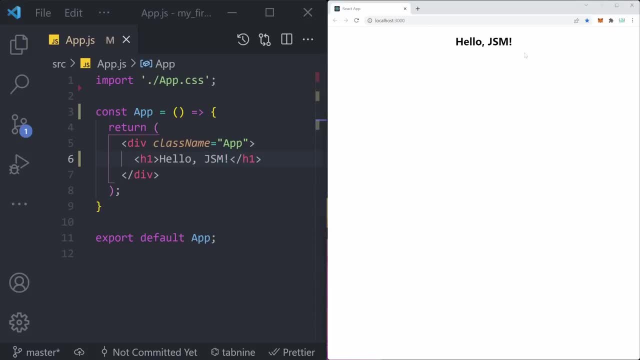 For example, hello JSM And save it, You should be able to see the code update in real time. So now let's explore that dynamic or reactive nature of React. We can create different variables right here inside of this functional component. 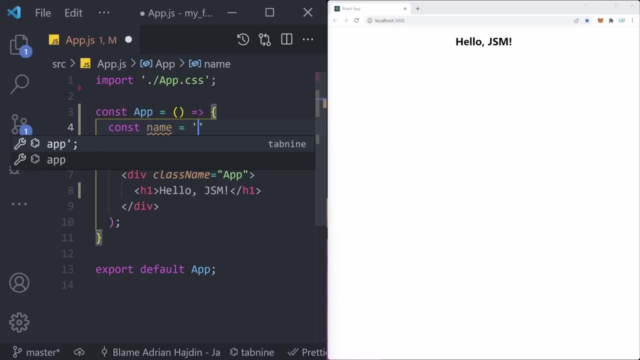 So by saying something like const name is equal to And let's do something like John- We can use this variable inside of our JSX. So, right here, we can open up a pair of curly braces Like this And simply reference this variable inside of those braces. 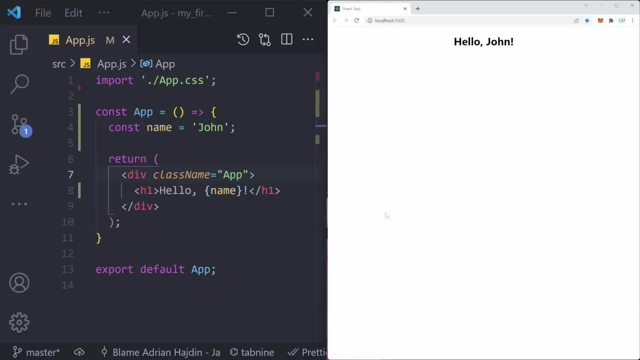 If we save that, you can see. hello, John. Now this might seem like magic, Because this seems just like basic HTML, But we've just injected real JavaScript code straight into it. That is the power of React. We can also do something more powerful. 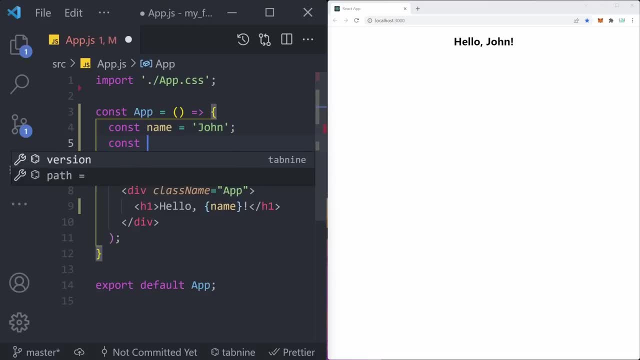 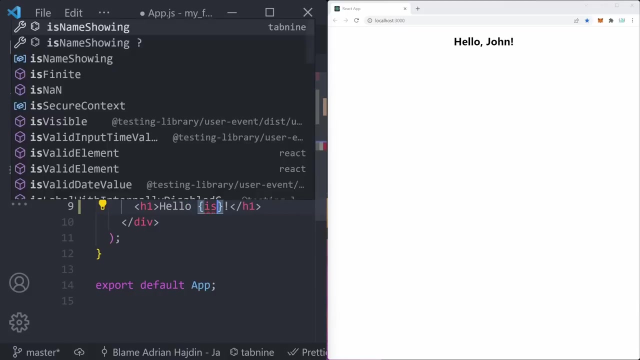 Like: create different ternary expressions. Let's create a variable: is name showing Like this And that's going to be set to true Right here. what we can do is say hello And then we're gonna check if is name showing is set to true. 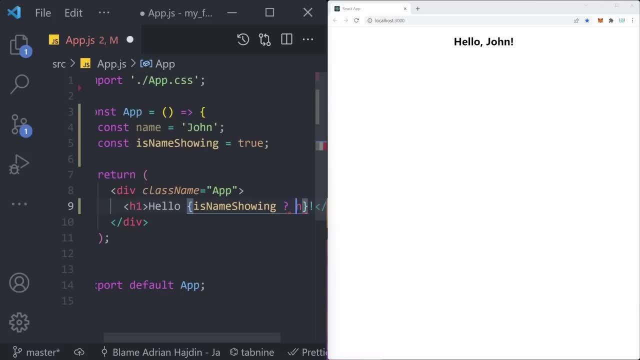 If that is the case, then we can simply show John Else. we can say: let's do something like someone. Now, if we save that, you can see that we're showing hello John. But now if we switch this variable to false, 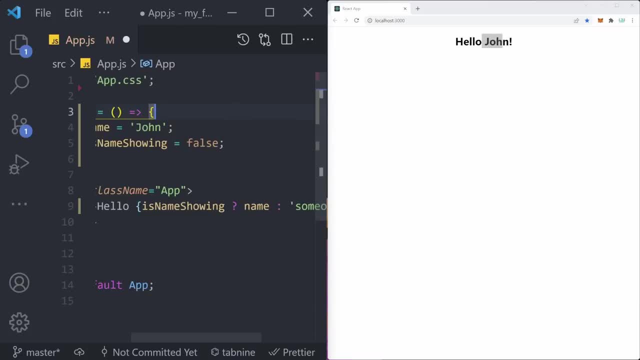 Is name showing false? Is name showing false, Then the different part of the ternary expression is going to be ran, And now we can see: hello someone. With this, we've just made the render of our application dynamic. We're gonna show a different display based on different dynamic data. 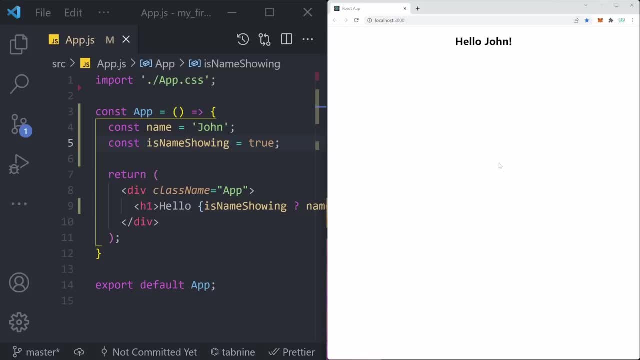 You wouldn't be able to do this this easily in just basic HTML and CSS. Of course. take your time and play with this a bit. You can explore all of the other possibilities that React offers. We're just showing the name here, But you can do any kind of arithmetic. 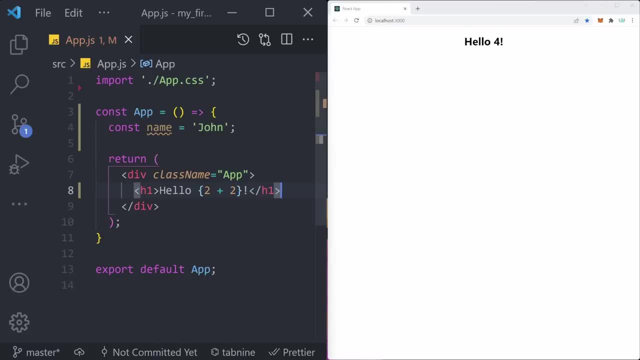 Like: 2 plus 2 is 4.. That's going to show up. Using these expressions, we can dynamically render larger blocks of code. So if we open up curly braces And then check if name exists, In that case we want to render this React fragment inside of these parentheses. 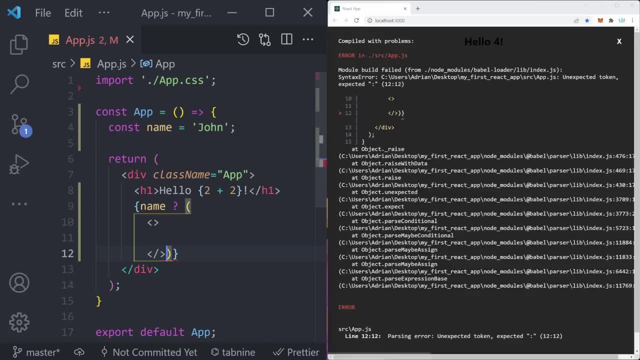 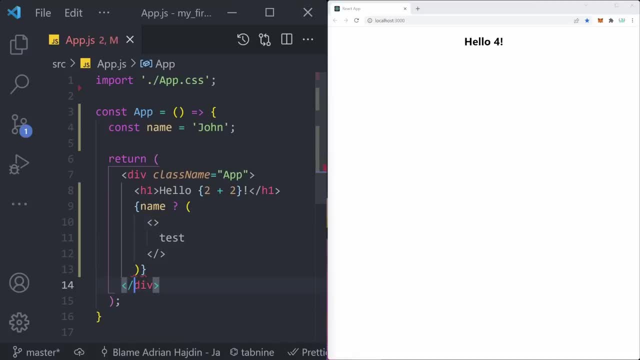 And a React fragment is just like an empty div. Inside of there we can put some code. So let's say test for now. And then of course we need to have a second part of our ternary expression And inside of there we're going to say test as well. 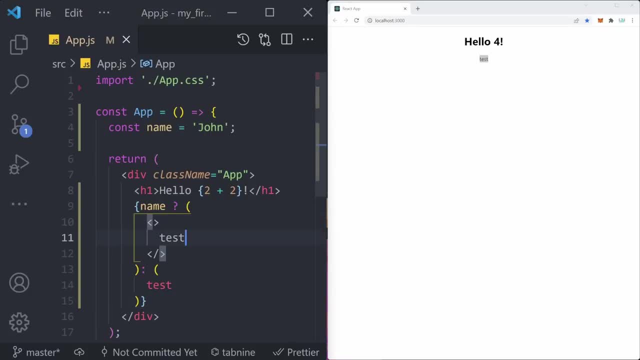 There we go. We can, of course, see test, But why do we even need this empty block, So-called React fragment? Well, let's say that instead of test at the bottom, we want to show something like an h1.. 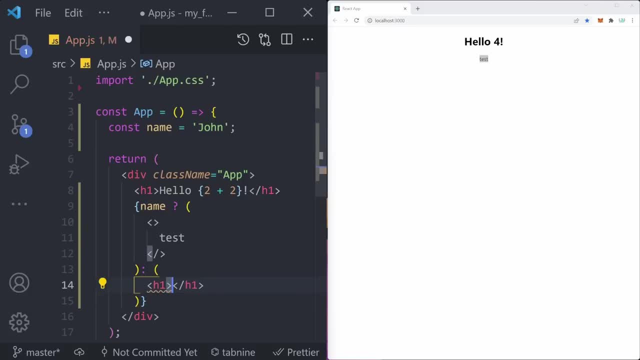 Let's close it properly, And there we're going to simply say test, Because we don't have access to it. We don't have access to the name in this block down there. Now let's set the name to be null. 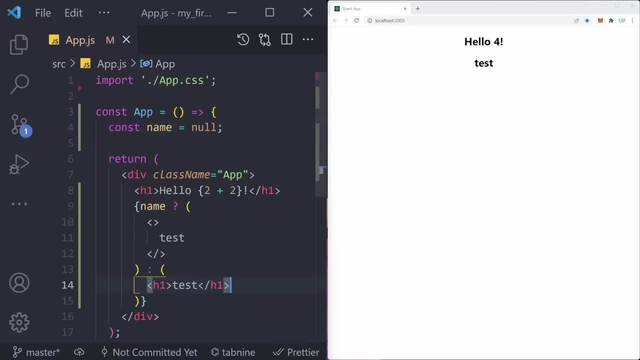 So the below expression is going to run. We can see the test. But now what if you want to add a second h2? that's going to simply say there is no name. If we save that, you're going to see a really often appearing error. 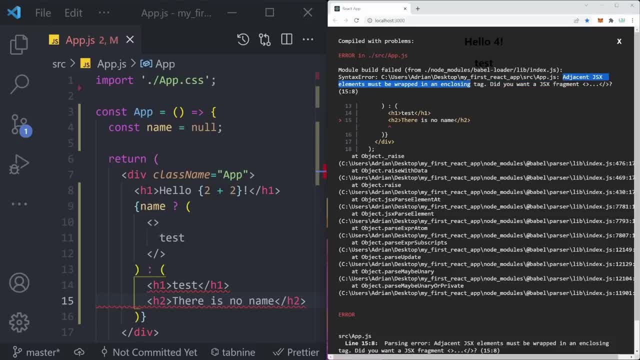 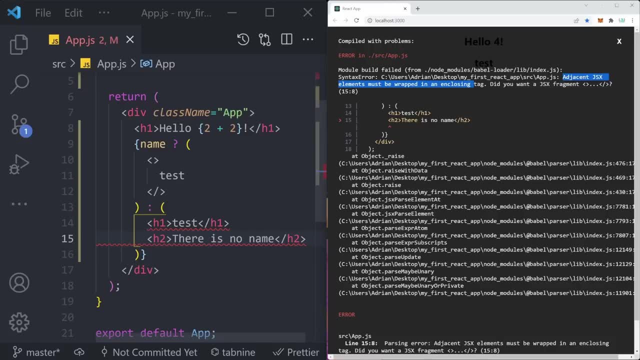 Ejectant JSX elements must be wrapped in an enclosing tag. So this is a rule that React has. If you want to render two different elements one next to another, you need to wrap them in a so-called React fragment. So right here, what we can do is just wrap this in a fragment like so: 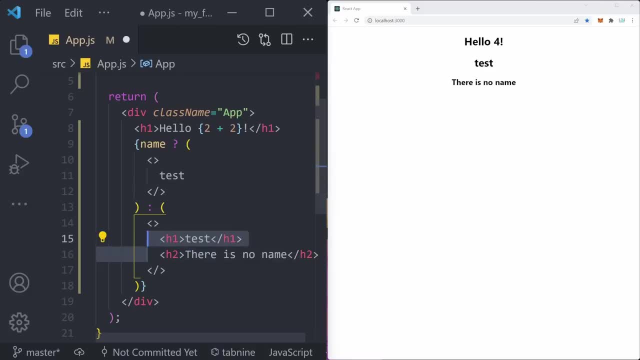 And then we won't have an error anymore. There we go, So below we're saying there is no name, And right here we can say h1.. And of course we can render the name inside of the curly braces. 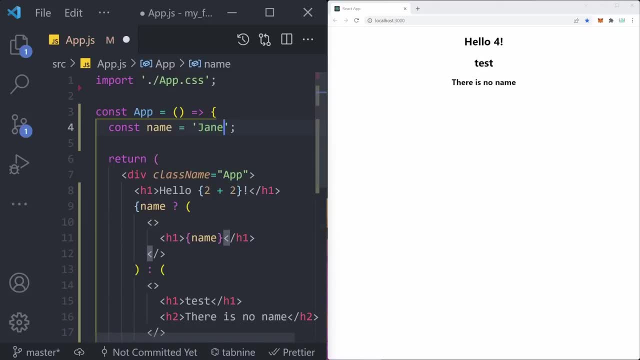 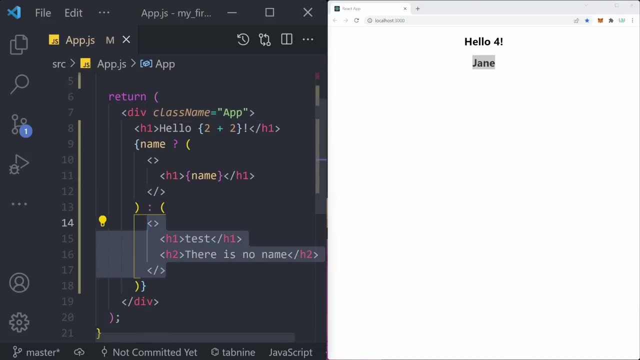 Now, if we change this to Jane, Save it, You'll be able to see Jane, And otherwise, if there is no name, you'll be able to see this block of code down there, And right now we're working with just two different tags. 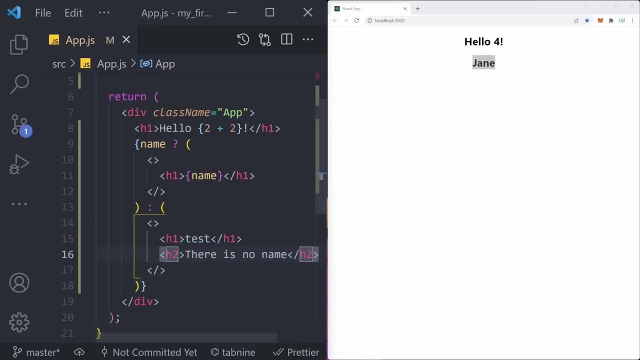 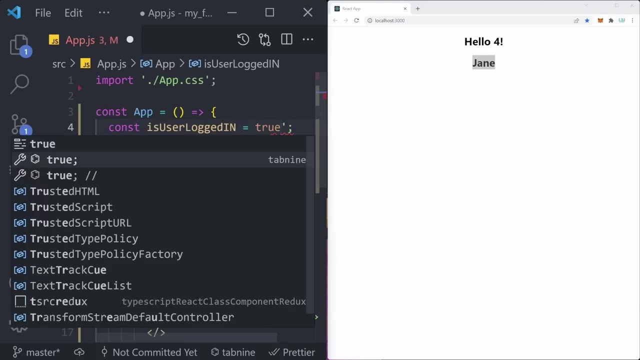 You can do the same thing with thousands of lines of code and completely change the user interface when something changes. For example, you can have a variable: is user logged in? And let's say that the user is logged in. In that case you can show some data and display his user profile. 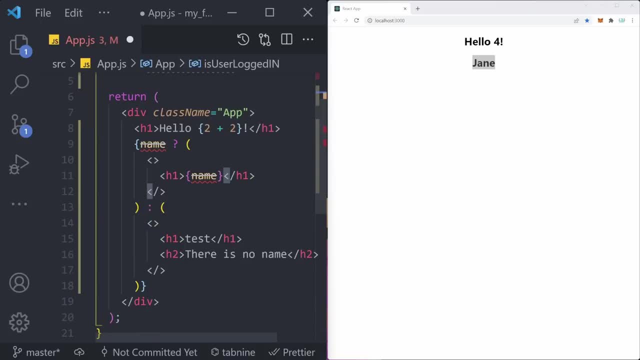 Else, you can simply render a login button. That just shows you that there is a lot of possibilities. Now let's dive into one of the core React topics, And that is components. We can create many different components and then import them into our larger components. 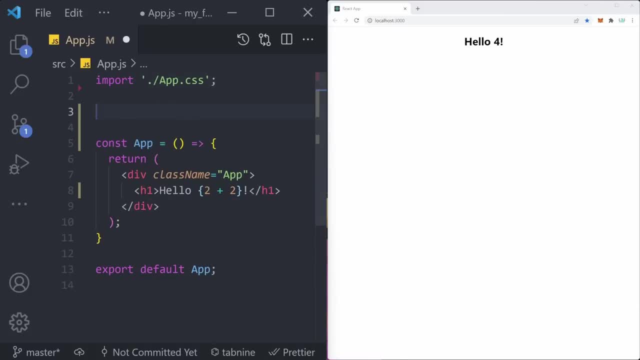 So, for example, we can create a new component just above the current one. that's going to be called person Const. person is going to be a functional component And it's going to have a return statement. For now, let's simply return an H1. that's going to render. 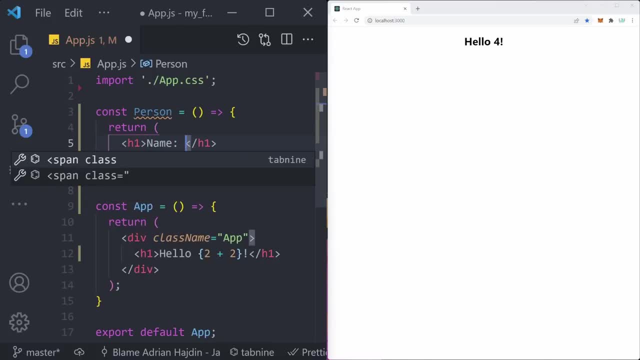 Let's do name, And then that's going to be set to John, And then we're going to wrap it in a React fragment so that we can add something below that We can simply say H2. And then we're going to do last name. 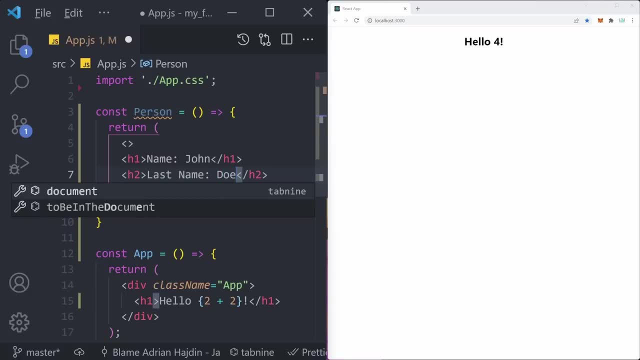 It's going to be dough As well as the age, And let's do something like 30.. So this is our person component, And a component is a piece of code that returns or renders some JSX, And in here we can call our person component by its name. 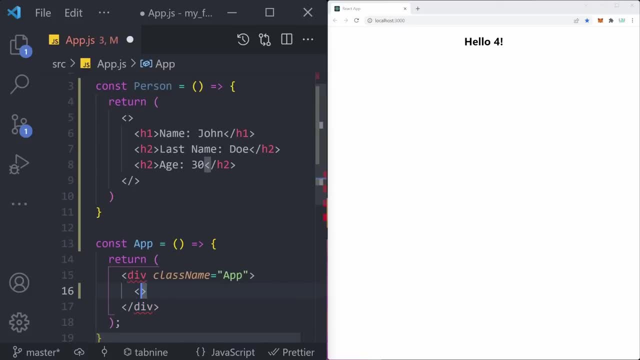 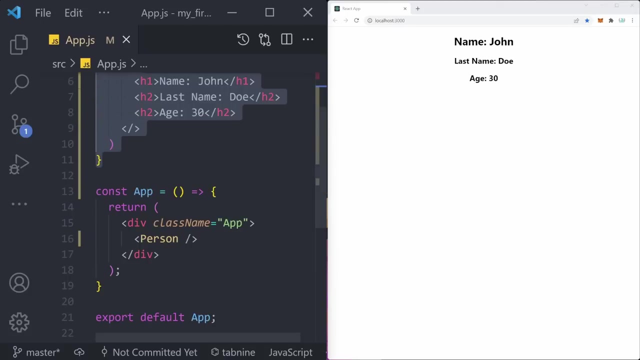 Take a look: It's called person. The only thing you have to do open up a code brace and start typing person And then simply close it as a self-closing tag. As soon as you do this, you'll be able to see that all of the code from the above component got imported or injected straight right here inside of the app. 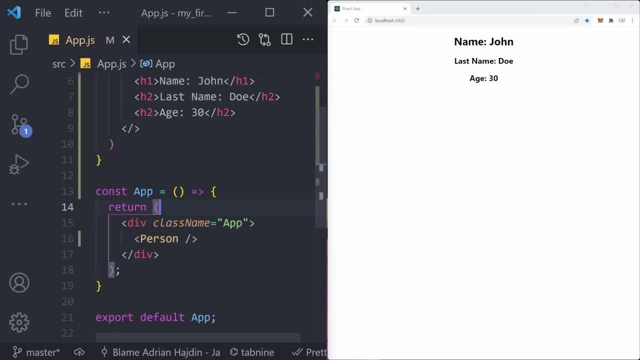 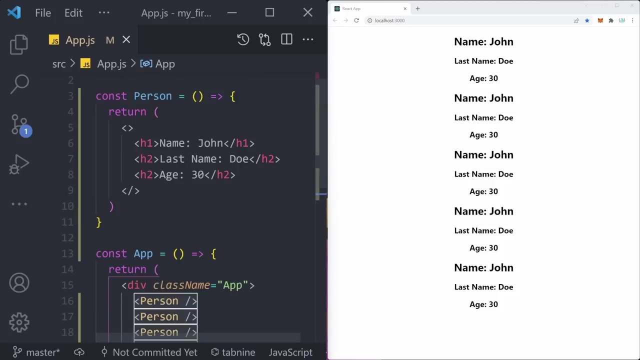 Isn't that crazy. One advantage of creating a custom component and then referencing it right here is that we can duplicate this line five times, And with that we have five person components. Of course, if we wanted to write this manually, we would have to copy all of these three lines. 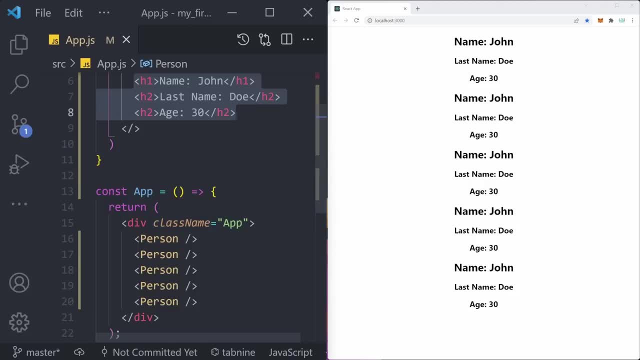 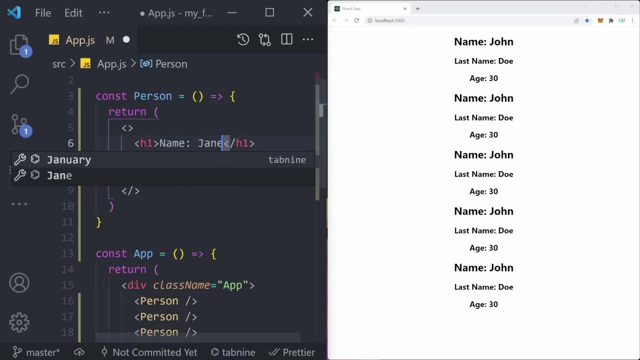 But now you might be wondering: why would we ever do this? This data is the same. How can we change this? Do we have to manually change everything? But then if we change something here, isn't it going to change in all of them? 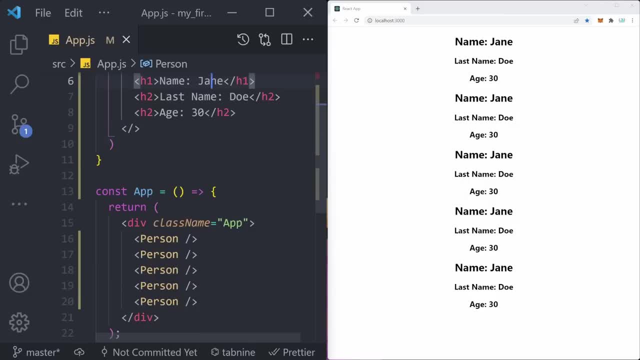 And that is true. But now we came to a really important part of React, And that is props. Props allow you to pass dynamic data through React components. Props are just arguments that you pass into React components. They are passed via attributes. They are just a shorter way of saying properties. 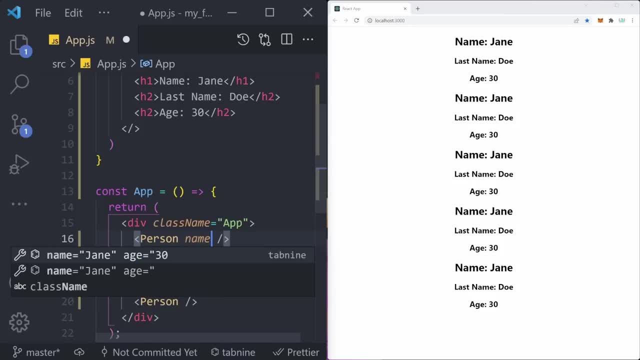 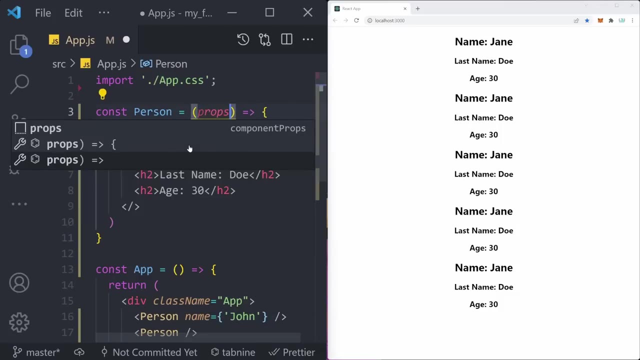 So in here, if we pass a name is equal to and we can pass a string of John, we can accept this prop inside of our person component. And how can we do that? Well, every component has a built-in props object And right here we can reference that props object by saying props. 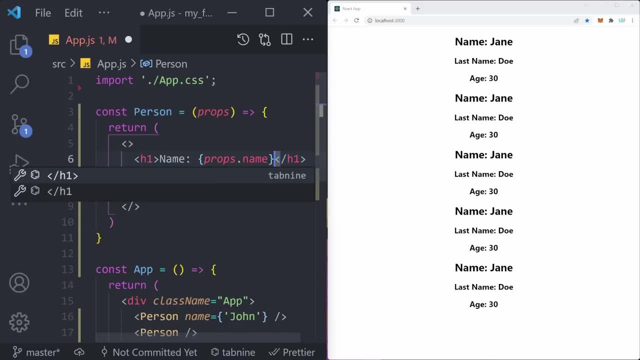 Props, dot and then name. So why did we do name here? Because that's how we call this: prop, Props, dot, name. Now, if we save this, you're going to notice that only the first component has our name and all the other ones are empty. 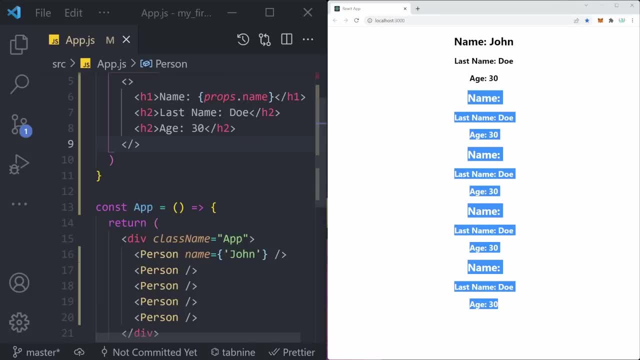 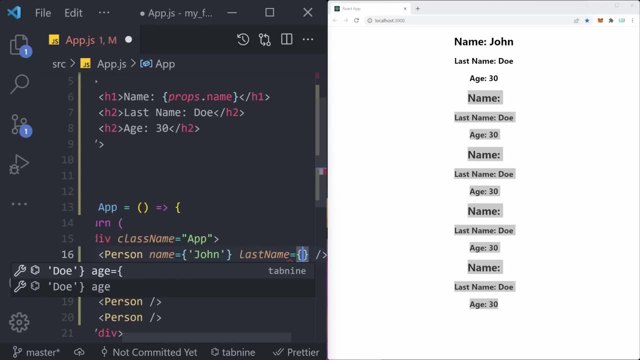 That's because we didn't pass a different name to any of our other components. What, of course, we can do is pass the last name as well. So let's say last name is equal to dough, And also let's do age is equal to 25.. 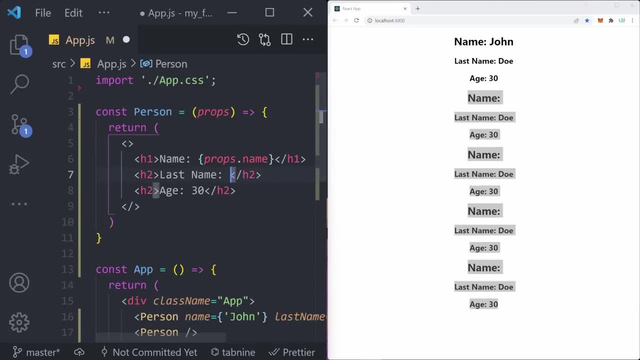 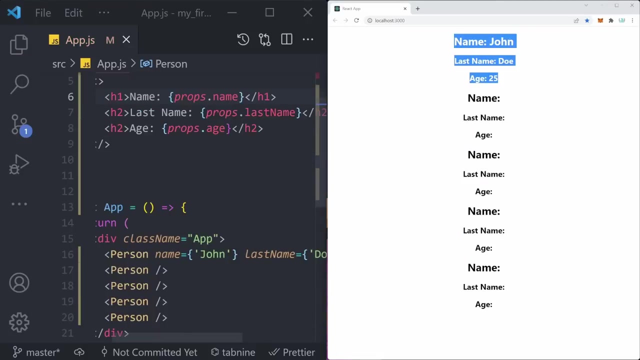 Now we can repeat the process. Last name is going to be props dot. last name- Notice how I'm putting this in curly braces- And then in here that's going to be props dot- age. And if we save that, you're going to notice that only our first component has all the data and the other ones are empty. 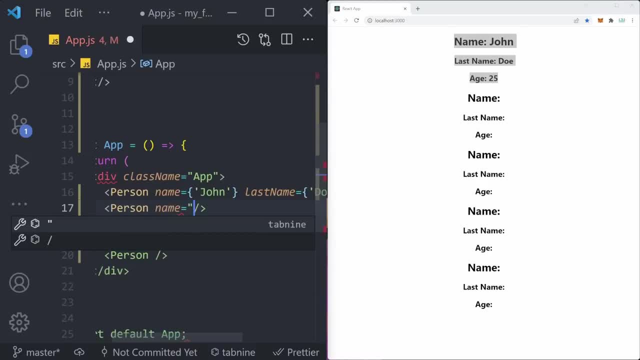 So now let's pass some other data Like name is equal to Jane. You can do it just like this without curly braces. if it's just a string, There we go. That works as well. But if you're passing some dynamic expressions like let's do, age is equal to 2 plus 2.. 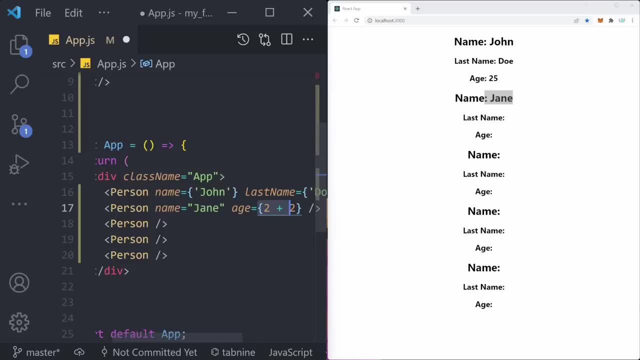 In that case you have to use curly braces, But in this case we were just fine with using normal strings And, as you can see, we can use both double and single quota strings. It doesn't matter. Now let's remove some of our people. 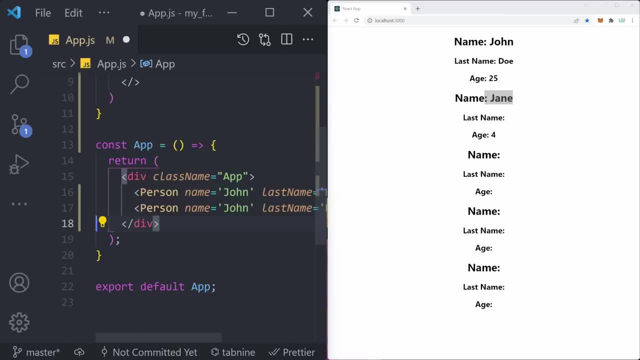 Let's copy our John person And let's just simply rename it to something like Mary Doe, And that's going to be 24.. And there we go. Now we have just two different people, And every single person is completely different when it comes to data. 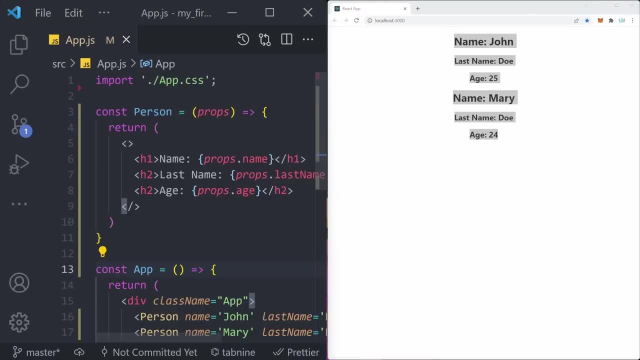 Now, of course, imagine if each one of these people is going to be an entire user profile. It would have much more than just three packs. It would have an image, all different kinds of properties, hobbies about sections, many more other things. 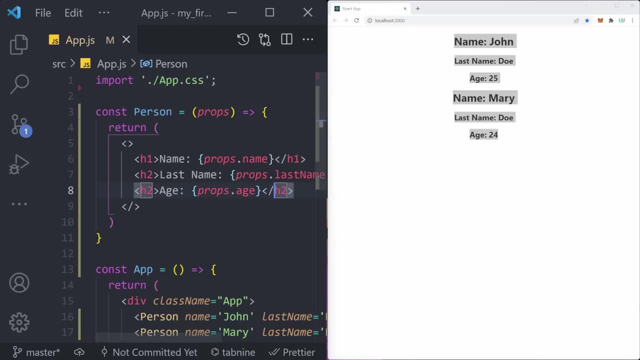 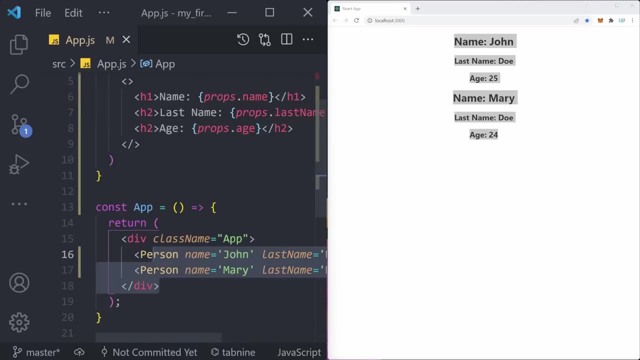 Many more other components and class names. So if that were the case and if we didn't use custom components, then we would have to copy and paste all of the JSX every single time. But if we put all of that code into a component, we can simply call it every time in a single line and pass new dynamic properties based on a different person. 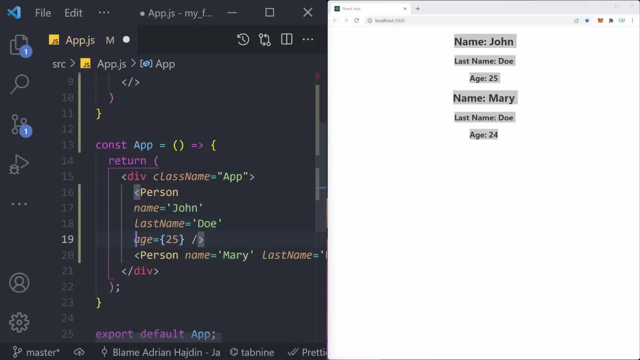 Of course, if you have a lot of properties, feel free to space them out in a new line like: so. That way it's going to be just a bit easier to read. There we go. Now that we've learned about props, let's learn about React state. 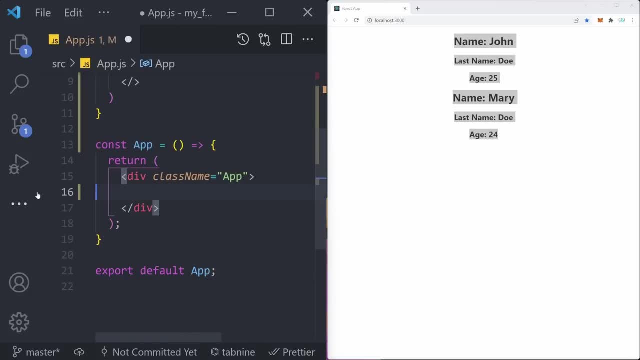 We can remove all of these people right here And also remove our custom component. State in React is a plain JavaScript object used by React to represent a piece of information about the component's current situation. It is completely managed. It is completely managed by the component itself. 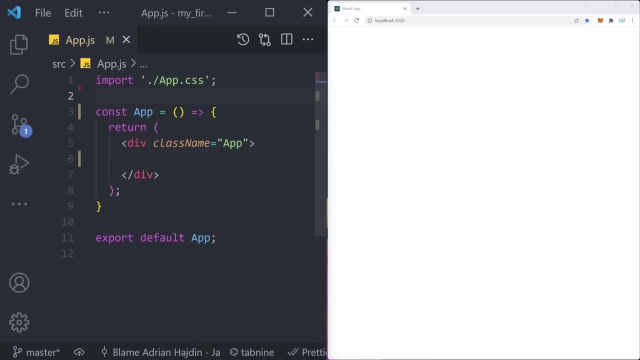 So how can we actually create state in React? First, we have to import in curly braces a so-called useState hook from React. This is going to allow us to use the state. of course, And before we actually call this useState, let me show you a scenario where you're really going to notice the purpose of state. 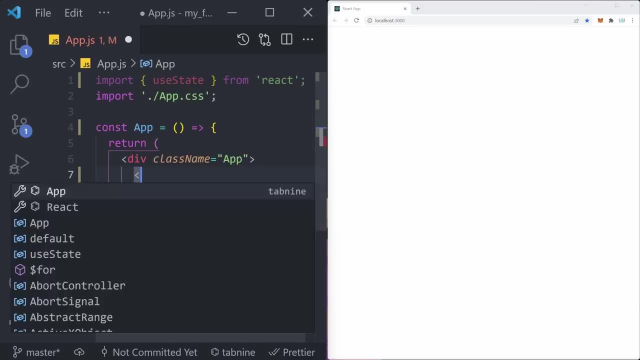 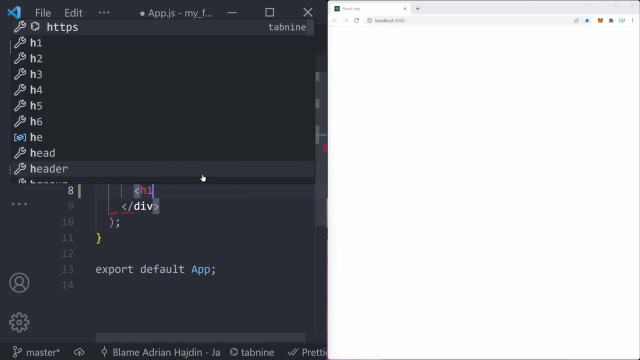 Let's create a counter. A counter is going to have two buttons: This one that's simply going to say minus. It's going to have some kind of an H1 in the middle that's going to show the count which is going to start at zero. 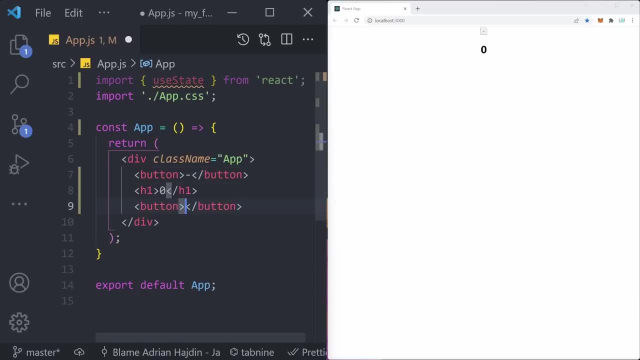 And then we're going to have one more button which is going to have a plus icon And it's going to increment that count. We can see that minus is on the top and plus is on the bottom Right now. if we click this, nothing is going to happen. 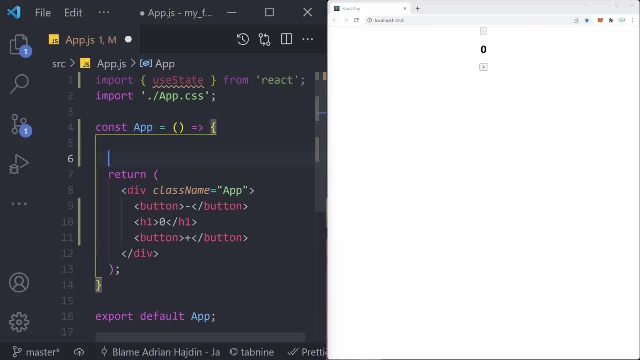 So we have to use state. Right here at the top of our component. we can say const and then use a concept of array destructuring. That is how state works. So we create a pair of square brackets, We say equal to and then call the useState as a function. 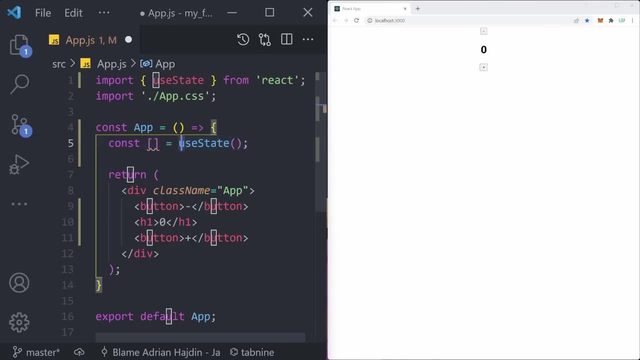 Whenever you call something as a function and it starts with use, in React we call that a hook. Now, the first part in the square brackets pair is going to be the name of that state, So let's call it counter. The second part is going to be a setter function and we can call it setCounter. 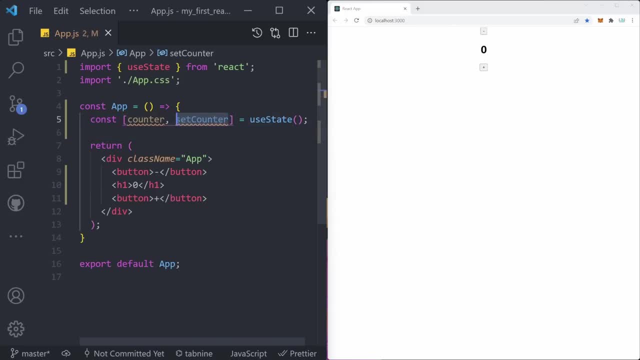 A good rule of thumb is that you call the second variable the same as you call the first one, but add the set in front, Because it is a setter function for the first variable. Now, inside of the useState, you provide the initial value, which is going to be zero. 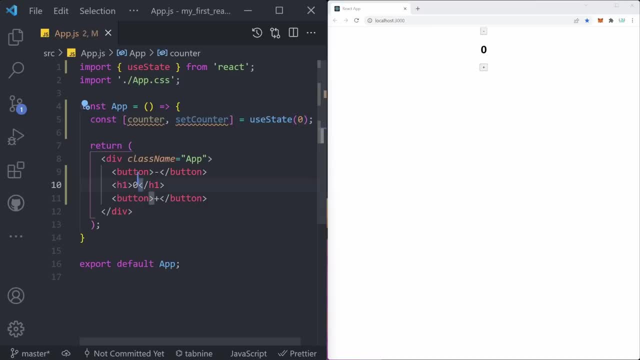 Now you can use this counter just as a normal JavaScript variable. Right here, let's reference it Counter And, as you can see, nothing changed. That's because the initial state is still zero. So now we're going to learn about events. 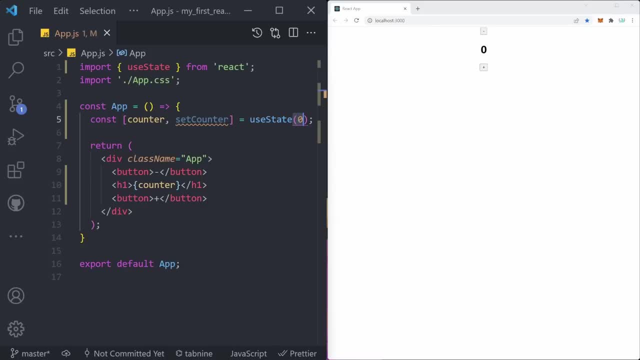 An event is an action that can be triggered as a result of the user action or some kind of a system generated event. For example, a mouse click or a button press is an event, And here is how we can handle events. in React On this button, you can add an onClick property written like this: 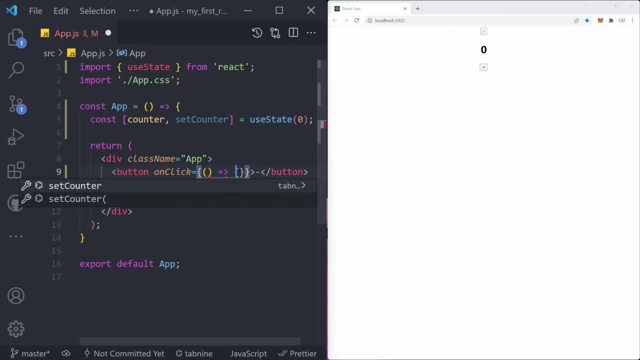 There we're going to have a callback function. A callback function is the one that simply doesn't have a name. it's here and it's just waiting for some kind of a command. Right here we can write an inline code by simply saying: alert clicked. 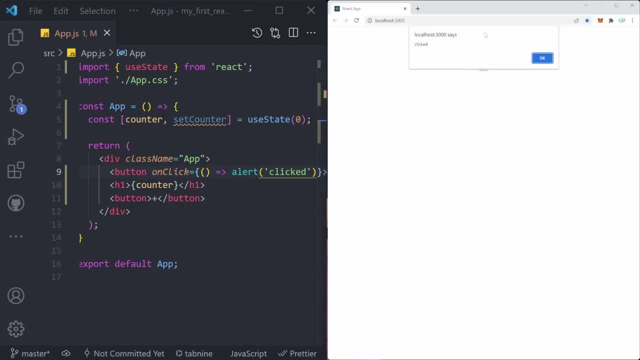 If we save this, you can see that if we click on a minus button, we're going to get an alert that says clicked. That means that we've read the event properly. But now on the click, we don't simply want to alert something. 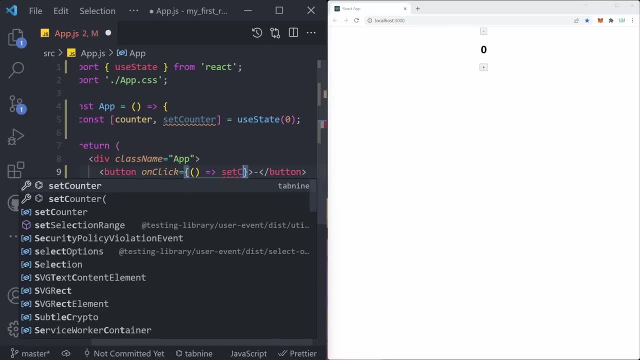 We want to change the state. For that we're going to use the setter function, Set counter. What we can do is we can set it to something like minus five or any other value, And if we now click this, you can see it gets reset dynamically. 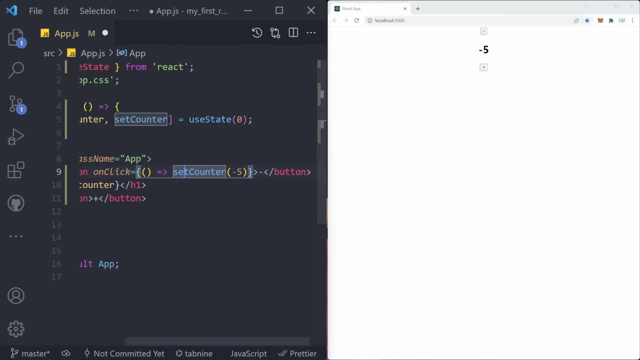 The code changes. Now how can we lower the count by one each time that we press a button? Well, inside of the set counter, we're going to create a callback function, And right here we have access to something known as a prev count. 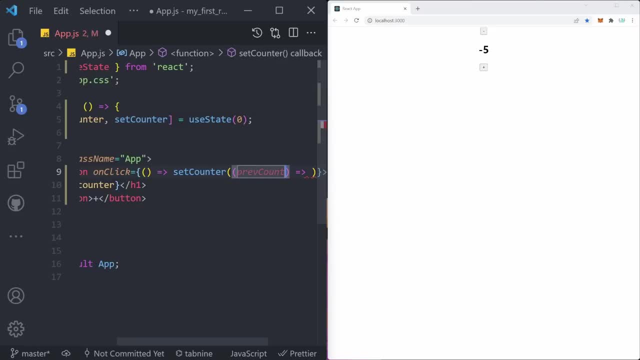 This is just a parameter of the set state. You can call it however you want, but a good practice is to call it prev, as in previous, and then the name of your state, And what we can do is simply call the prev count and decrement it by one. 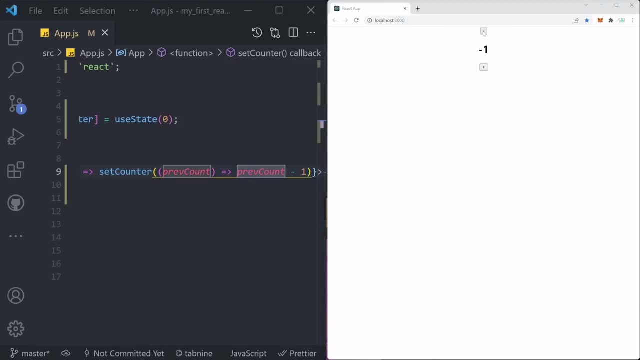 Now, if we save this and reload the page, as you can see, we can keep clicking the button and the count changes. We can duplicate this line, paste it below our counter and in here the only thing we have to change. 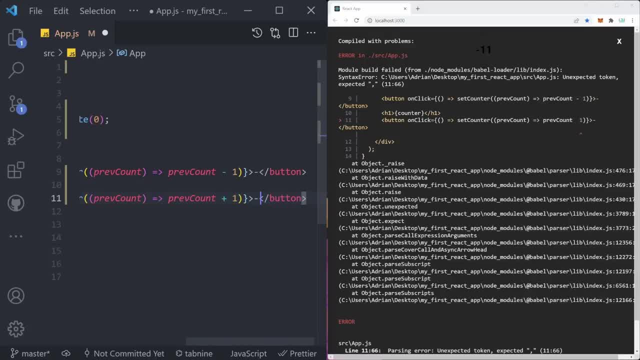 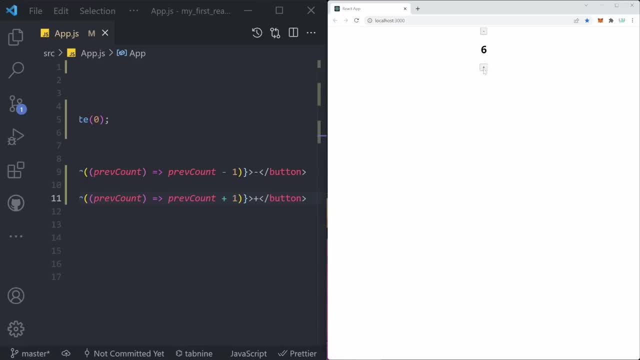 is to add a plus right here as well as right here. Now we can increment our counter as well, And I know this is a small application, but it's dynamic. You're clicking on it and you're changing the state. 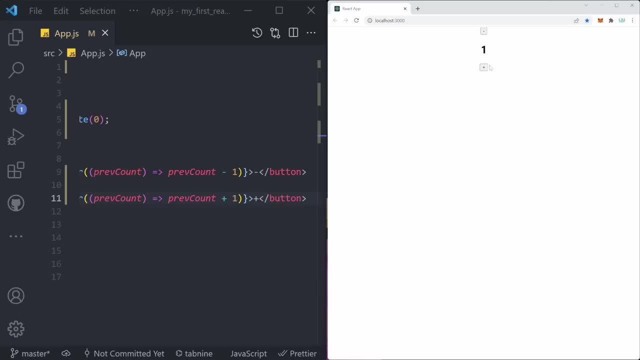 and therefore re-rendering the view Again. a really important thing is that all of this is happening without a website reload. If you keep tracking this, keep looking at this reload button. When I reload it's going to change, But now, if I keep clicking, 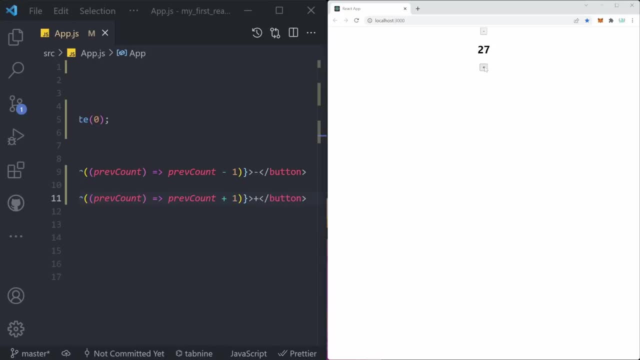 it remains the same, which means that the website is changing without a reload. And you might think, of course, this is a simple application, nothing has to reload here, And you would be right if you think that. But imagine all of the complex websites. 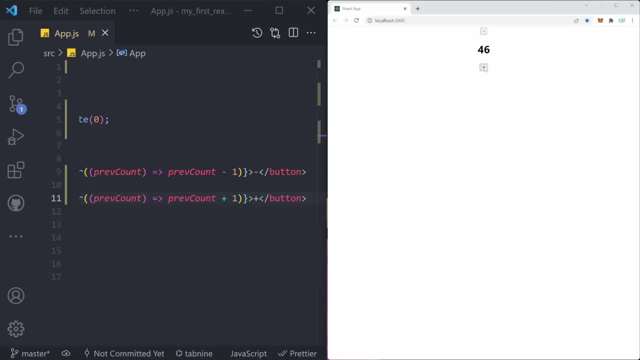 that have tons of functionality, a lot of moving pieces and everything else. The situation is going to be the same. If you're using React, then you can update everything on the page without needing a page reload. That is amazing. When we started talking about state, 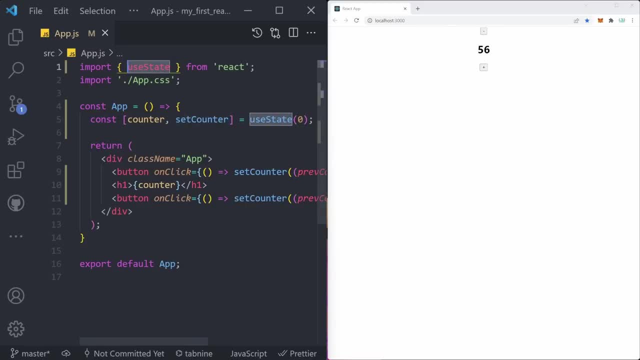 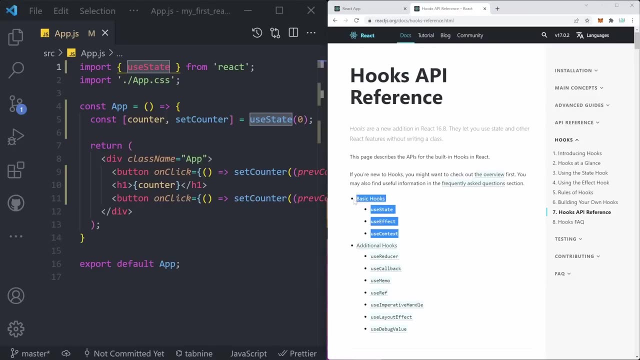 we immediately mentioned hooks, because we cannot use the state without using this React hook, And there are many other hooks. As you can see, we have the three basic hooks, as well as some of the additional hooks. By the way, I'm looking at this. 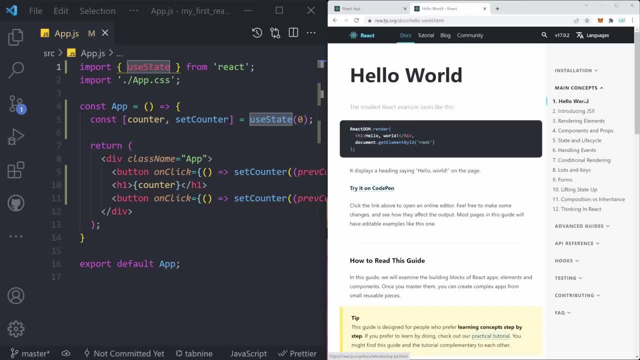 in the official React documentation. I would strongly encourage you to go through their docs, at least through the main concepts from the hello world all the way to thinking in React. Their documentation is phenomenal. Definitely make sure to go through it as the practice. after watching this video. 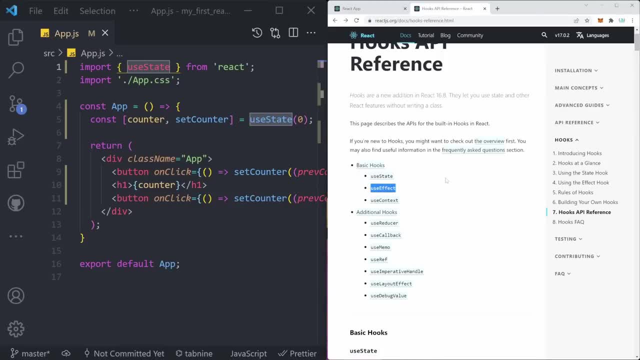 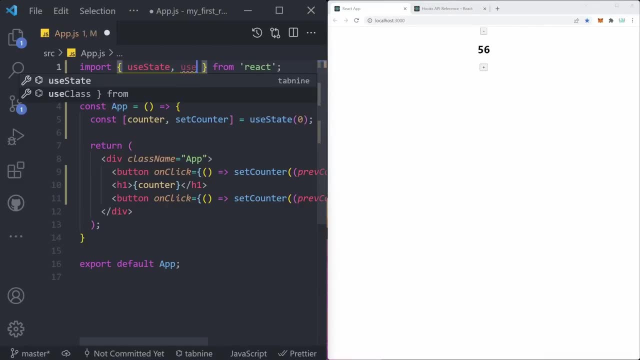 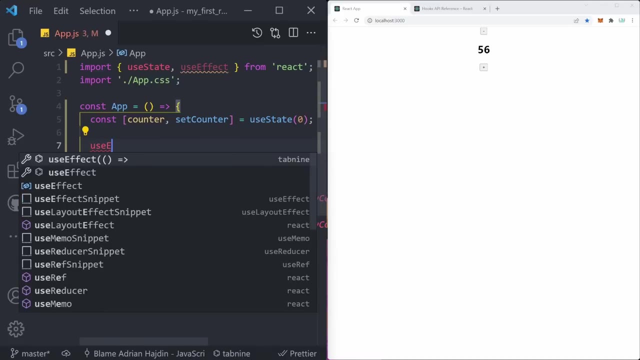 So, with that said, let me also show you the second most used React hook, which is useEffect. We can simply import it at the top, as we imported the first one- useEffect- and it's going to get called a bit differently. We type useEffect right here. 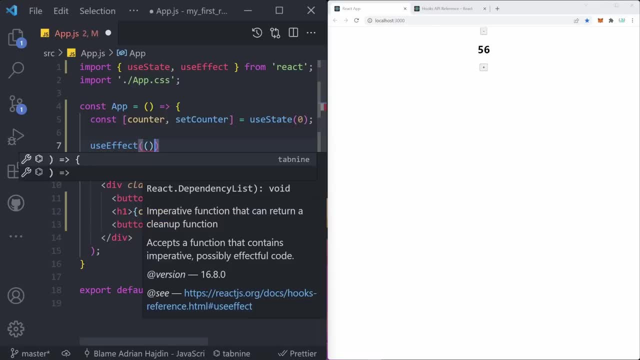 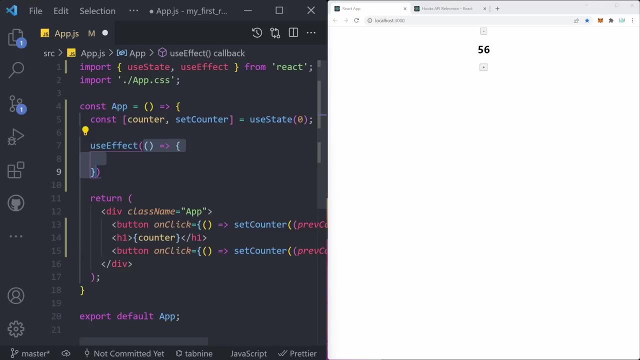 call it as a function and then it accepts one more function as the first parameter, Again a callback function. You can see that we're using a lot of ES6 syntax Array, destructuring, import syntax, arrow functions and more. 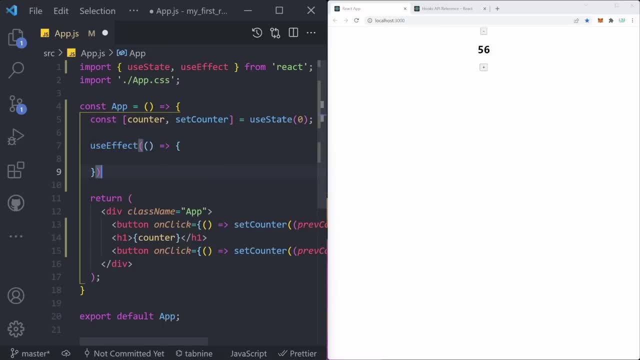 So I would strongly encourage you to get comfortable with JavaScript ES6 Plus before you dive into React. useEffect allows us to do something on some kind of an effect or, let's say, on some kind of an event. So this code right here is going to get run. 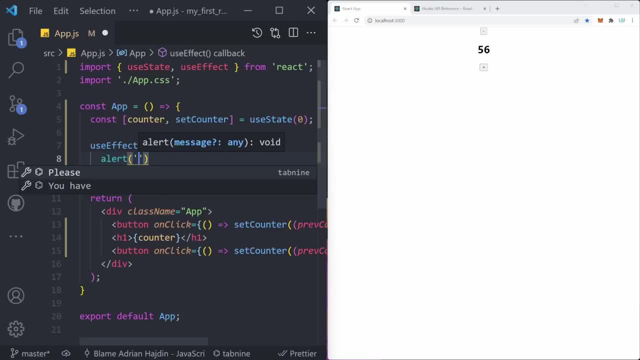 as soon as the page loads. So let's say reload. There we go, I saved it And I get an alert that says reload. If I reload the page one more time, it's going to happen again, because this code happens as soon as this component renders. 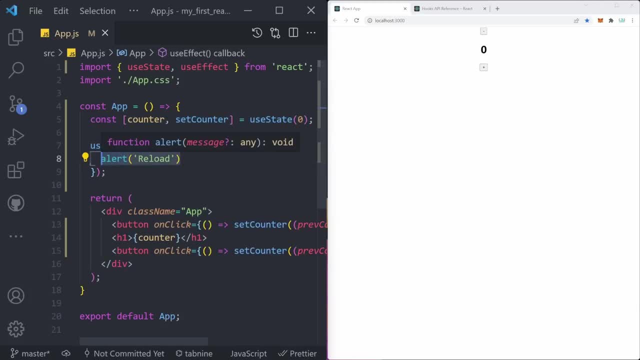 So, using this useEffect and knowing that this is going to happen at the start, how would you change our counter? our state to be 100 as soon as the page loads, If you wanted to do something like this? counter is equal to 100. 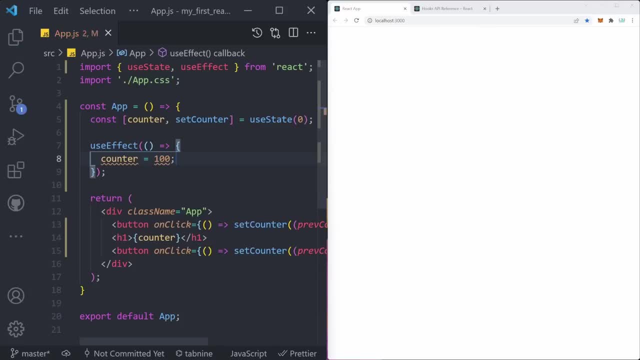 That's going to cause a major issue. We cannot see an error yet, but that's because we're breaking the most important rule of React, And that is: never modify state manually, Never mutate. the state Counter is not just a normal variable. 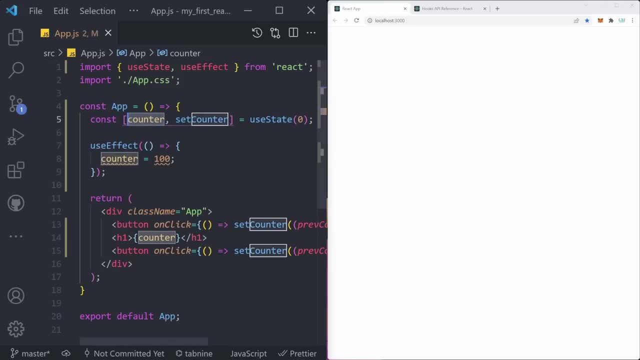 It is a part of the React state, And React state can only be changed using its own setter function. So this here is strictly forbidden And, as you can see, the app doesn't work. So let's simply call a set counter And this is how you would set. 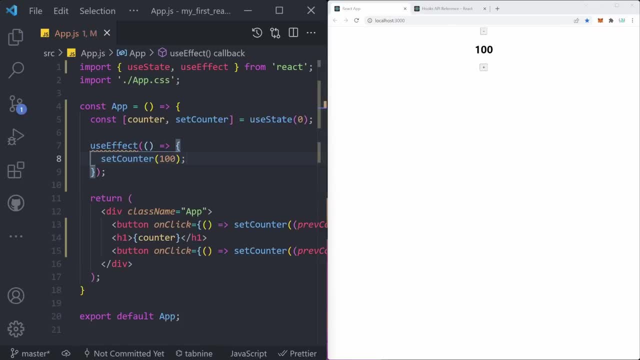 the counter to 100.. As you can see, it is 100 initially and now we can modify it. But something happens. We cannot really modify it. It seems that this useEffect is happening too often And as soon as we click it. 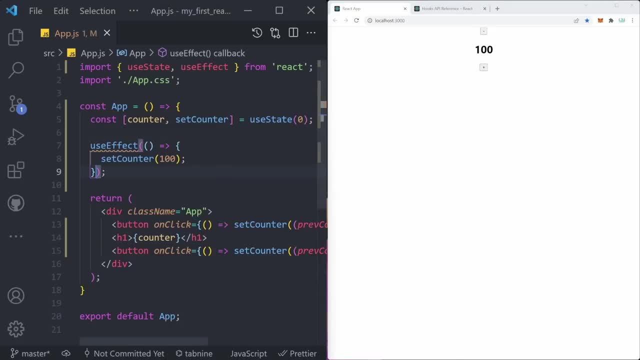 it brings it back to 100.. So there is the second parameter to the useEffect, which is called a dependency array. If we now save this, we've just left our dependency array to be empty. So now, if we modify this, we can clearly do that. 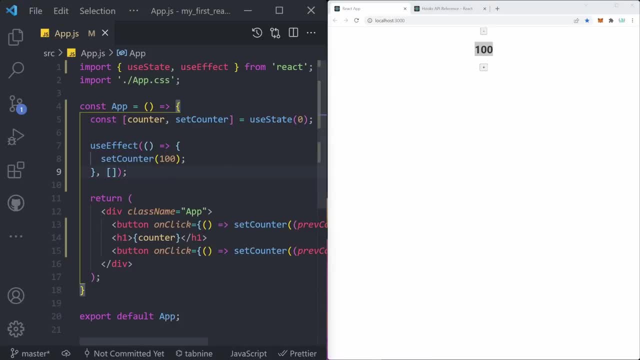 The value only gets set at the start. That is because when the dependency array is empty, the code inside of here, more specifically inside this function, is going to only happen at the initial load of the component. But if we add some kind of a variable here, 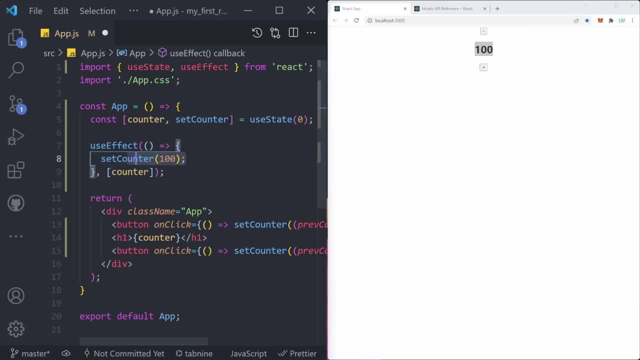 like a counter, then this code is going to update every time that the variable inside of this array changes. We would got into an infinite loop if I tried running this. That is because if I initially set the counter to something and then I keep changing it, 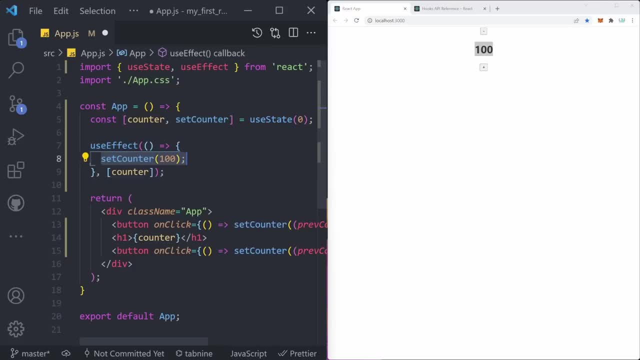 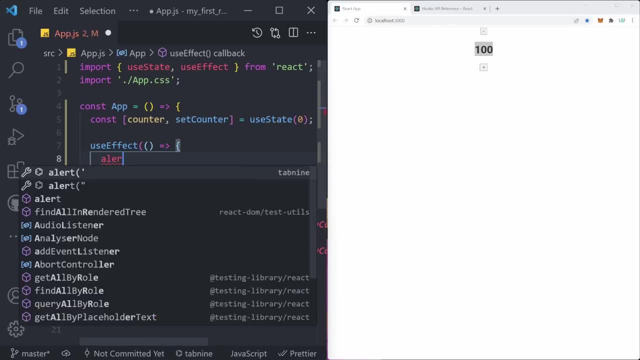 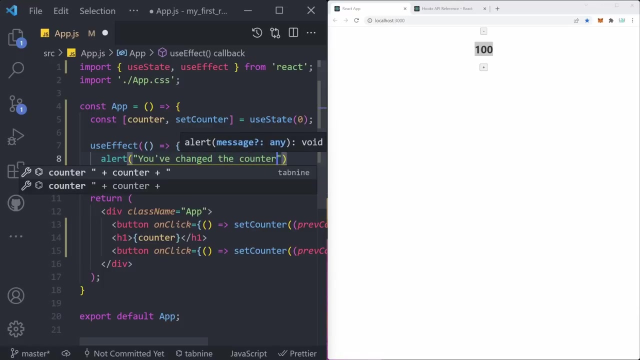 it's going to continuously run because this function is changing the counter, and then the counter recalls it. That is not a good practice, So what we can do is simply alert something whenever the counter changes. Let's say, you've changed the counter to. 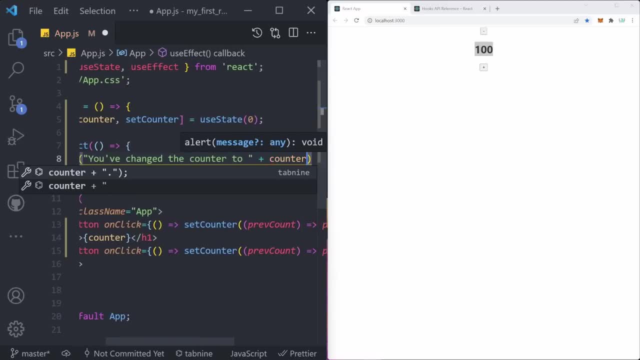 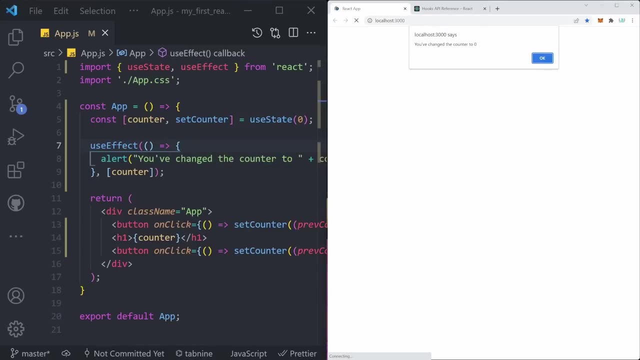 and then let's simply say: counter: There we go Now, if we save this, you've changed the counter to 100.. Let's reload the page. You've changed the counter to zero, You've changed the counter to one, two and so on. 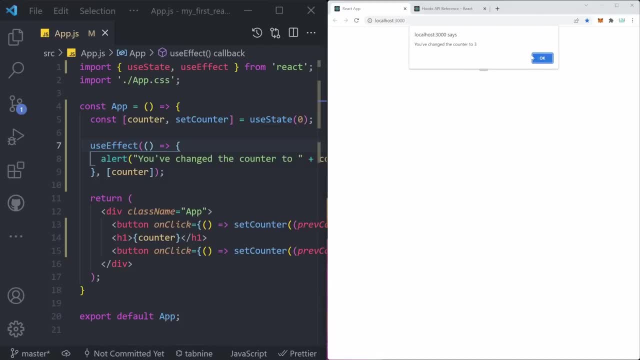 This is not a good user experience, definitely, But the only thing I wanted to show you here is that you can call some code whenever something happens in your React application by simply providing that variable here, and whenever that variable changes, then you can call the code. 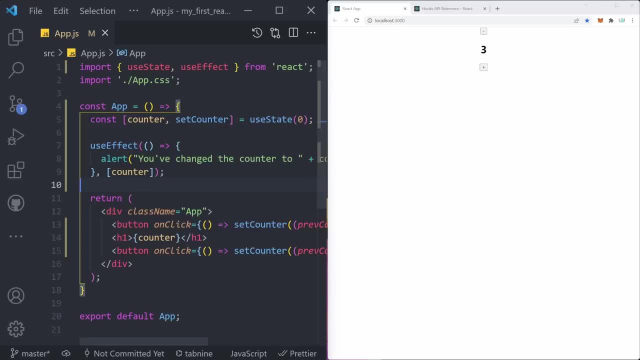 inside of the useEffect. With that we've learned the three most important things that React offers, and that is components, state and props. Of course, alongside that, we also learned hooks, specifically the useState and the useEffect hook, And we also talked about events. 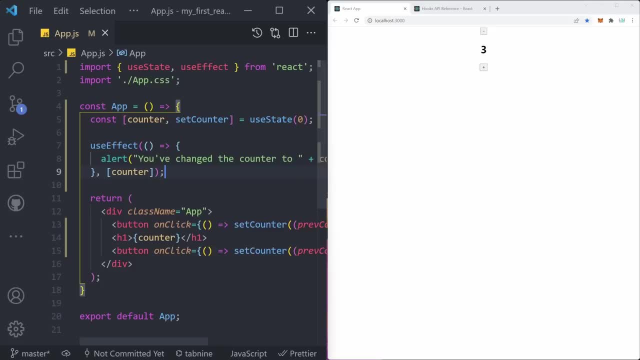 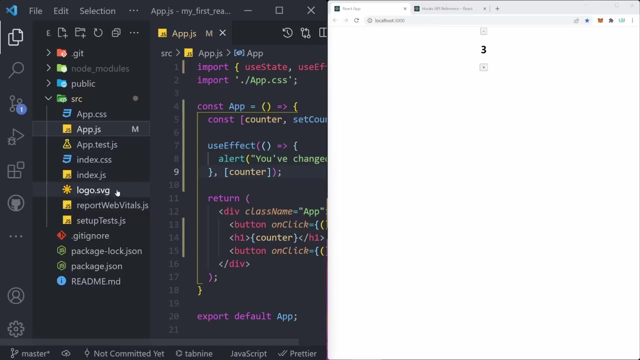 more specifically, the onClick event. I'm pretty sure that you're ready to build your real ReactJS project right now, So what we can do is open up our file tree by clicking here and we can completely delete the source code, because we don't need many of these files right here. 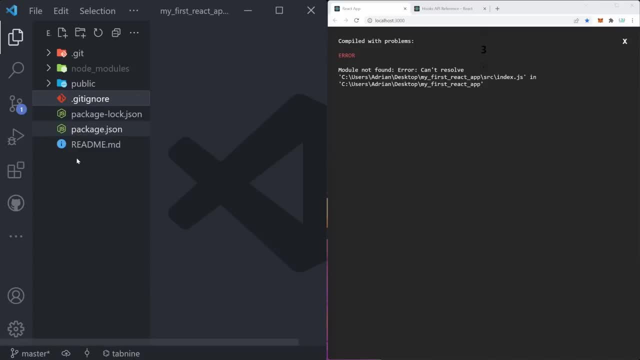 So let's go ahead and right-click, click, Delete, press right-click right here and create a new folder called src. Now let's test your knowledge. What does every source component needs to have? What is one file that absolutely needs to be there? 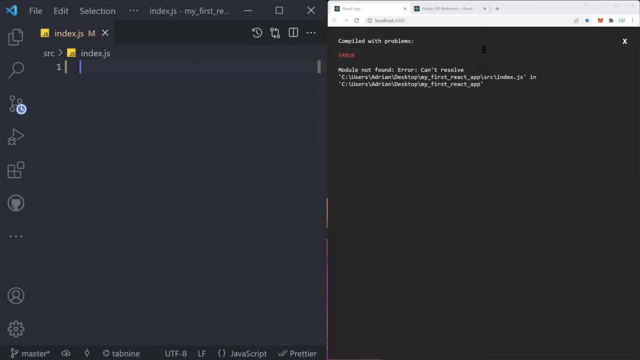 That is going to be indexjs. Inside of there we import React from React as well as import React DOM from React-DOM. Then we can say: import app and that app is coming from slash app. Of course we haven't yet created this. 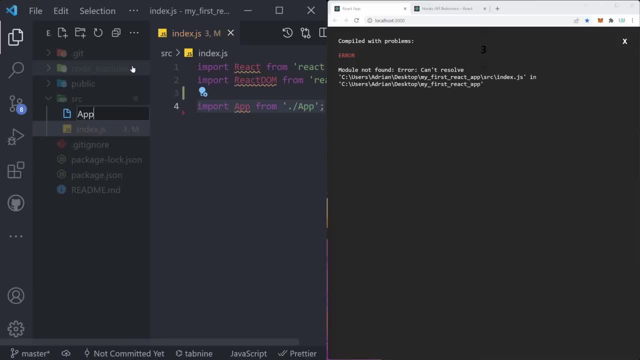 so let's go ahead and create a new file which is going to be called appjs. Inside of there, we can import React. from React We can create our app, which is the main functional component. that looks like this: Our app is going to have: 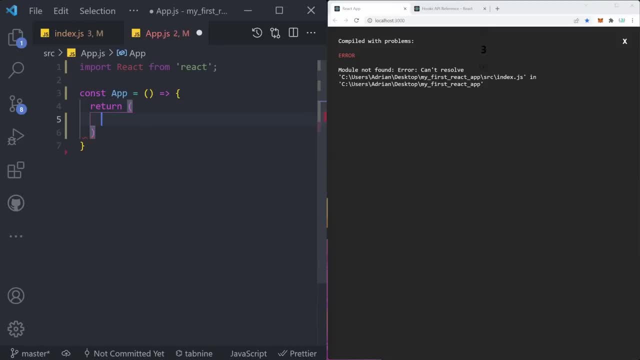 a return statement and then inside of that return, for now we can simply return an h1. that's going to say app. Let's add a semicolon here and of course, let's do export default app. We have to export every single one. 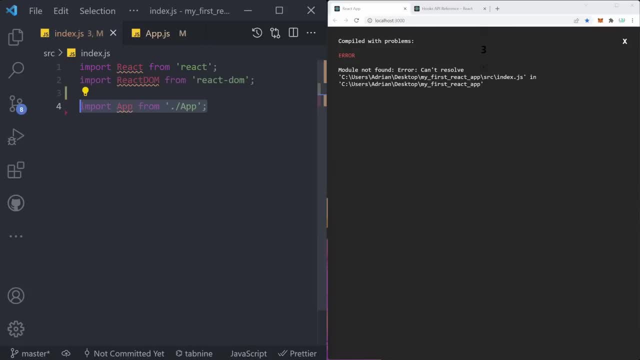 of our components so that we can then call it from somewhere else. In this case, we're importing it inside of our indexjs file, And inside of our indexjs, as we learned before, we have to do react-domrender and then we have to pass in the component. 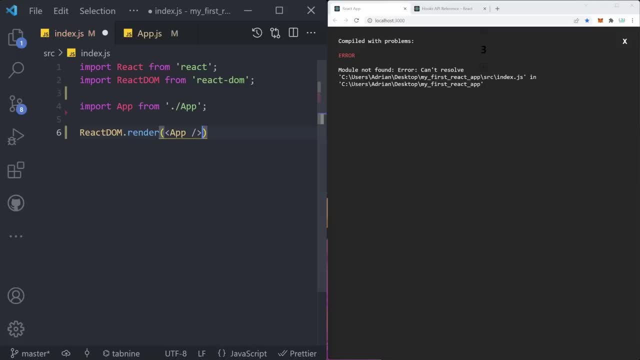 we want to render, which is, in this case, the app component, And then we have to trigger documentgetElementById and then pass a string of root. This is going to trigger our div with an id of root and it's going to inject. 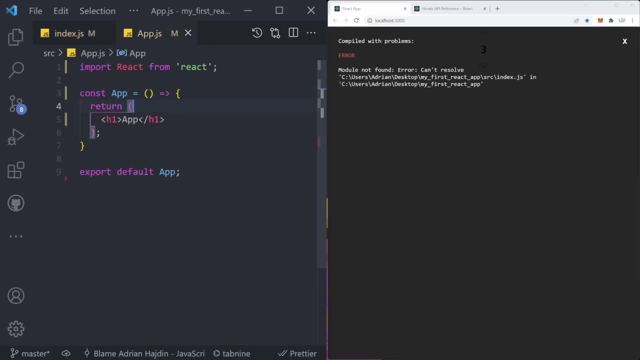 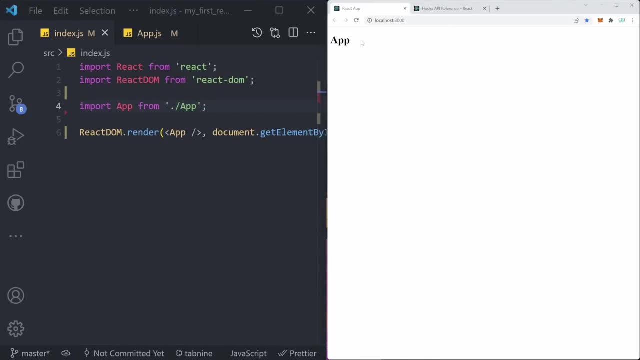 our entire React application right inside of it. And finally, if you reload the page you should be able to see app right here. Sometimes React messes up a bit when you delete the entire source folder, so you might need to go to view. 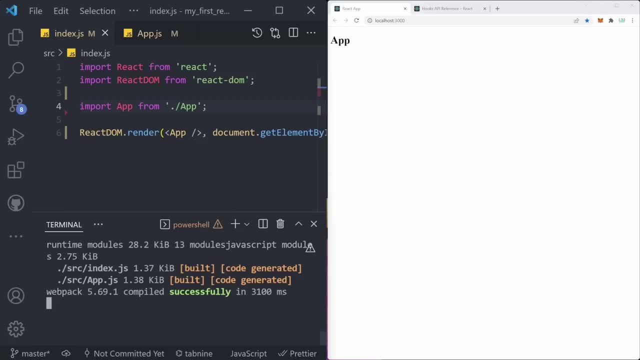 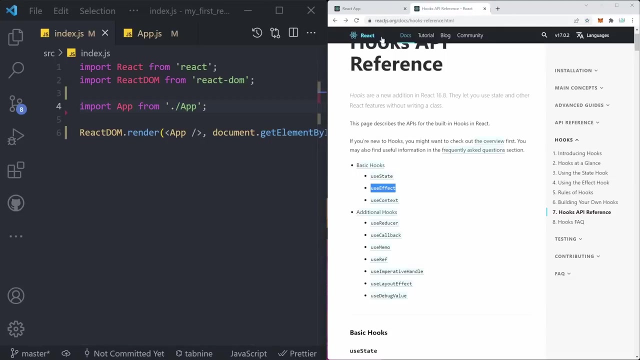 and then terminal, and then press control C and then Y, like this, And then just restart application by running the npm start command Whenever you want to restart it or close it. control C and then Y. There we go With that said. 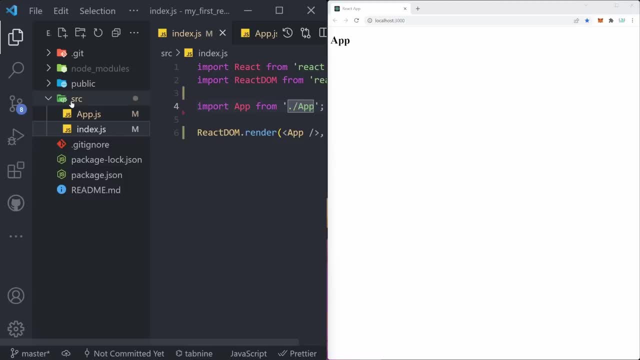 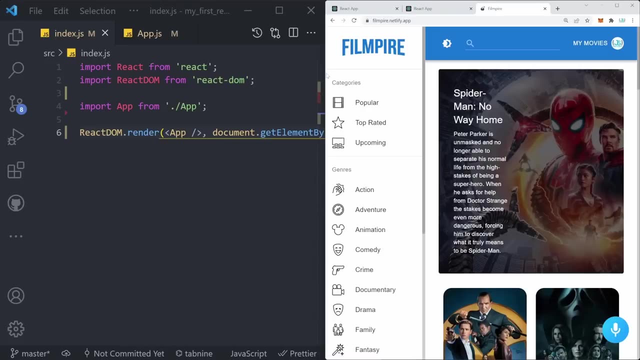 now we have an empty working environment, just the source with the app and indexjs, and we are ready to create our application. Believe it or not, in this video you're going to build a simplified version of the FilmPyre project. 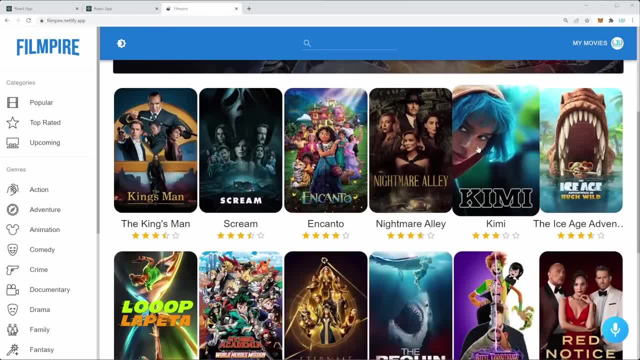 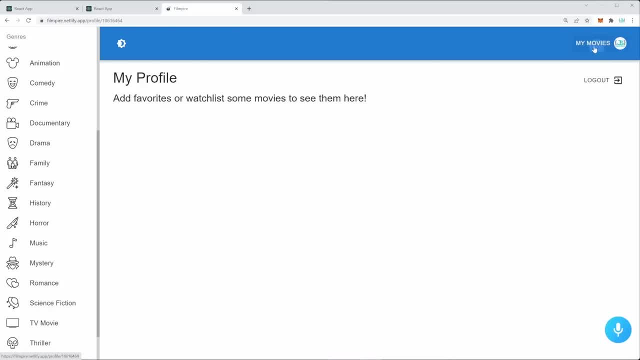 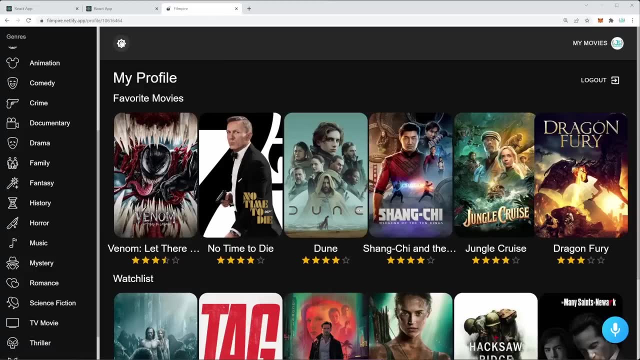 So this is the FilmPyre project. It has nice animations, a central card, all of the different categories, movie details, information, animations and even voice, artificial intelligence. Of course, dark mode is there as well, But we're going to build this. 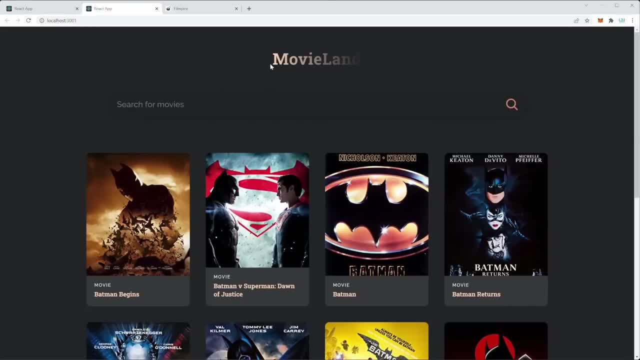 which is a simplified version of the FilmPyre application called Movieland. There you get access to all of the movies that you search for. In here we have Batman. Let's try to go with something like Shrek. That should be good. 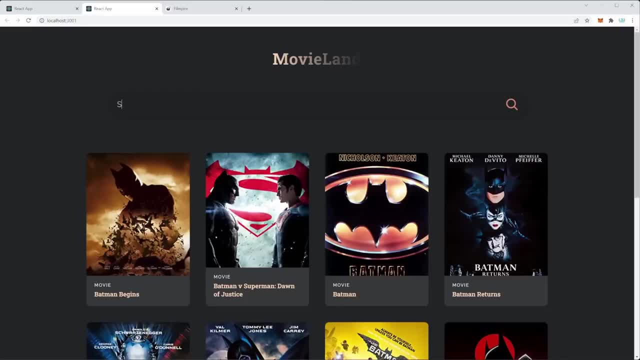 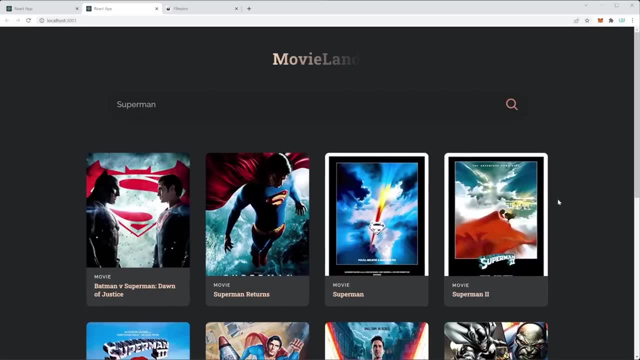 There we go- Let's try to go with something like Superman as well- And just click Search And you immediately get all of the latest Superman movies and you can scroll through them. Of course, the application is fully mobile responsive, So if you right-click, 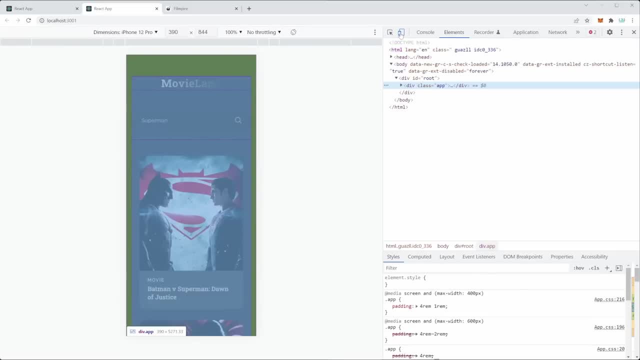 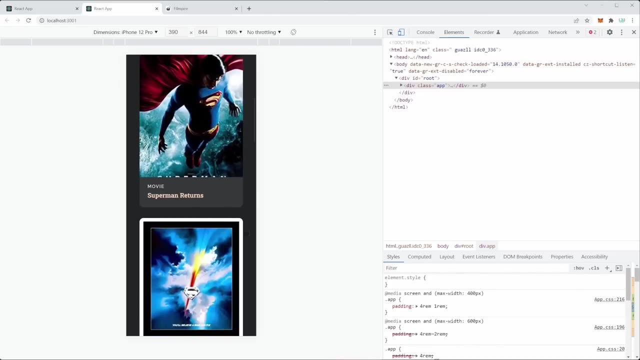 click Inspect and then click this little icon right here that's going to toggle the device toolbar and you can see that your application is fully mobile responsive. So what do you say? Let's go ahead and get started with implementing everything you've learned so far. 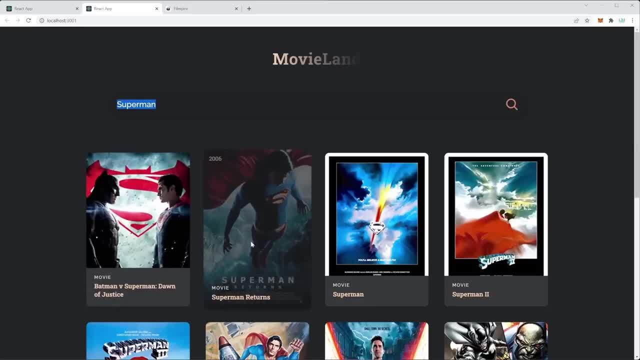 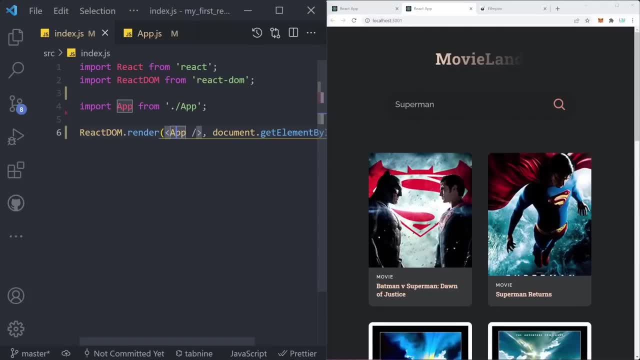 Managing state using different components, props and so much more. Let's pull our browser on the side and let's get started by going into our appjs. I'm going to keep this website open, just for reference When it comes to FilmPyre. 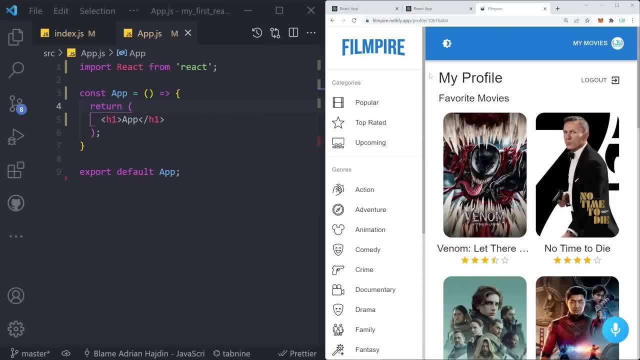 we can close that tab. By the way, if you're interested in learning React to extremely advanced levels while building this website, this great application, definitely make sure to click the link in the description: join our newsletter to be the first one to get into the course. 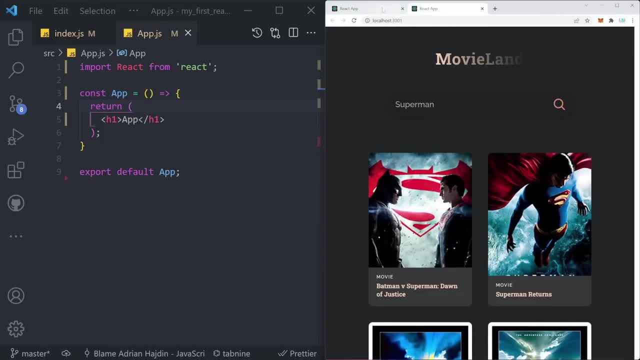 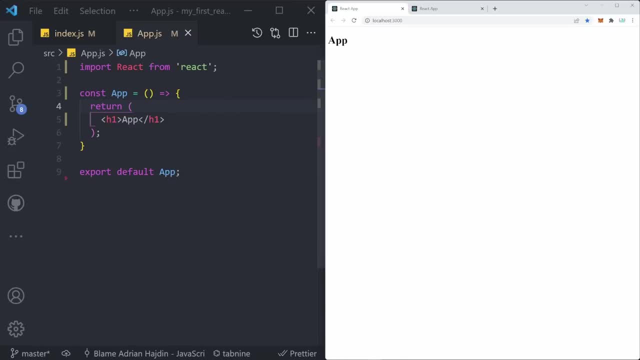 With that said, we can now close this and start transforming our app into movie land Alongside, using state hooks and so much more, we're going to also use an external API, an application programming interface that is going to give us access to data about these movies. 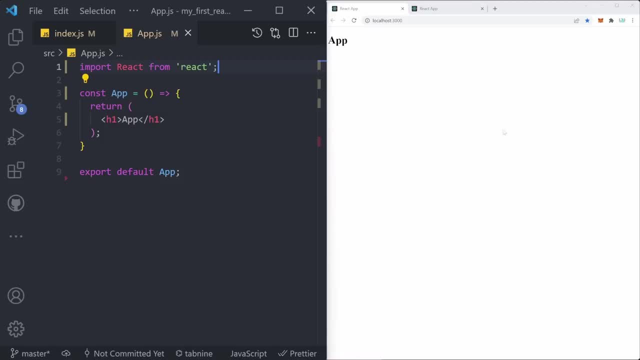 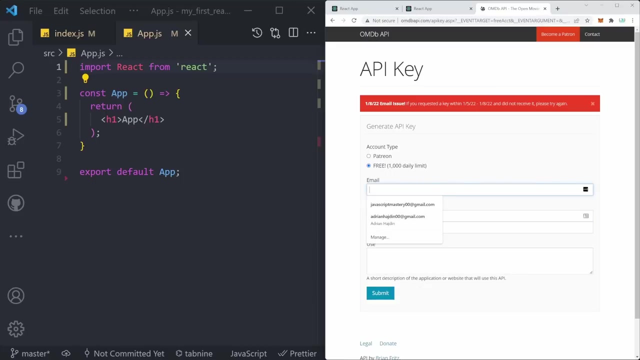 So that might be a good starting point. You can head to omdbapicom forward slash API key. The link is going to be down in the description. Then you can choose your account type as free and enter your email. I'm going to do JavaScript Mastery. 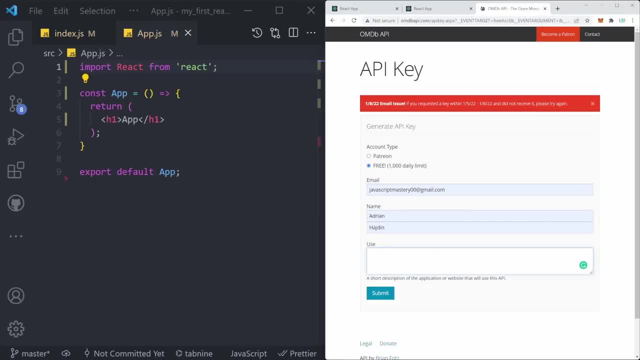 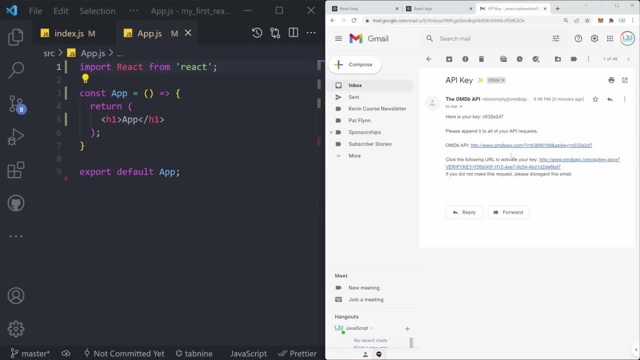 enter my email right here and you can type: use building a movie app and click submit. In a few seconds you're going to receive a verification link to activate your key to your email address. Once you get the email, you'll have to activate your key. 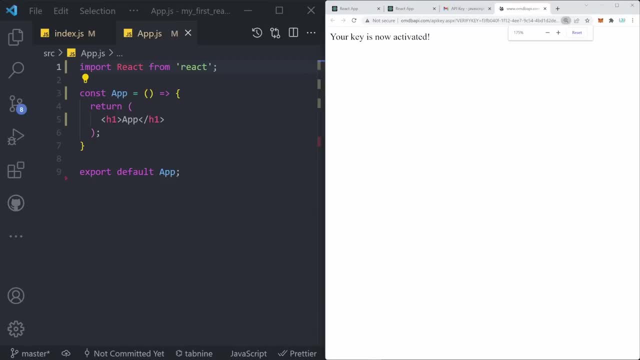 by clicking right here, You're going to see a message that says your key is now activated, And then you can go back to your email and copy your API key and paste it as a comment right here, because we're definitely going to use it later on. 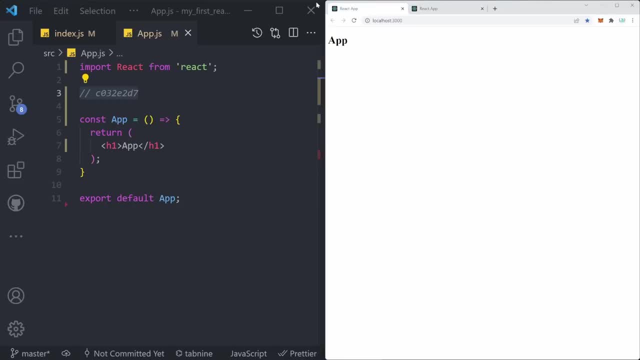 Now we can close this, close this as well and go back to our application. So let's explore the ways in which we can call this API to get all the data about movies. We're going to create a static variable called API underscore URL. 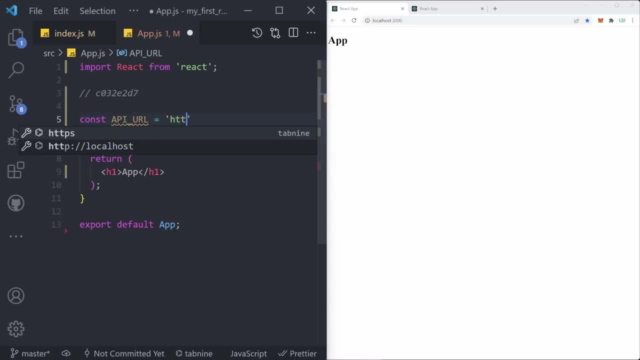 And that's going to be a string that's equal to: http//wwwomdbapicom. API key is equal to: and then you can simply copy your key and paste it here. That's going to be our API URL. Now we can use that. 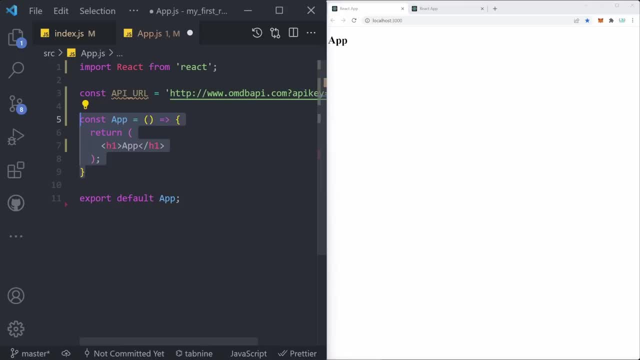 from inside of our component to gather the data. More specifically, we want to fetch the data from this API as soon as our component loads. Do you know which hook can we use for that? It's going to be the use effect hook. So right here. 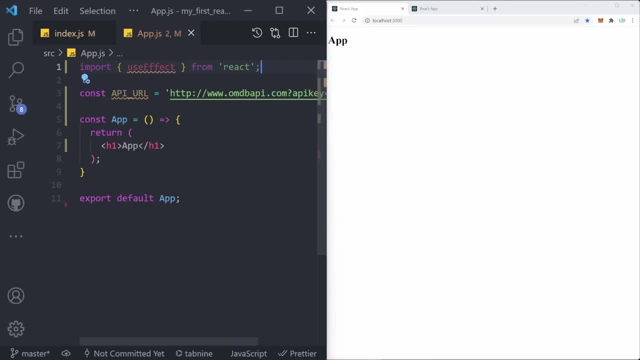 we can import the use effect hook from React. Let's call it as we learned: use effect accepts a callback function and an empty dependency array as the second one, if we only want to call it at the start, Now inside of there. 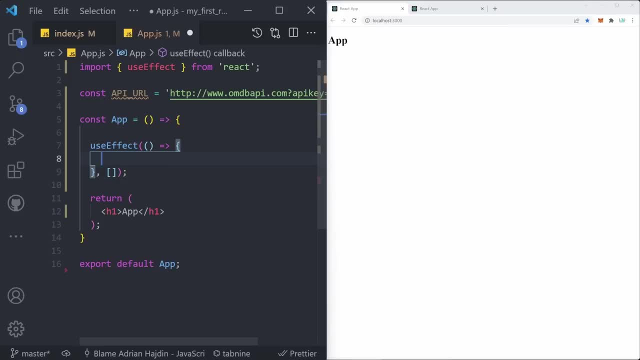 we're going to call a function that's going to fetch our movies. So just at the top of our use effect, let's create a new function. const search movies is equal to an async arrow function. Async stands for asynchronous data. 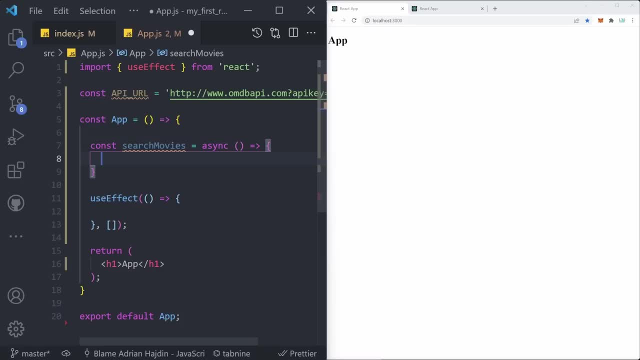 which means that it takes some time to fetch these movies And the search movies is going to accept a search title that we want to search by, like Superman or any other title. There we can say: const response is equal to await fetch. 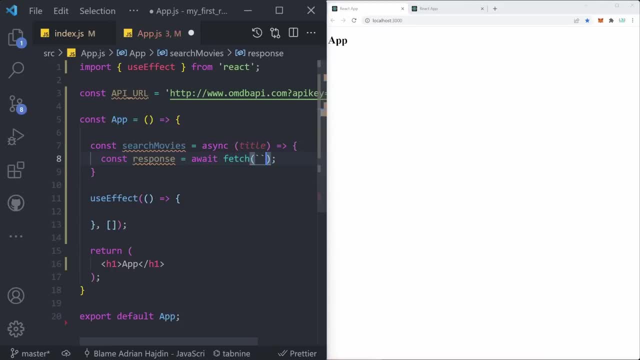 And then in here we can use a template string. You can do that by using the backticks On my keyboard. it is a key left to the one key. There we can dynamically specify the API URL. So API underscore URL. 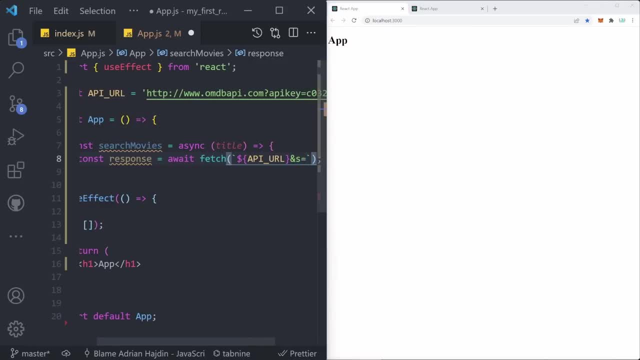 And then say: and s is equal to. And then one more time in here we want to specify the title. So this is going to call our API. Now, once we get the response, we have to get the data from it. 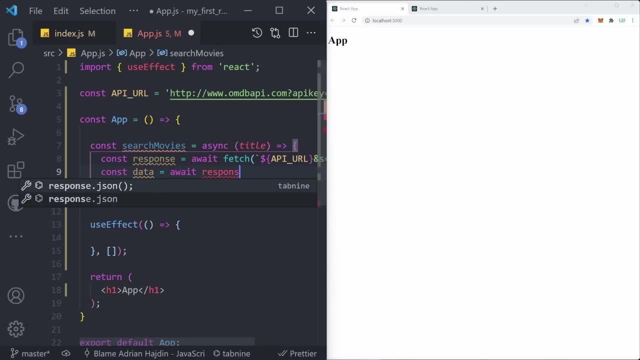 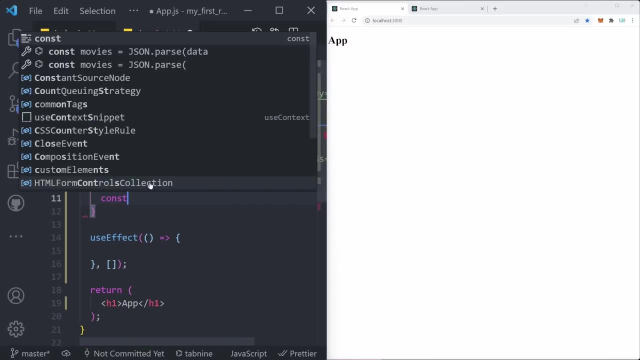 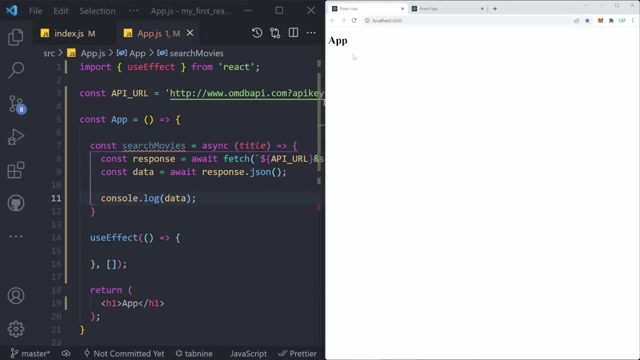 by saying const data is equal to await response dot json. Now inside of this data object we should have the data about the movies. So let's simply console log it for now. console log data. We can open up our console. 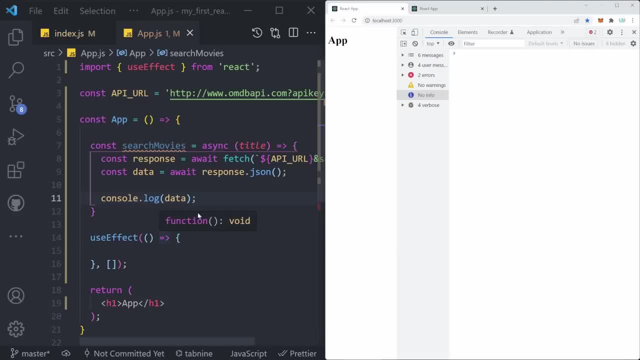 go to inspect and console. Right here, nothing is happening because, as you can see, we're never calling our search movies. So what we can do is simply call it inside of our use effect, And let's also provide it a title. 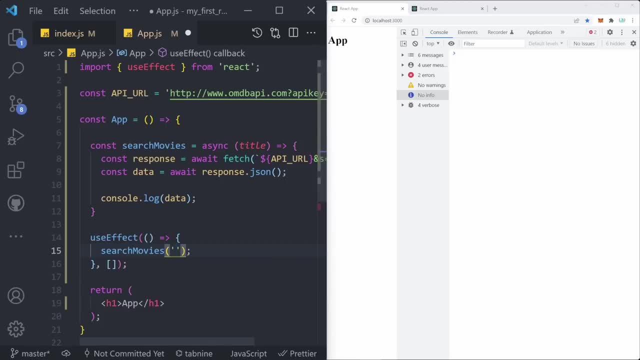 which is going to be a string of your favorite movie. Feel free to put any title in there. In this case, I'm going to go with Spider-Man and save it. As soon as we save the file, we're going to notice that we get back the search. 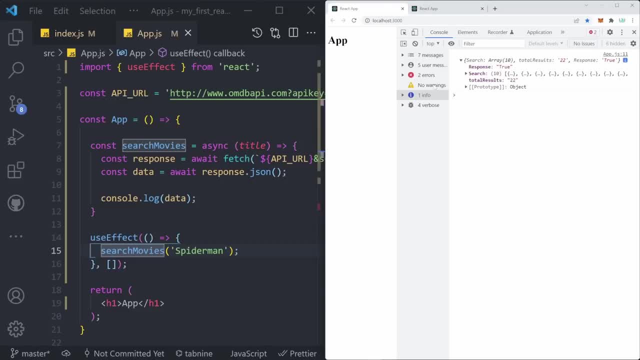 the response and total results. We only need the movies array so we can console, log, data, dot search, And now we get only an array with 10 Superman movies. That's great. That means that the API fully works. But now 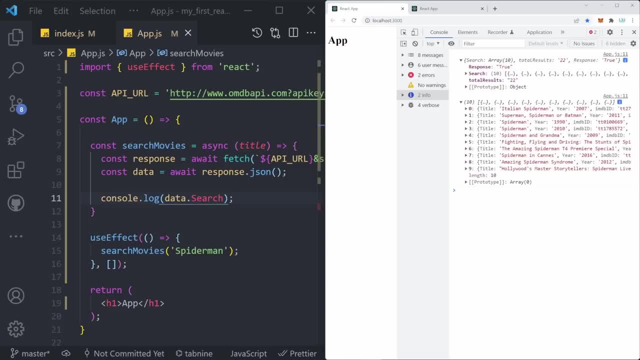 we need to be able to render that data and show it inside of our application. To make your life easier, I'm going to provide you with the entire CSS file for this entire application. Today's focus is to learn React, And you're going to do that with this project. 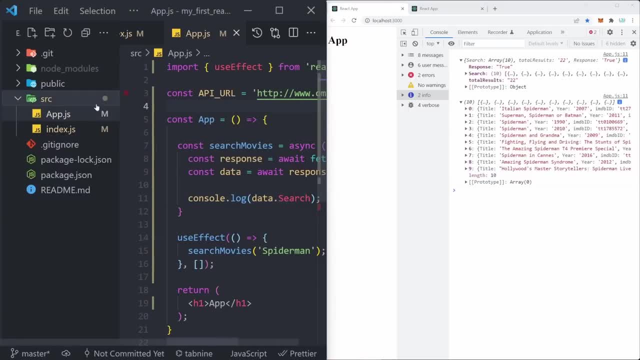 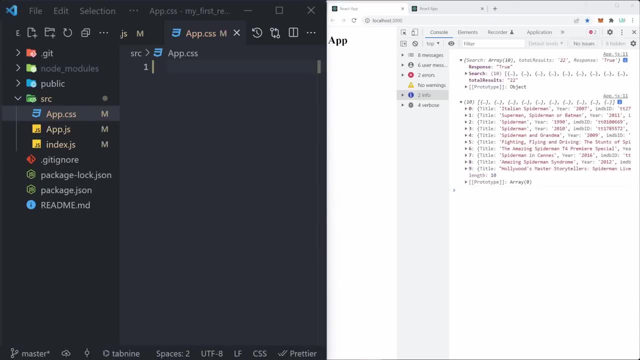 but you don't have to manually write every CSS line, So what you can do is create a new file called appcss, And then, in the link below this video, there's going to be a GitHub gist containing the code for the entire appcss. 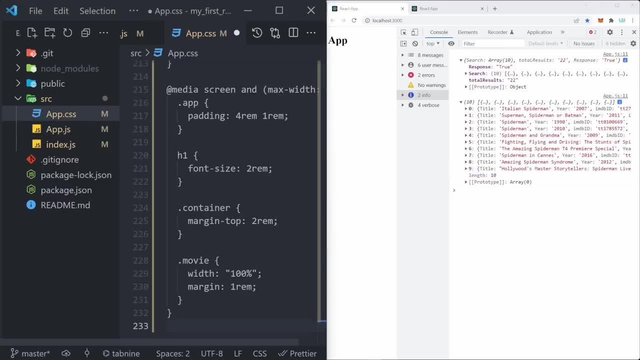 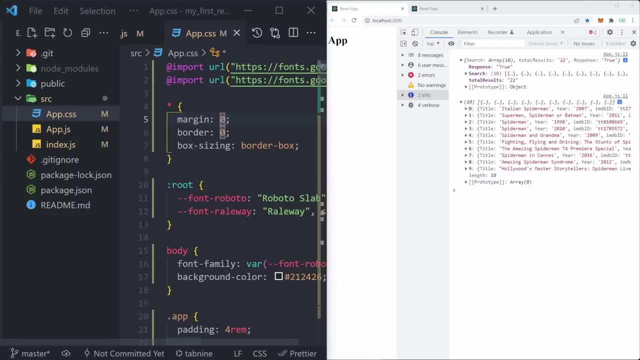 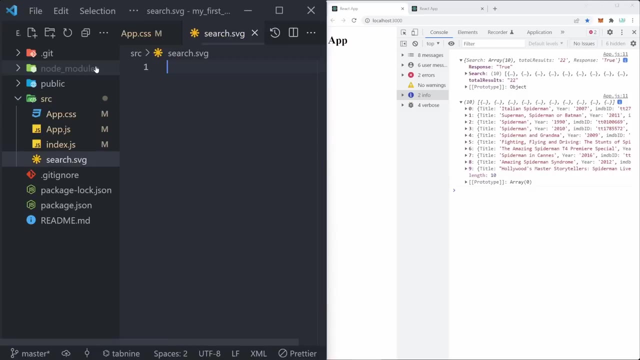 as well as appjs. You can simply copy the appcss and paste it right here. This is going to contain the styling for our project. There's also going to be a searchsvg, So let's create a searchsvg And let's simply paste what you copied. 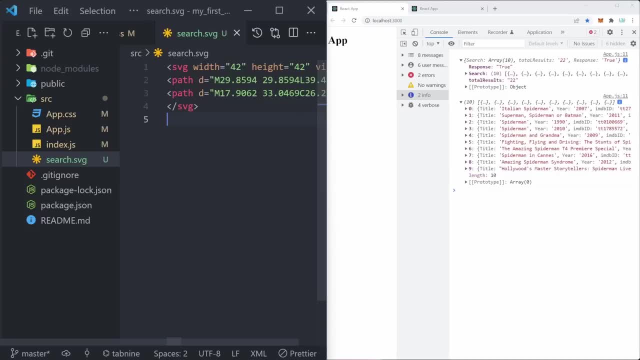 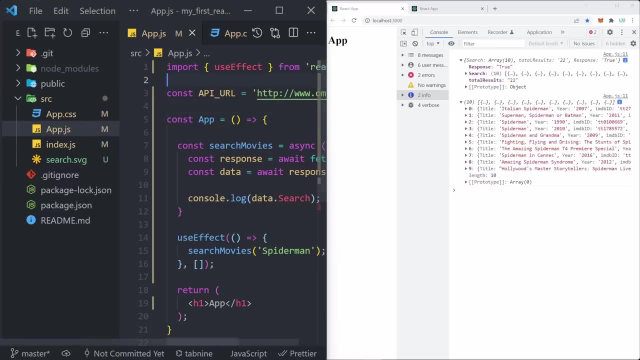 from the GitHub gist down below. This is just going to be a search icon. Now that we have the styles, we of course have to import them as well as import the search icon. We can do that by saying import in a string: slash, appcss. 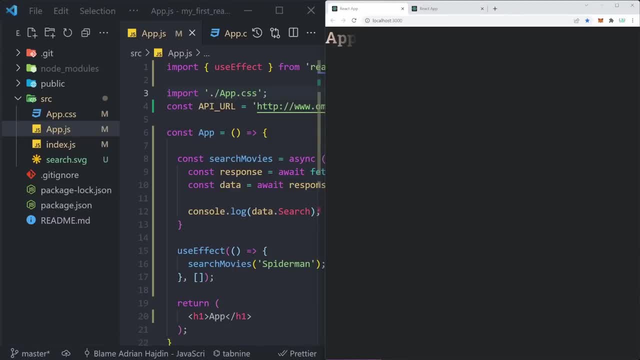 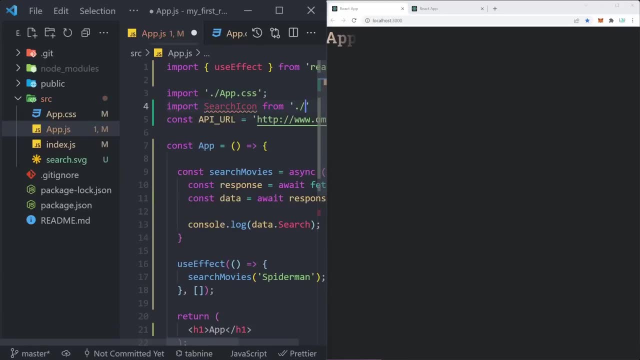 As soon as we do that, you're going to notice that the styles are immediately applied. And while we're here, let's also import the searchsvg. We're going to use the search icon from slash, searchsvg. Great, We're going to use this later on. 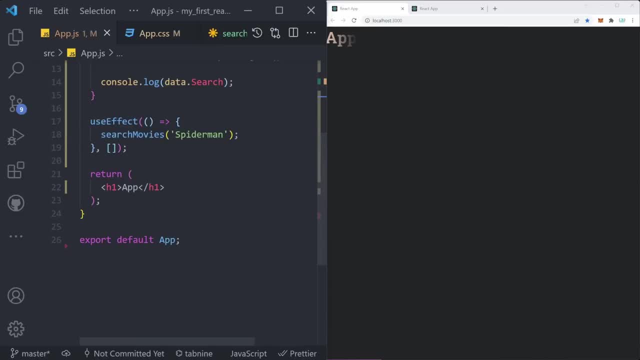 Now we are ready to start creating the JSX of our application. So let's start with a div. We're going to wrap everything inside of a div, And that div is going to have a class name equal to app. Inside of there, we're going to have an element. 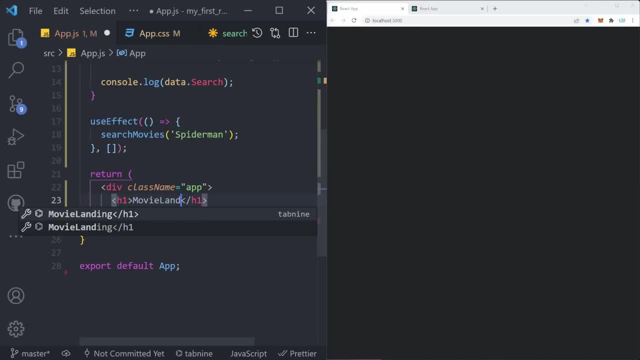 that's going to be the name of our class And that div is going to be the name of our application. Let's call it movieland, And it gets positioned nicely in the middle. This is like writing HTML, but you're going to notice the power of React. 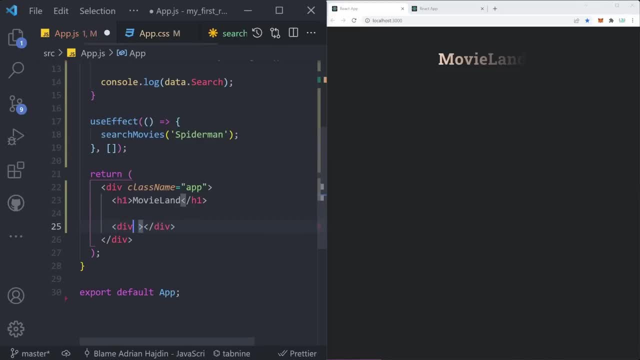 as soon as we start making it dynamic Below that we can create a div that's going to have a class name. Keep in mind: this is class name, not just class as it is in HTML, And that's going to be equal to search. 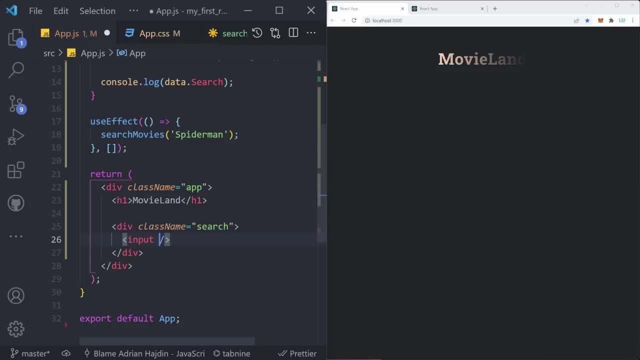 Inside of this div, we're going to have an input field. An input is a self-closing tag that has to have a few properties. First of all, it has to have a placeholder which is going to be equal to search for movies. 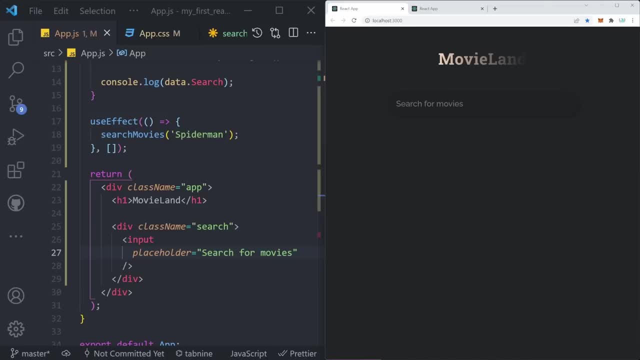 If we save that, you're going to notice this nice input appear right here. An input in React needs to have another two things which are crucial. The first thing is going to be value, For now let's set it as a static string of Superman. 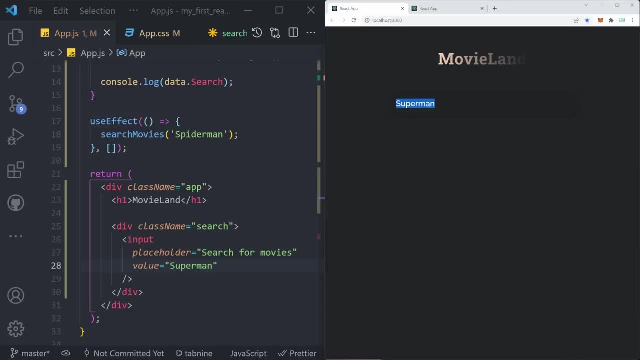 As soon as we save that, you're going to notice that this input immediately has the value of Superman. But now, if you try typing something, you won't be able to because the value is statically set. So how do we change it? 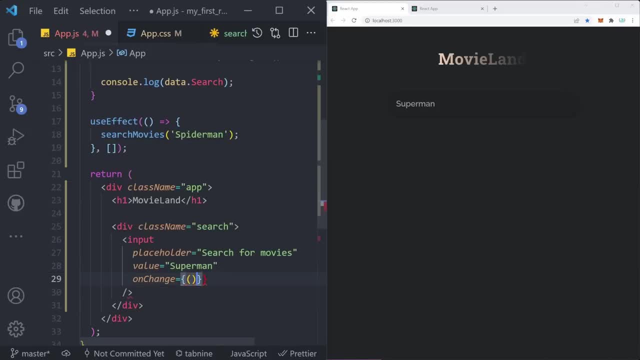 For that we have to have an onChange which accepts a callback function that looks like this: For now, let's leave it empty. We're just going to make it static for now and then later on, once we implement the state, we're going to make this actually changeable. 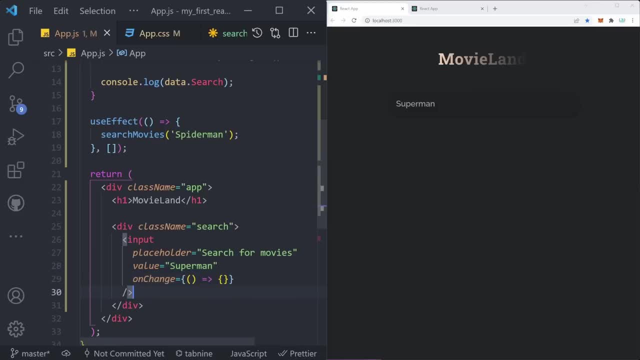 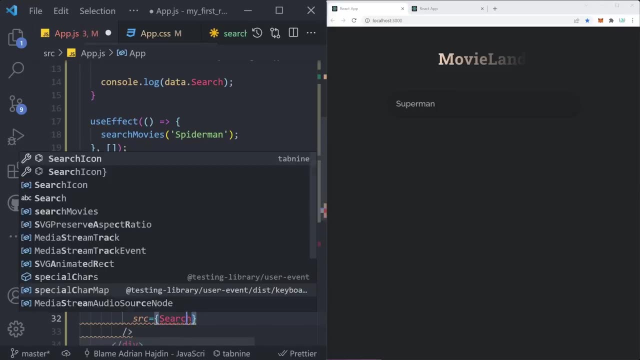 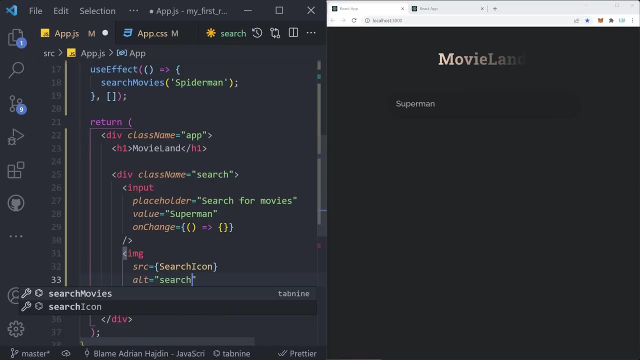 and that's going to recall our API. Below our input, we're going to have a self-closing image tag and the source is going to be search icon. Of course, every image tag also needs to have an alternative tag, which is useful for screen readers. 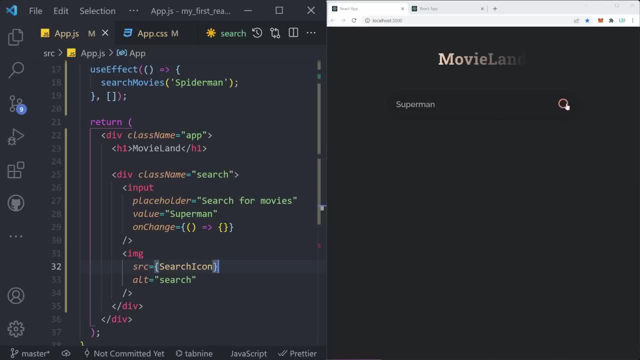 So we can say: search and save it. And there we go. Now we have this magnifying glass icon. Our magnifying glass icon is also going to serve a purpose of a button, So we can add an onClick property right here and also add an empty callback function. 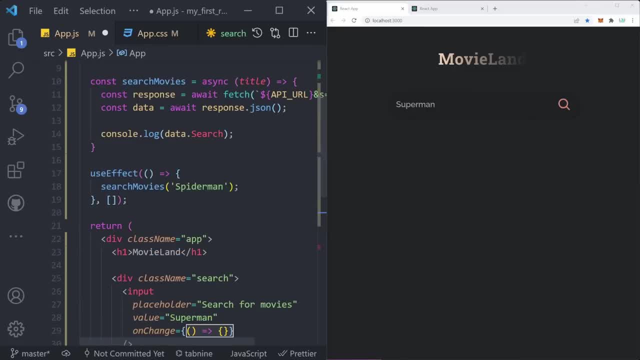 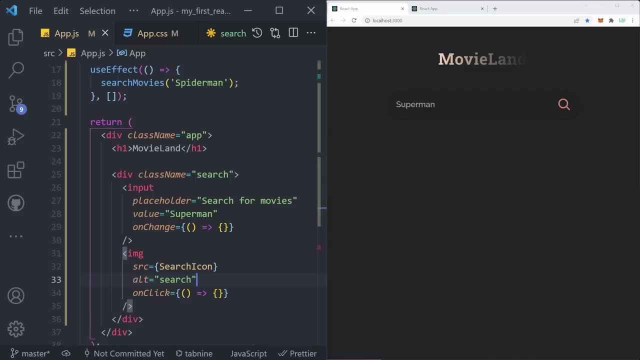 because later on we're going to be calling our above API straight from here, But for now we're just building the JSX, so we don't care about that for now. Now we can go below this search div and create a new div. 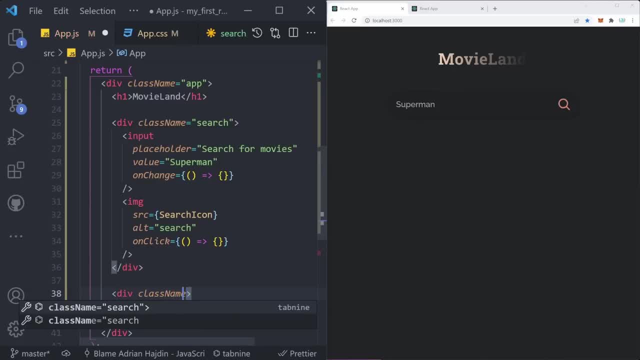 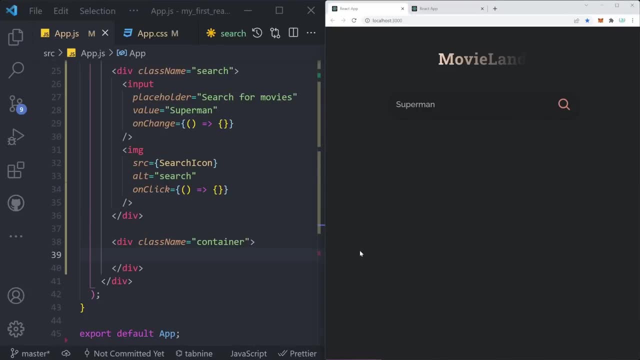 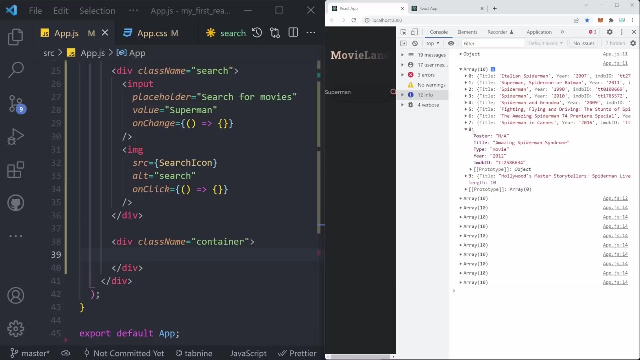 This div is going to have a class name equal to container. So what we can do right now to test this out is go to inspect, go to console array. Let's take one of these Spider-Man movies and let's copy the entire object. 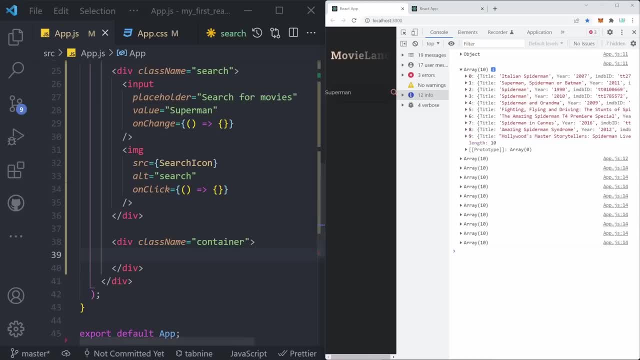 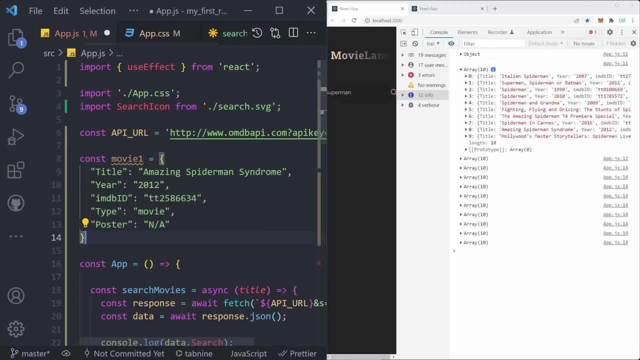 by right clicking and clicking copy object We can go to the top and say const movie1 is equal to, and then we can paste that Right here. we're going to get the data for that specific movie. We're going to use this as static data. 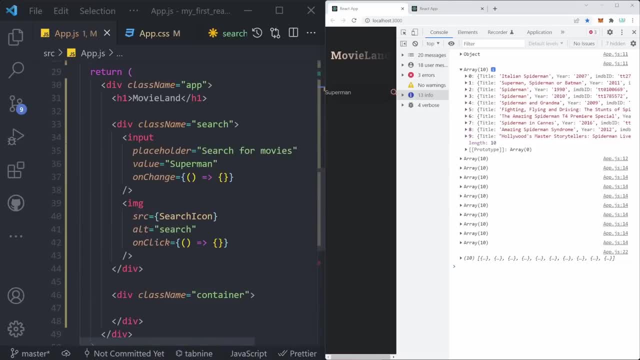 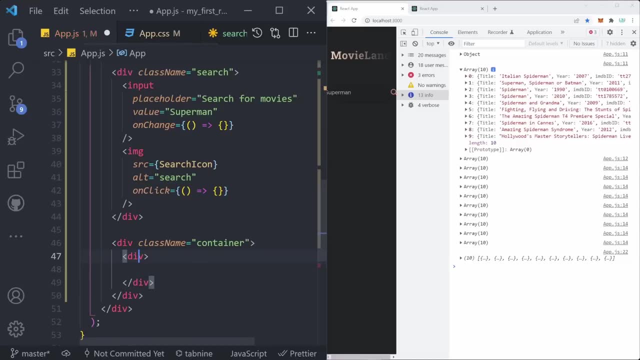 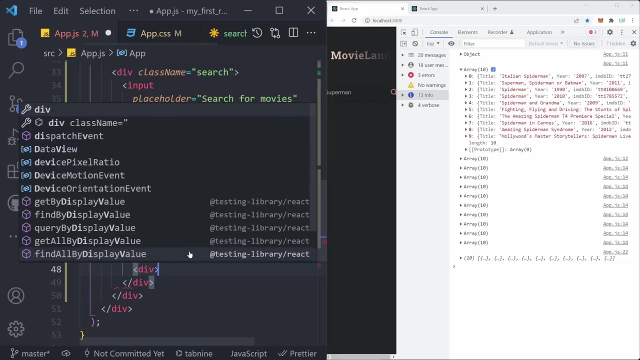 just to render out something so that we know what JSX are we writing. So, inside of this container, what we can do is create a div that's going to have a class name equal to movie. Inside of there, we're going to also render a div. 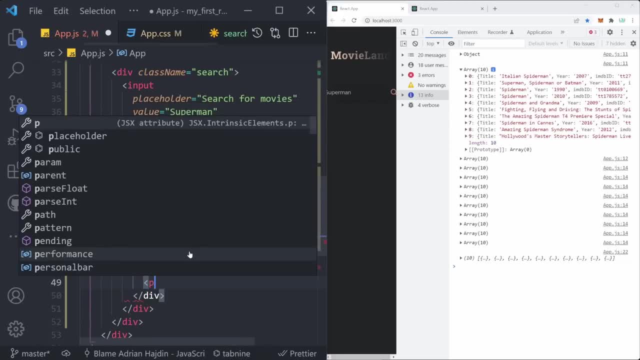 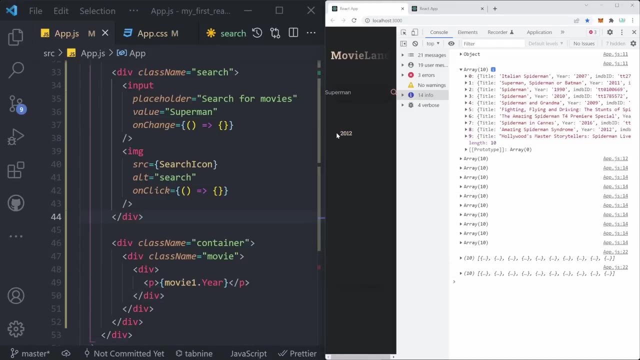 and inside of that div we're going to render a paragraph. There we want to show the year of the movie, So what we can do is say movie1.year. Now if we save that, you can notice we got 2012 right here. 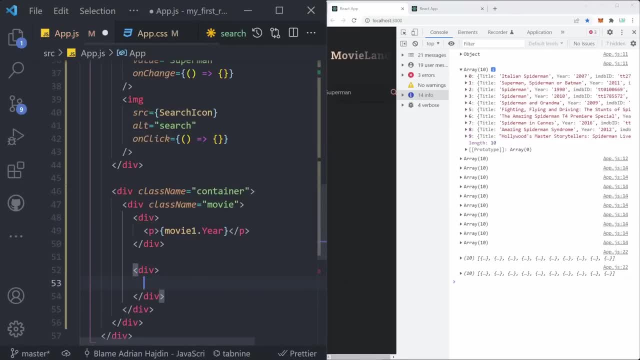 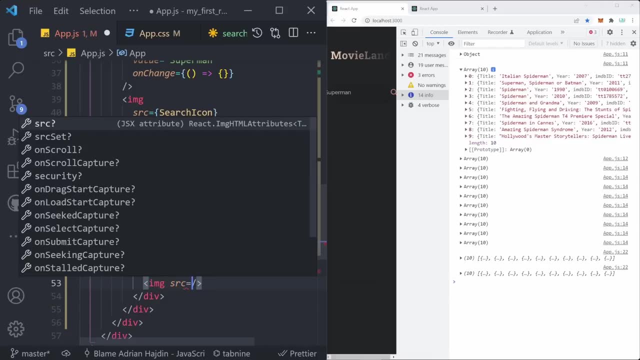 Below this div, we're going to create one more div, and this is going to be the div that's going to contain our image. Our image is going to have the src or source property equal to movie1.year. That's going to be poster. 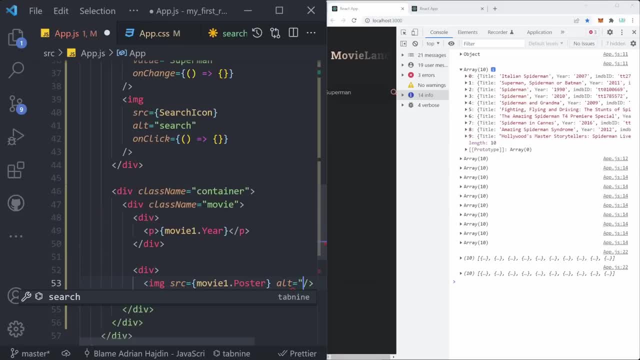 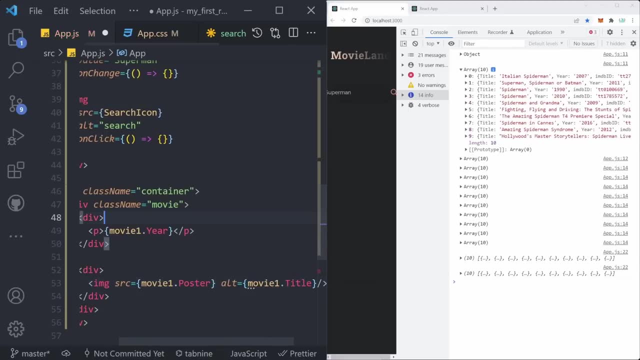 not poser. that's going to be poster and an alternative tag which is going to be equal to movie1.. And that's going to be title. Now, let's save this, and it looks like we cannot see the image for this movie, which is great. 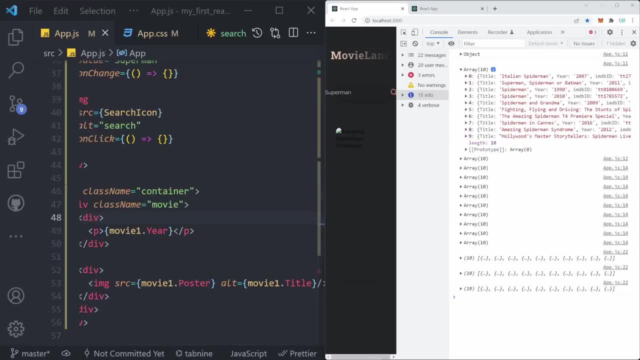 because it allows us to add an extra check to make sure that there is an image. So what we can do is say: if poster is not equal to na- this is how this API declares movies that have no image- then we can render a movieposter right. 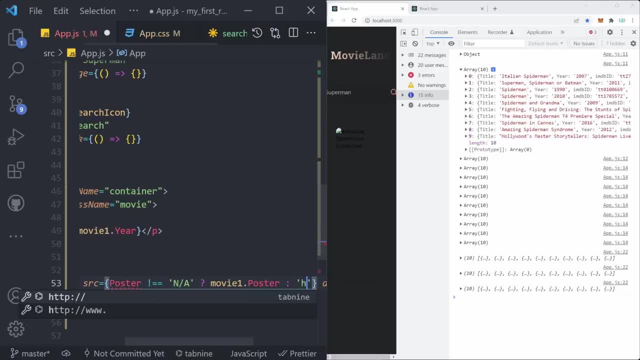 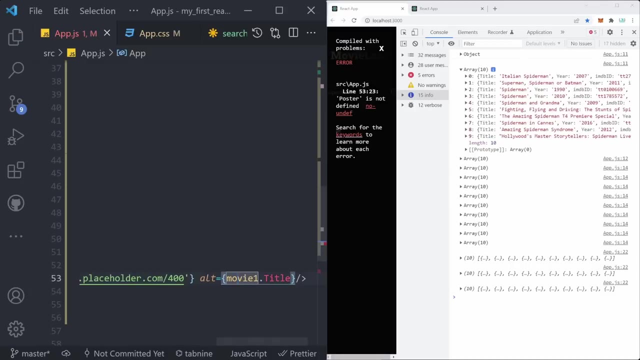 But if there is no image, then we can render: https//viaplaceholdercom/.400.. This is a placeholder image and we get a nice error from React saying that poster is not defined. So this is going to be movie1.poster. And there we go. 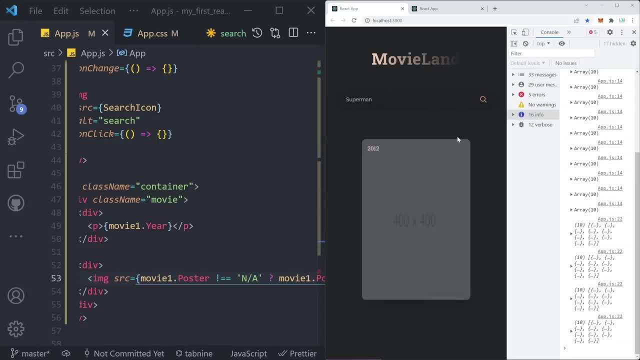 We have a 400x400 placeholder image. We're going to provide this placeholder image if the API doesn't provide us with a real movie image. With that said, the most important thing that we can add below this div is going to be another div. 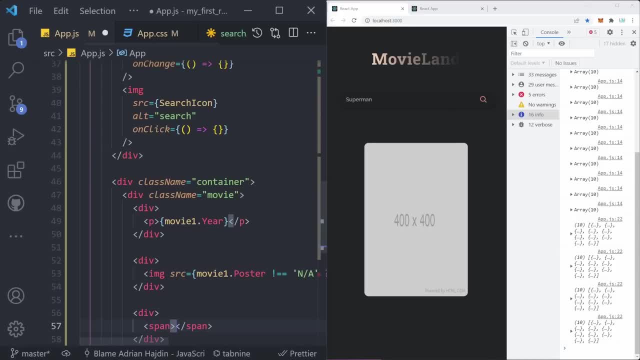 that's going to have a span element inside of it and there we can render movie1.type. If we save that, you're going to notice that the type of this movie is a movie. It can also be a TV show Below that span. 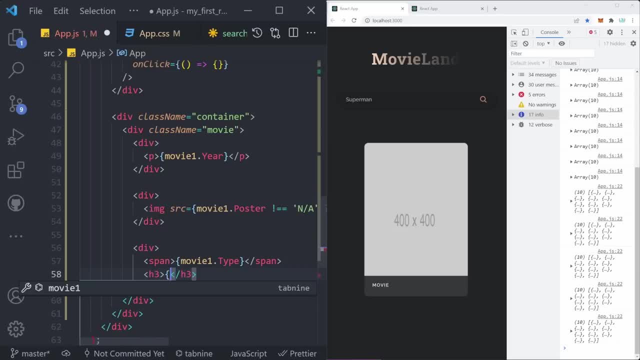 we can render our last element, which is going to be an h3. that's simply going to render the movie1.title with a capital T. If we save that, we're going to notice Amazing Spider-Man Syndrome Movie 2012.. Now we have the look of our single movie. 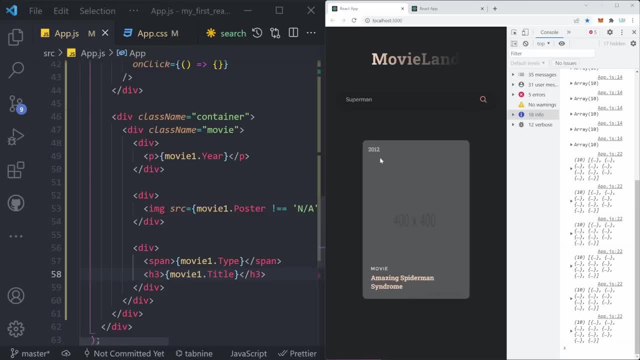 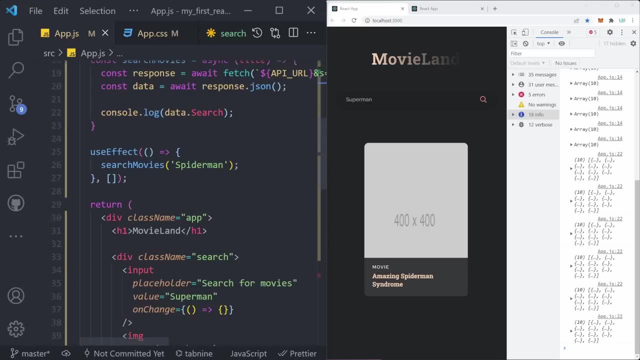 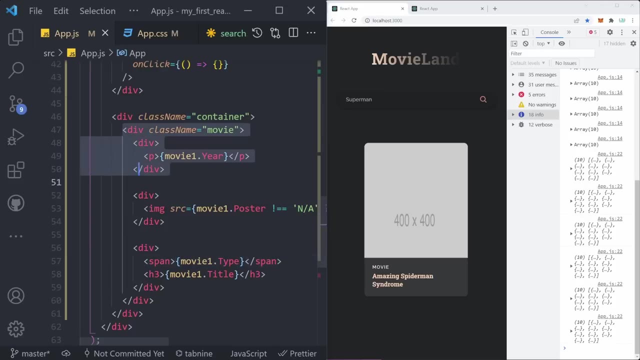 But this is not that good because it's just one and, more importantly, the data for that movie is static. So how can we fetch the data for all the movies and then display them here? The first step in doing that would be extracting the code for this movie. 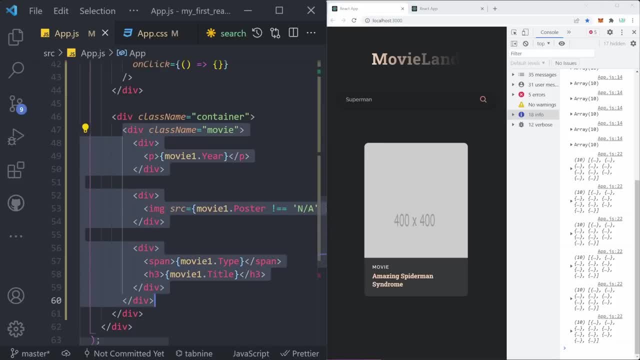 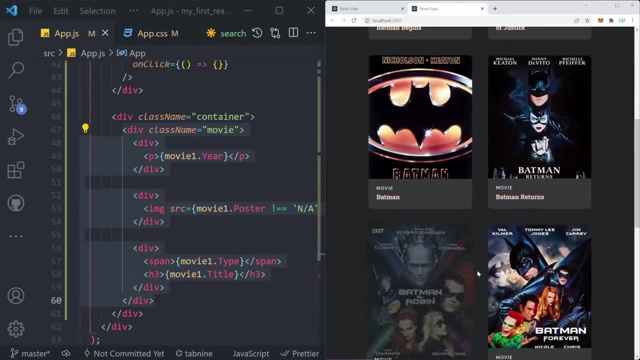 into its own custom component. And the reason we're doing that is because, if you think about it, we're going to have many of these cards. They're going to be repeated quite often. So instead of doing something like this, where we would have to have hundreds of lines, 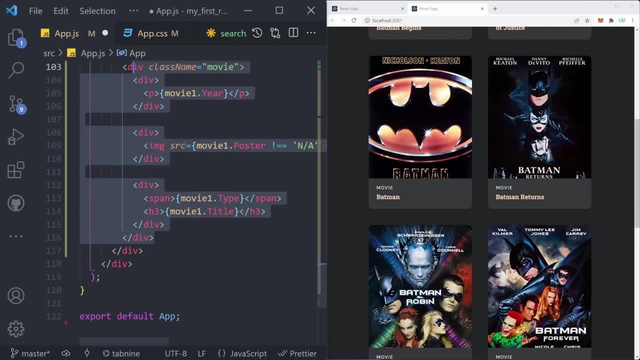 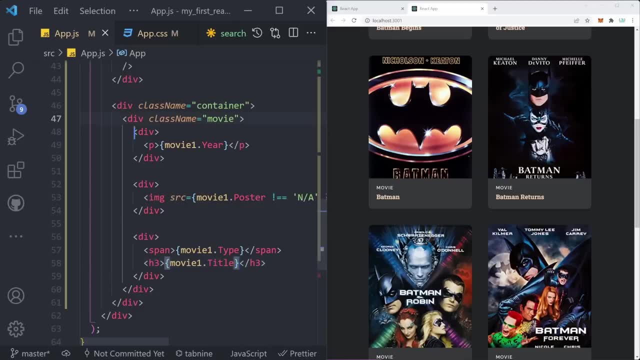 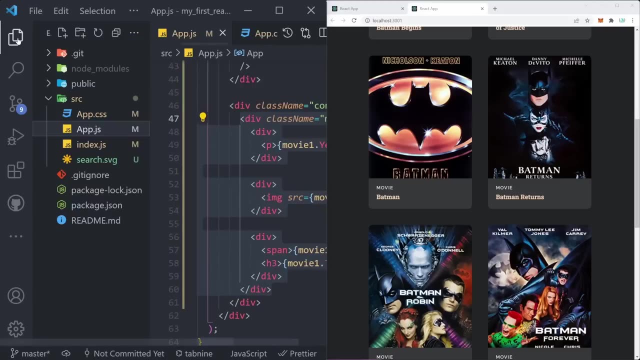 to show just a few movies. what we can do is just create a custom component, and that way we'll be able to do it almost in a single line. So let's copy this entire div with a class name of movie, Then go to our file explorer. 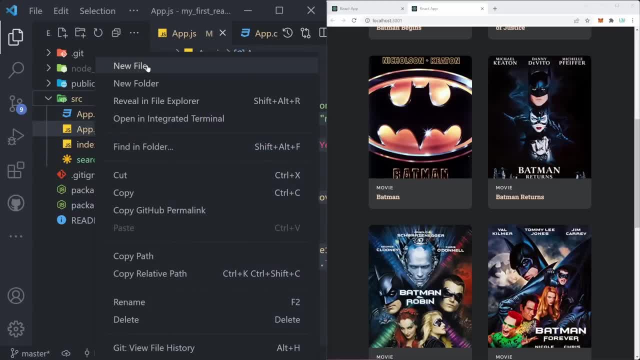 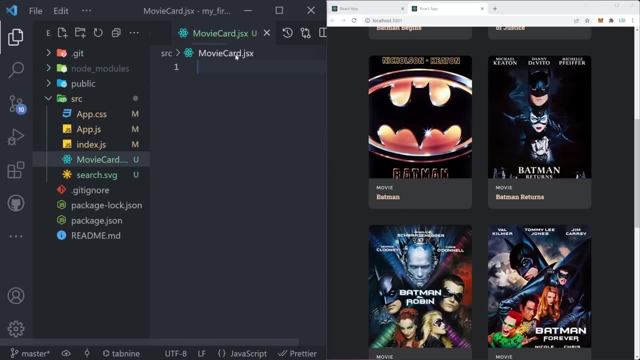 and create a new file inside of the source folder called movie-cardjsx. Now you might be wondering why did I add a jsx extension to this file In React? whenever you create a new React component, jsx extension is preferable. It adds this React logo on the left side. 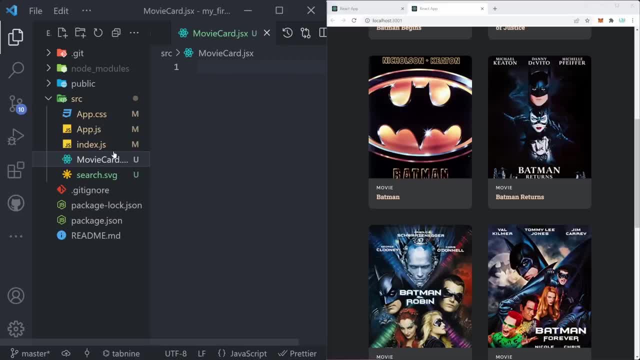 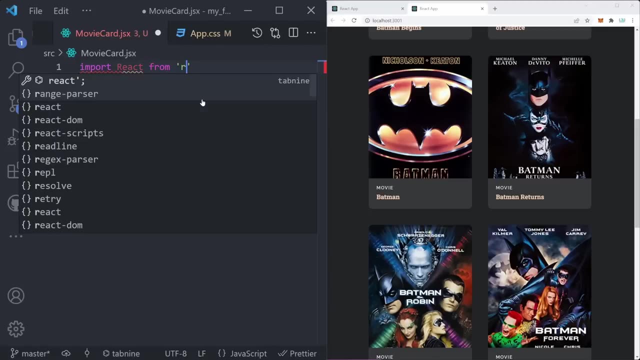 and that's basically it. There isn't any difference between a js file and a jsx file. I usually add a jsx file for any component that I create in React, And it's going to be the same. It's going to be import React from React. 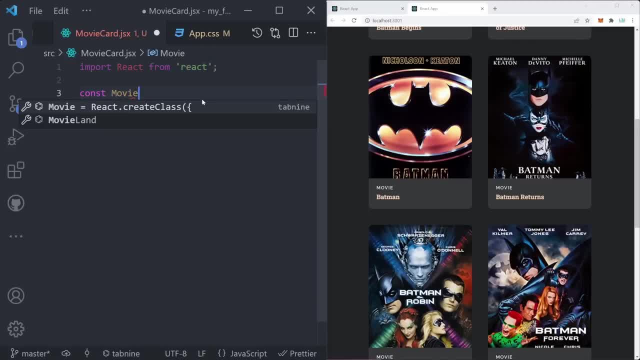 Then we're going to create a component const. movie-card is equal to a functional component. Notice how the file name and the component name are the same. This is not a necessity, but it's definitely a good practice. Then we can render the return. 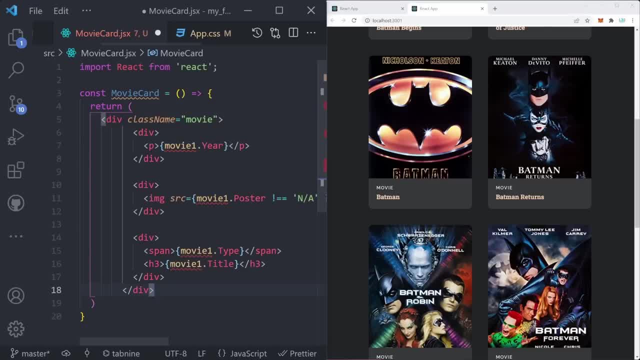 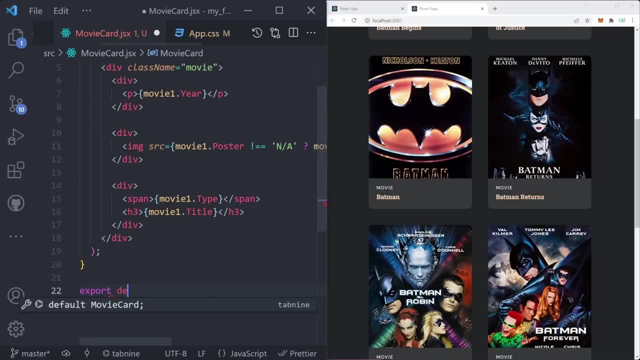 Right here, And then inside of the return we can paste what we copied. We can also hold control and alt and then press arrow down a few times, And then we can invent this properly. There we go. Now we can export default movie-card. 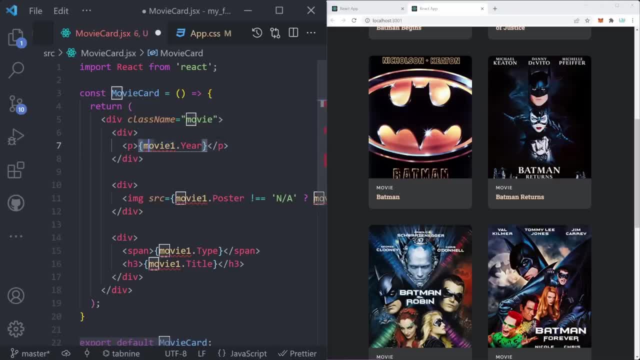 And we can also notice that right now we don't have access to this movie1.something, So we're going to potentially pass that over through props. You already know the drill. We're getting access to the props right here, But just so that we don't have to repeat ourselves. 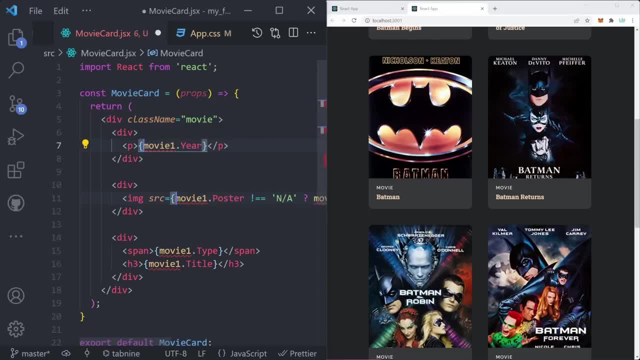 propssomethingeverytime. what we can do is destructure the props, Use object destructuring, So that means simply put a pair of curly braces here and then get something that you passed inside of those props. So now we have our movie component. 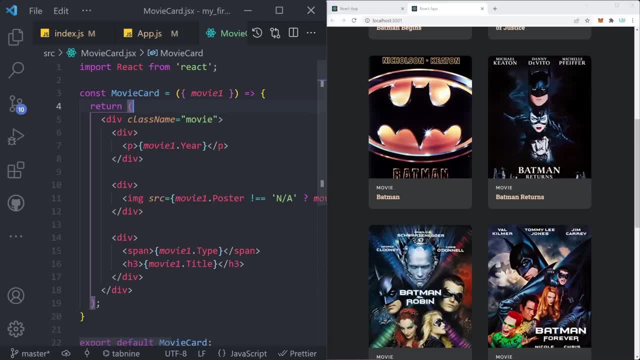 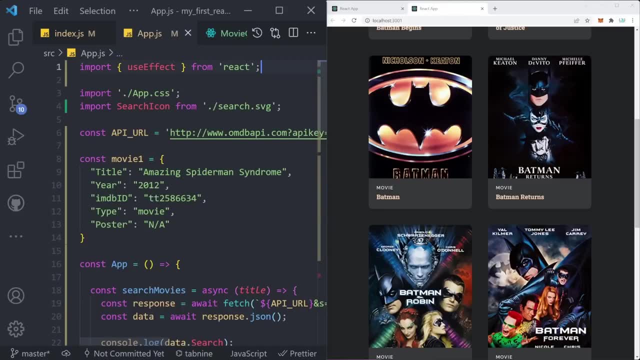 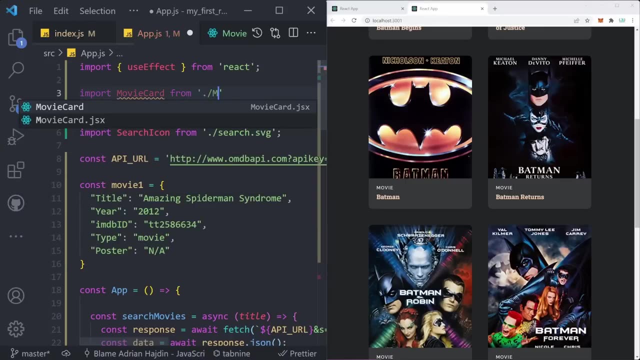 the same as we had our props, And we can also import the person component before, but it's in a separate file. So inside of the appjs we can now import, at the top, import movie-card from slash movie-card. And now, as we learned, 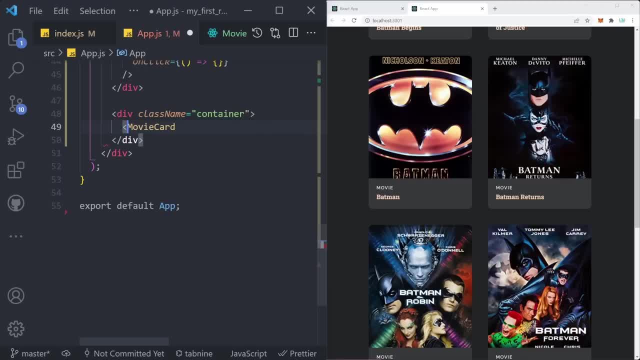 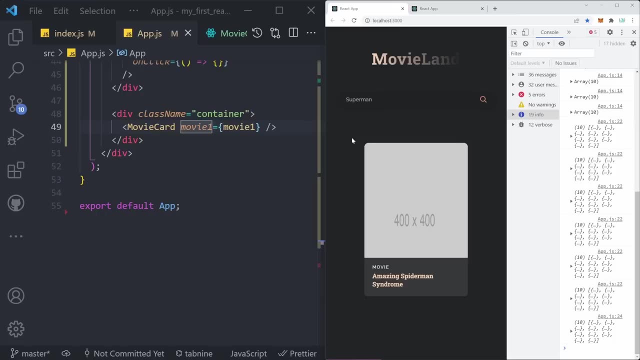 instead of this entire div, we can simply call a movie-card and call it as a self-closing component. Of course we also have to pass in a prop called movie1 is equal to movie1.. And if we do that and go back to our application, 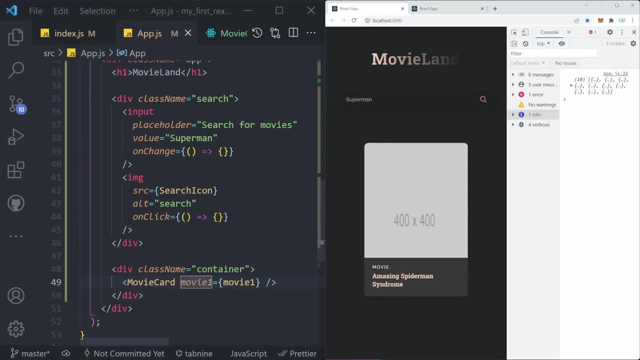 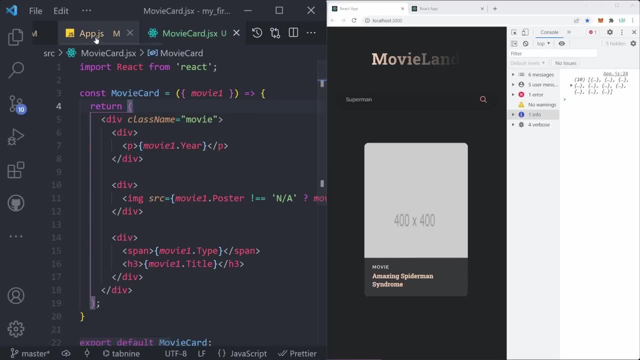 you can see that we have the same thing we've had before: just a single movie-card. But what we've done right now is going to make our life so much easier later on, once we want to map over all of our movies- The first step in doing that. 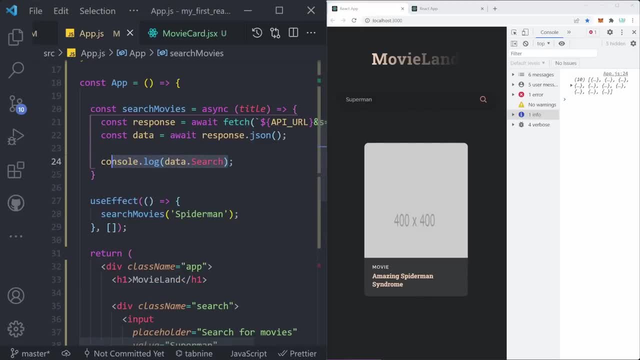 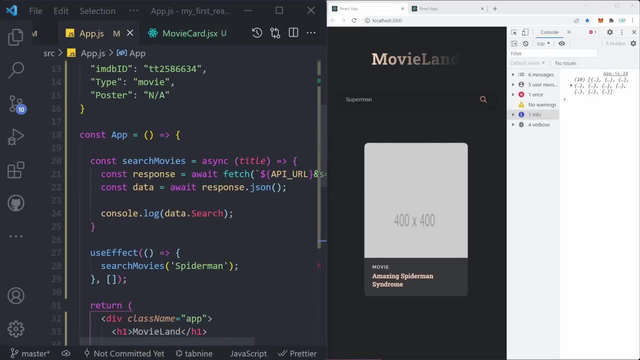 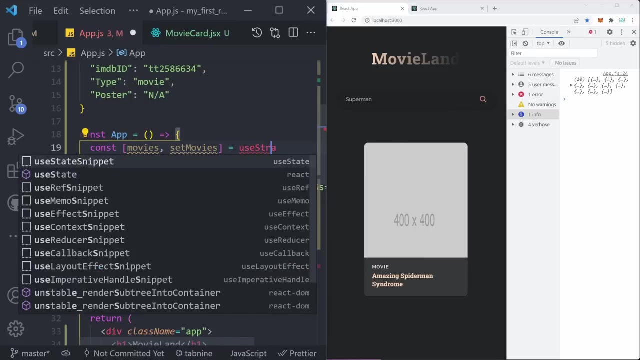 is getting our movies from right here, from our console log, all the way to here where we can actually map over them. So what we can do is create a new state. We can say const movies and set movies is equal to, that's going to be equal to the call of the useState hook. 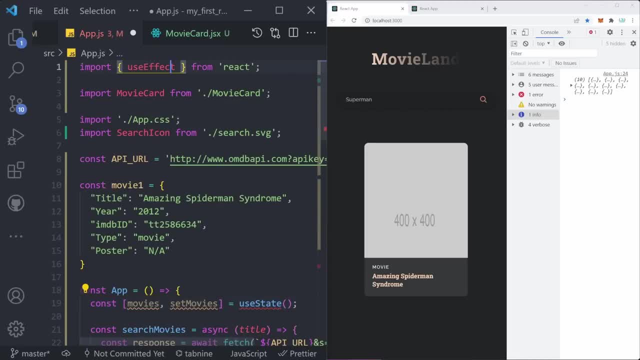 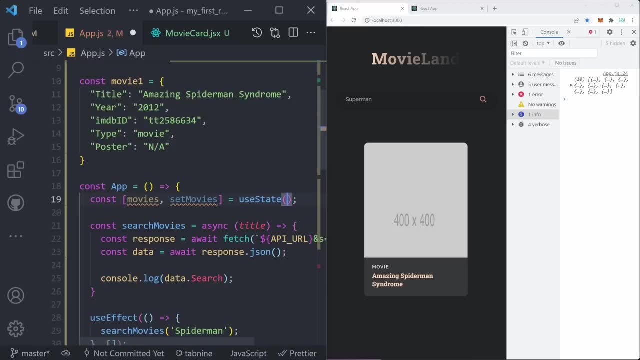 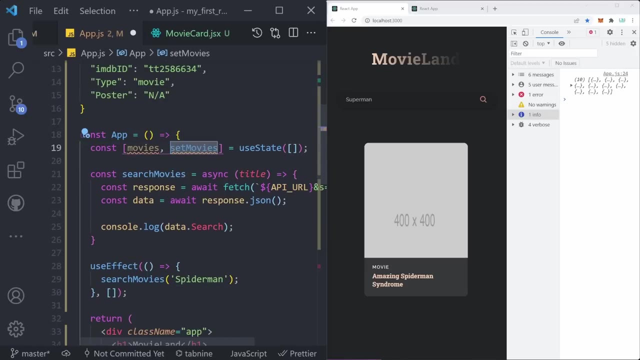 Of course, we have to import it at the top. That's going to be useState, Next to useEffect, And we can set the default value of our movies, which is going to be an empty array. This is going to give us access to the setMovies setter function. 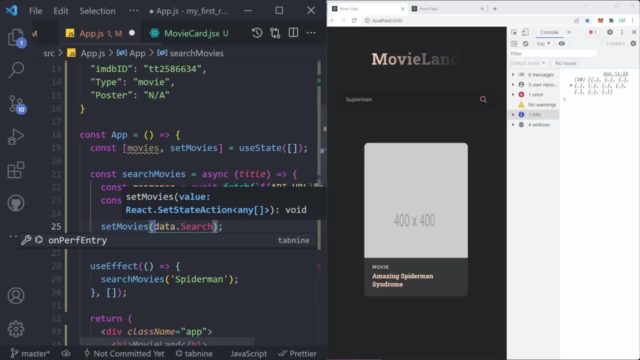 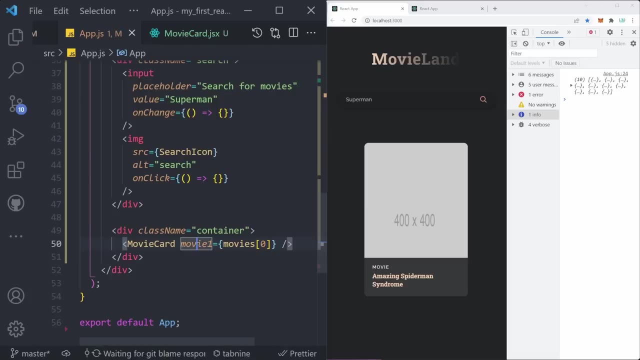 And instead of console logging it, now we can pass the datasearch into our setMovies. Of course, that gives us access to our movies. So now we can dynamically pass movies and then zero into our movies, And this is going to allow us to populate the movies. 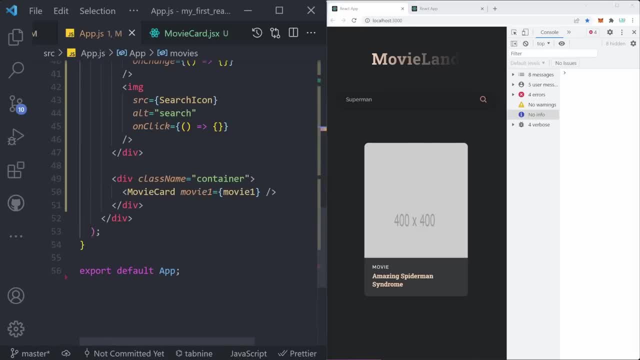 So what we can do right now is, at the bottom right here, open a dynamic block of code using parentheses and check if movies question mark dot length is greater than zero. If that is the case, then we want to render our movie card. So let's take this movie card. 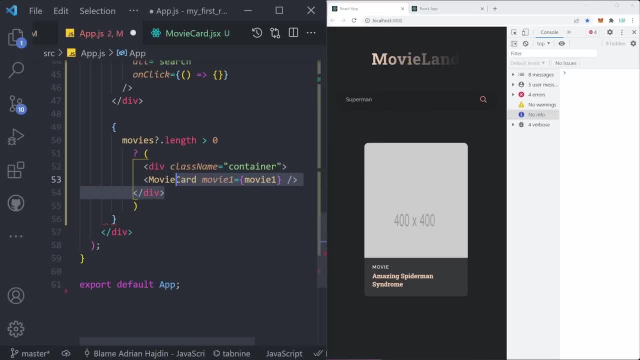 and put it right here. Let's indent this properly, And then else, if that is not the case, so if there are no movies, then we want to render something else And that something is going to be a div. So we can say div right here. 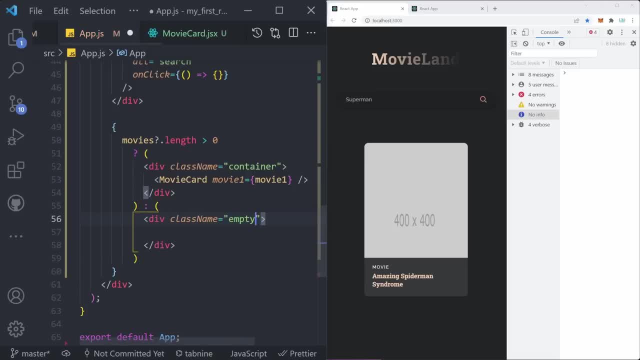 Give it a class name equal to empty And then create an h2 element inside of there. that's going to say no movies found And we can save that And nothing's changed. That's because we actually have movies in our array. We would only see this if the movie array was empty. 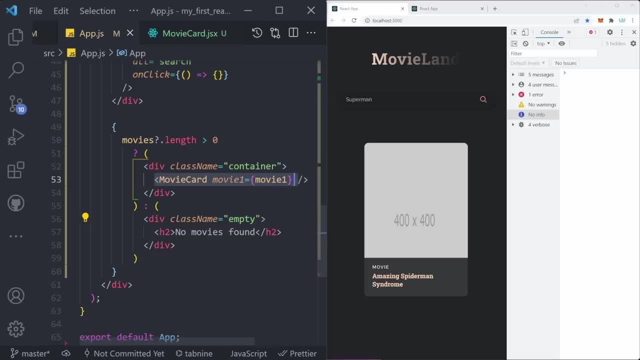 So, considering we do have the movies, why are we still seeing this one static card? Let's fix that immediately. What we can do is, instead of showing this one single card, we can open a dynamic block of code and then map over movies by saying moviesmap. 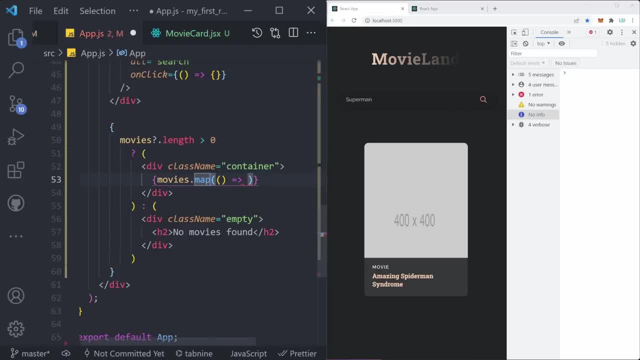 and then we can map over them. We're usually mapping over arrays which are plural, And then inside of there we're going to get a singular movie for each iteration of the map. So what do we want to render for each iteration of the map? 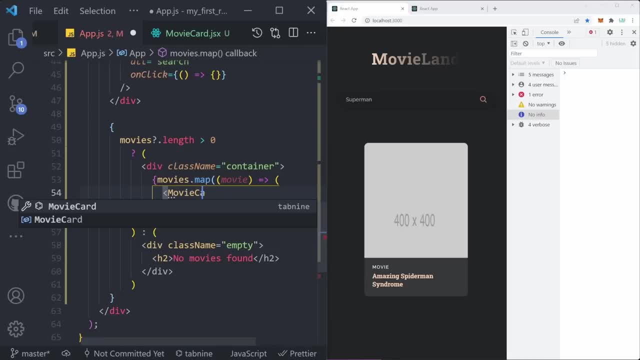 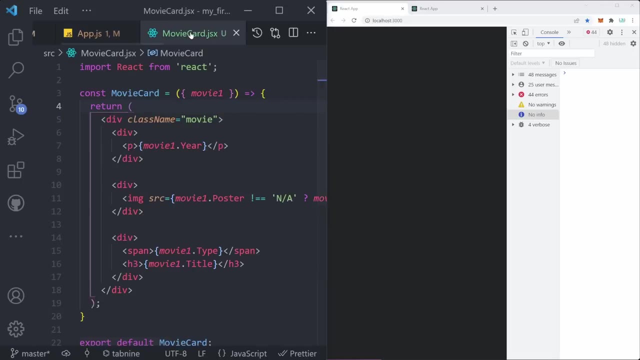 That is going to be a movie card component. If we save that, we're going to get an error because we're not passing the movie prop. So let's pass a movie prop equal to movie. Now this is going to dynamically change, But of course we have to go right here. 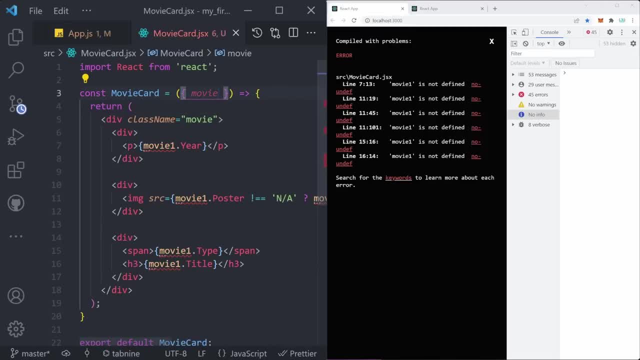 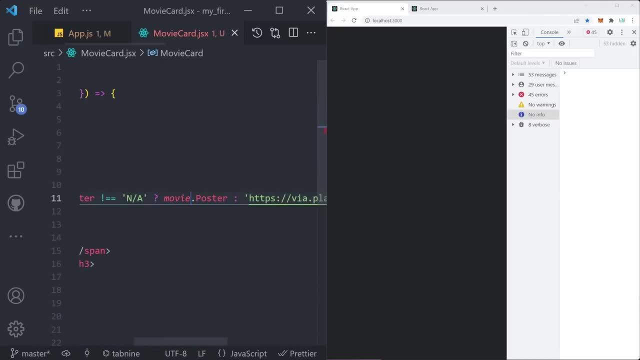 and we have to change this into movie. Of course, we have to change it in every single other place as well. The movie one was just a placeholder. There we go. We also have to change it here as well, And with that. 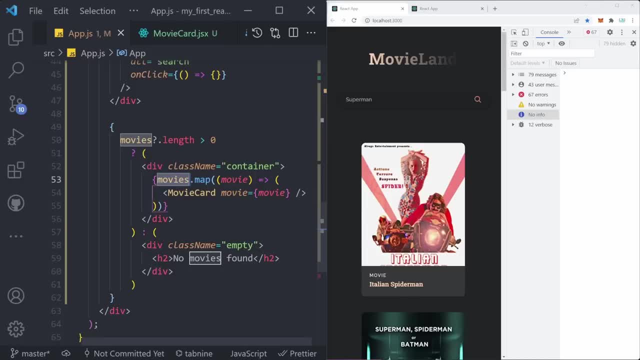 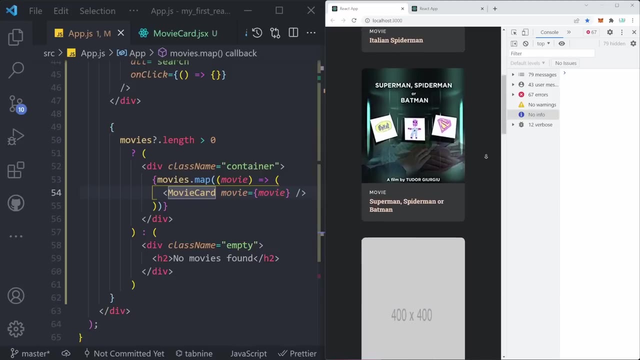 we're dynamically looping over our movies array, which is fetched from an API. We're taking each individual movie and we're dynamically passing it as a prop to our movie card And that's going to result in the render of all of our movies. Some of these movies don't have an image. 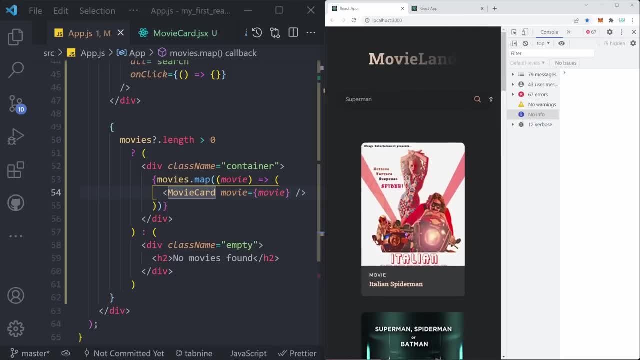 but don't worry about that at all. That is API's fault. Now we can kind of tidy this up a bit by putting this right here. putting this here as well. We can fix the indentation if we go ahead and move everything one step to the left. 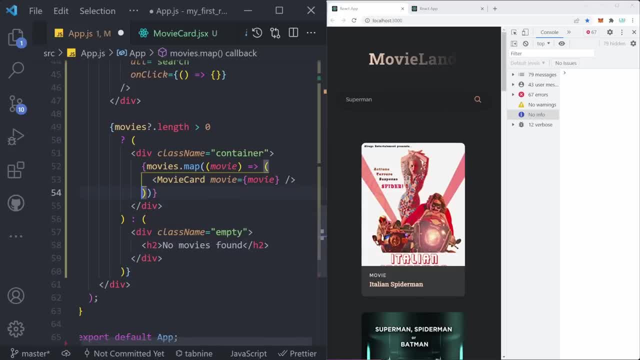 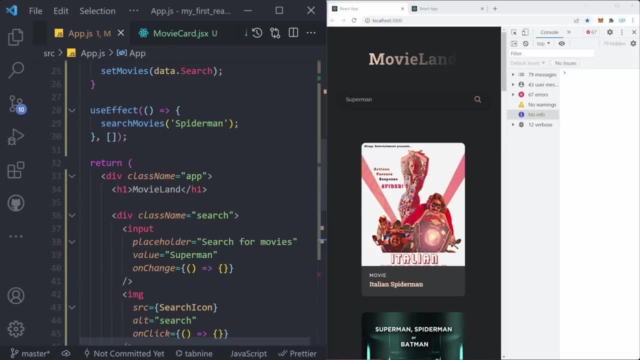 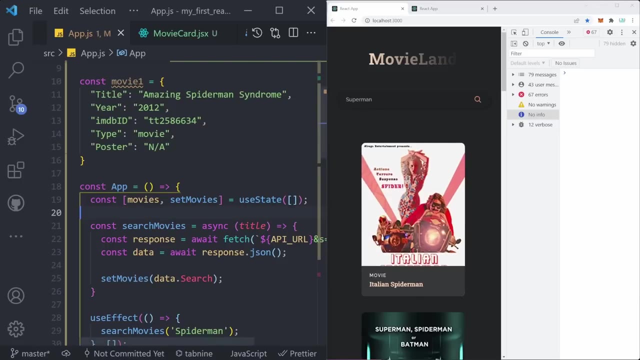 There we go, And this is already looking much better. Our next step is making the search functionality work, And for that we're going to need another state, So this might be also something new to you. You can have multiple states and even multiple use effect hooks. 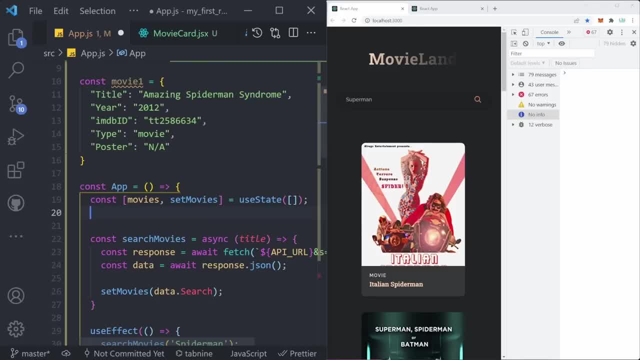 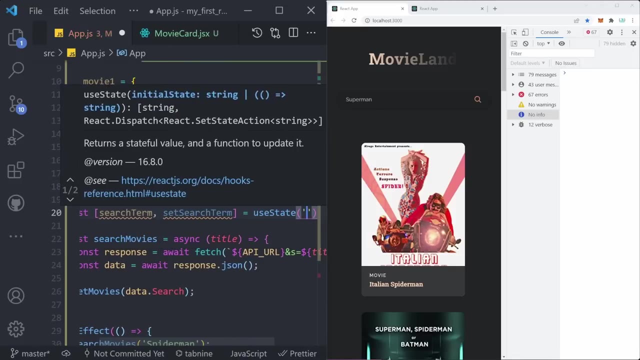 per one component. There is no limit. So right here let's say const searchTerm as well as the setSearchTerm is equal to- you already know- the drill useState, and then we're going to pass in an empty string because our searchTerm at the start is going to be empty. 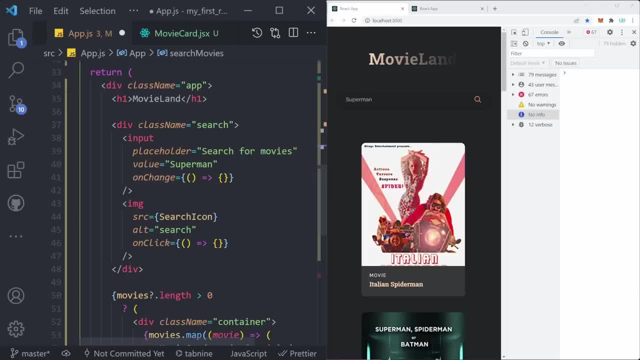 What we can do, then, is, inside of our input, dynamically change our searchTerm. So our value is not going to be static anymore. We're going to use curly braces and we're going to change that to searchTerm. So now it's dynamic, As you can see. 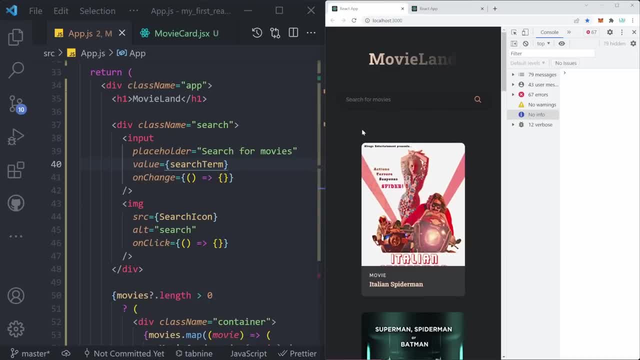 it's empty at the start, so we can only see a placeholder To be able to change it. we need to do a similar thing we've done before with the click event when we changed out counter. So we need to set the searchTerm and then we call it. 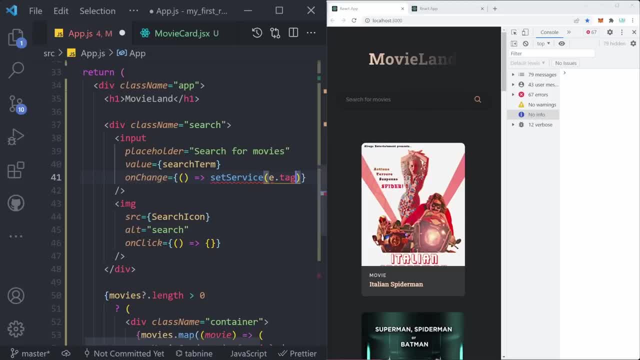 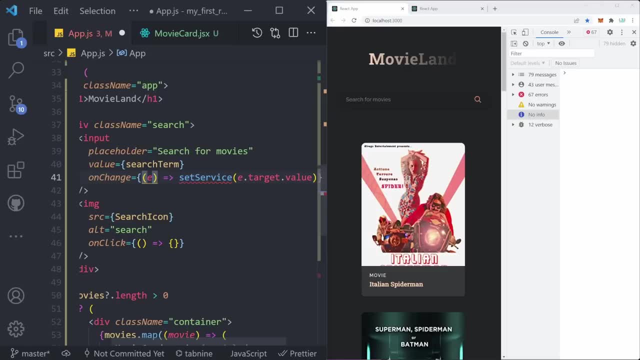 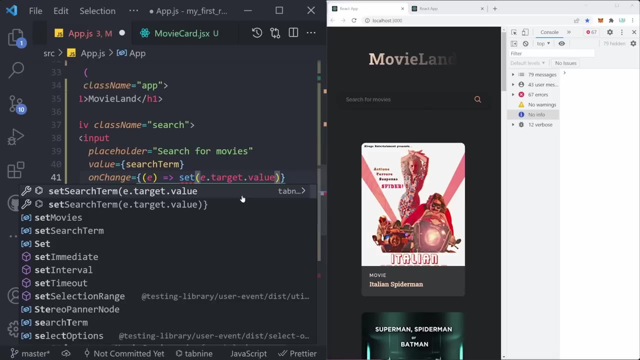 and pass in the etargetvalue, and that e we're talking about is coming from the callback function right here. That is the event Right here. not sure why I have setService- that was supposed to be setSearchTerm. That's much better. 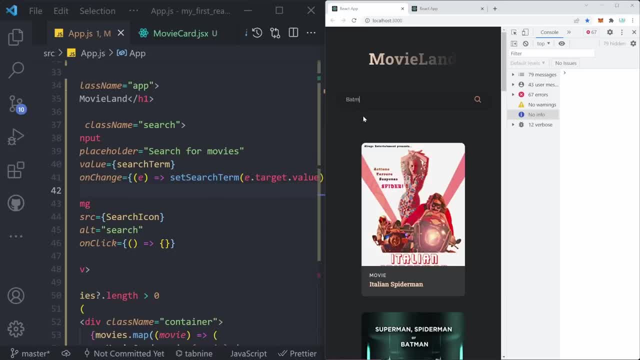 And now we can actually type into here. So if I type batman, you will be able to do that. The question is, how can we use that state to dynamically re-render our array of movies? For that we're gonna use this image. 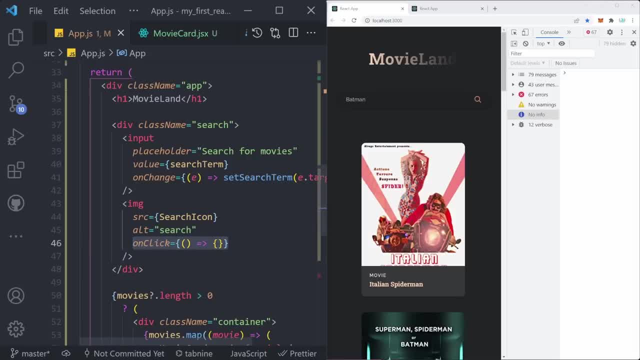 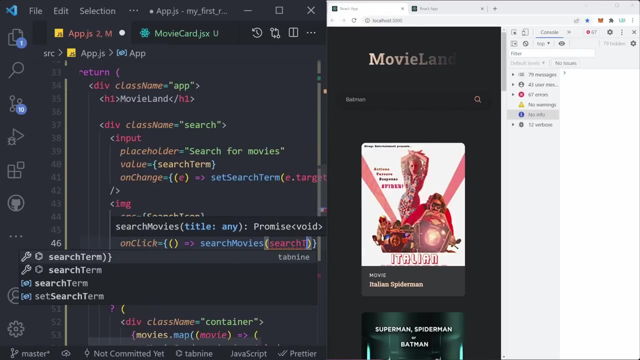 more specifically the onClickListener. We can recall our searchMovies function and pass in a new title. We can do that by calling searchMovies and then we can pass what? Not a specific title, which is static, but rather we can pass in the search term. 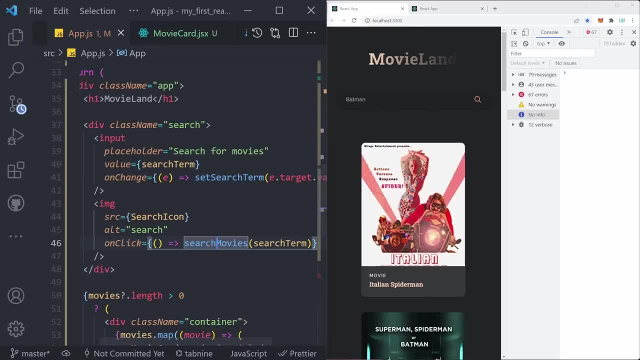 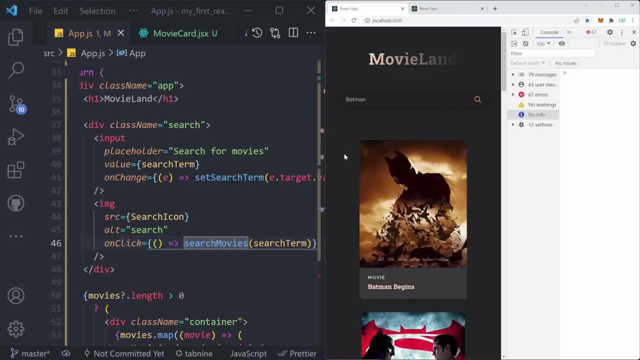 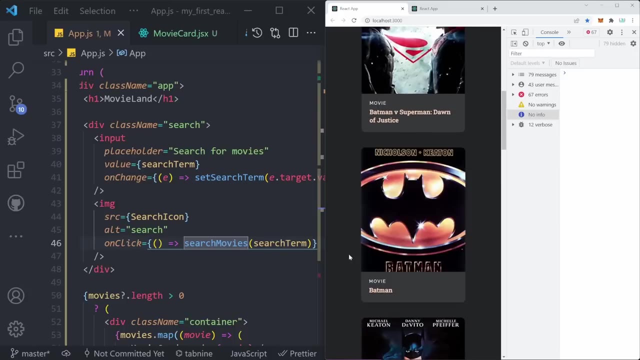 which is dynamic state. So now, every time that we type something in here and click the button, the state is going to dynamically change and that is looking great, You can see. we can hover over it to see the year, also, more details, and we have all of the movies. 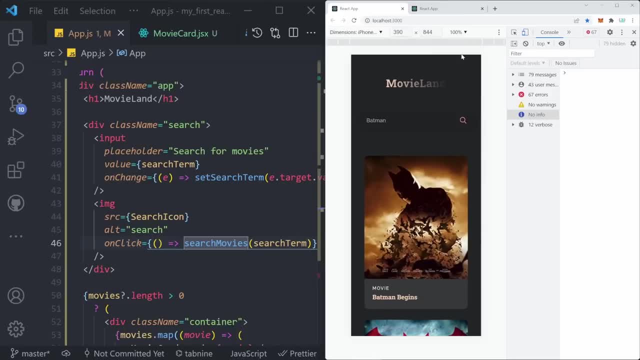 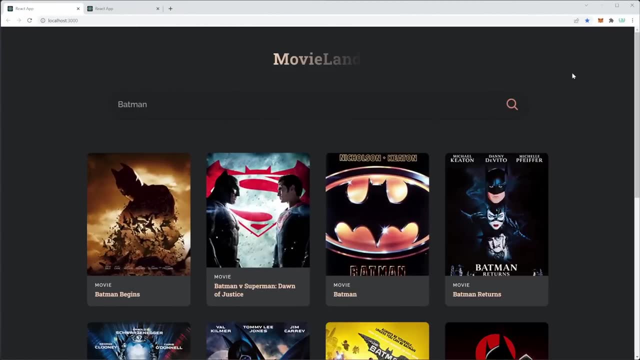 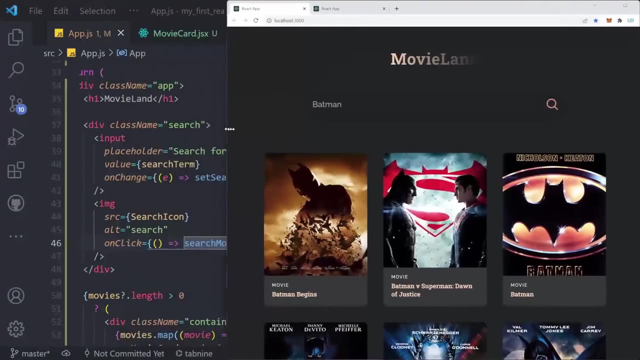 right here. It looks great on mobile devices and it looks great on desktop devices as well. This might be the first React application you've done, Congratulations. I hope that the ease of development of this little app showed you that React is definitely something you want to learn. 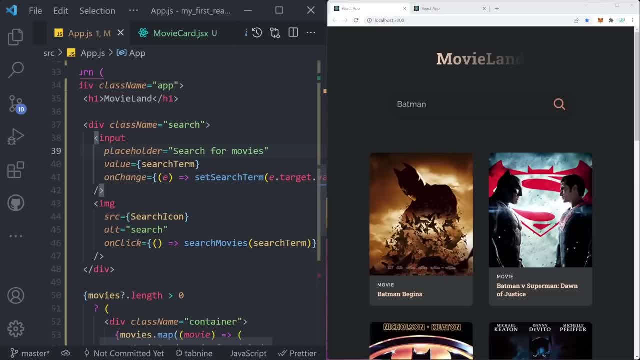 and be an advanced developer in. I've been a React developer for many years now and I can definitely say it's my personal preference. The ease of development and the ability to scale your applications are just amazing when working with React and also the developer workflow. 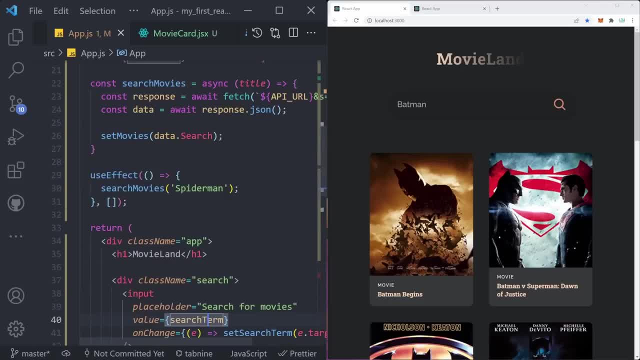 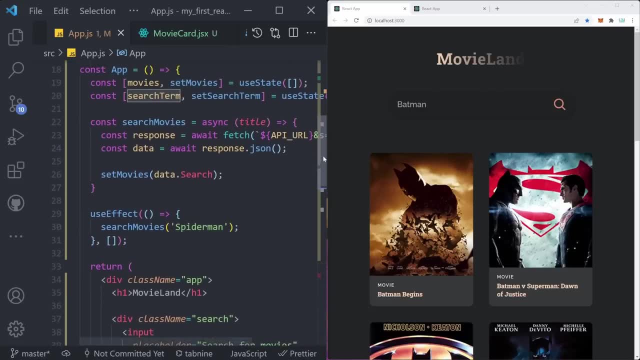 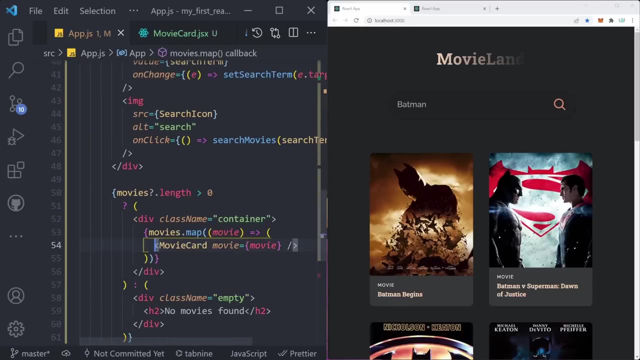 is quite nice. You can code HTML here and you can combine JavaScript immediately with CSS and HTML. We've learned quite a lot. We've learned about state, about use effect, about components, props and much more. I hope you've liked this. 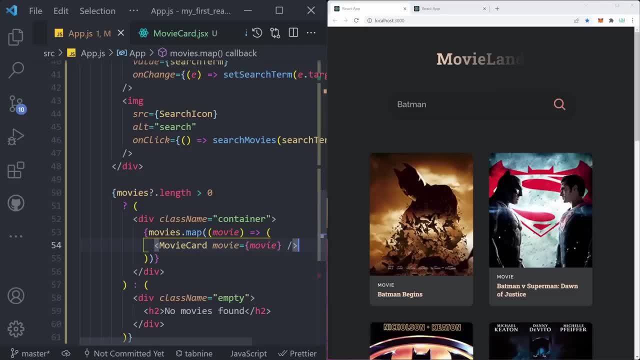 React crash course. This is just the beginning of your journey Here on JavaScript Mastery. we've covered countless more more advanced React projects which I'm sure you're going to love. So just keep learning and soon enough you'll be able to build. 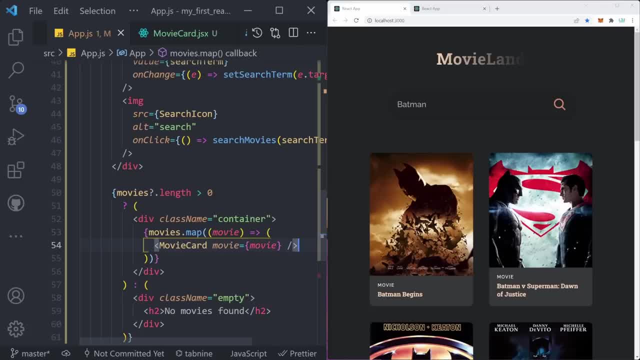 all of these projects. The FilmPyre project is designed to help you learn from bare beginnings to more advanced topics, So stay on the lookout. That is coming soon. If you're not watching this video at the time of the release, it's possible. 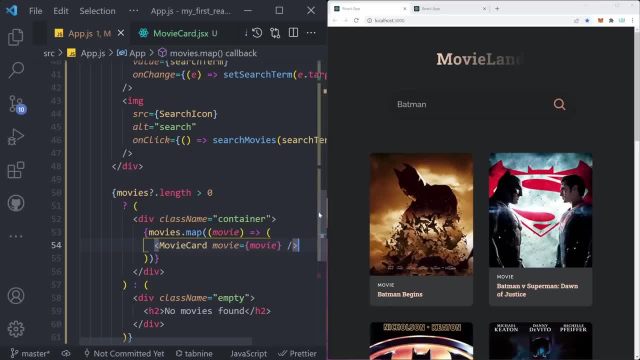 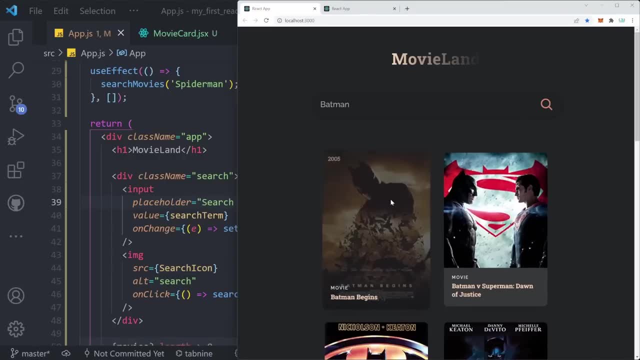 that it's already out, So definitely make sure to check out the description. And that was it for this video. We've learned about state hooks, props and so much more. You've also built this great application and you're ready to dive. 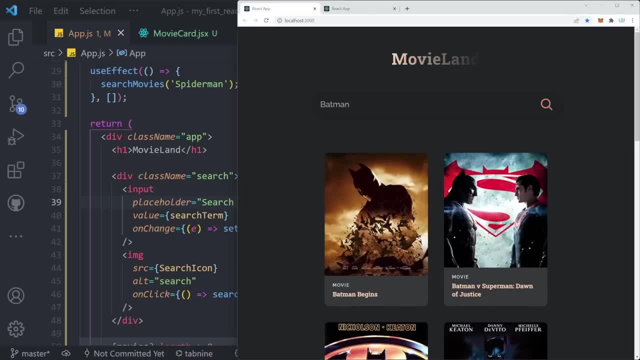 into more advanced React topics. Of course, the entire roadmap of how you can advance in React is down in the description inside of the React guide. Feel free to download it and also let me know your thoughts in the comments. I'm looking forward to hearing your thoughts. 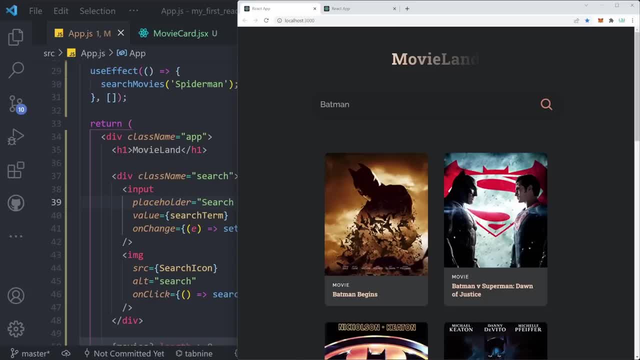 on. what do you want the next video to be? If you have any thoughts, just share them. That's going to be it for this video. I hope you enjoyed it and have a wonderful day.